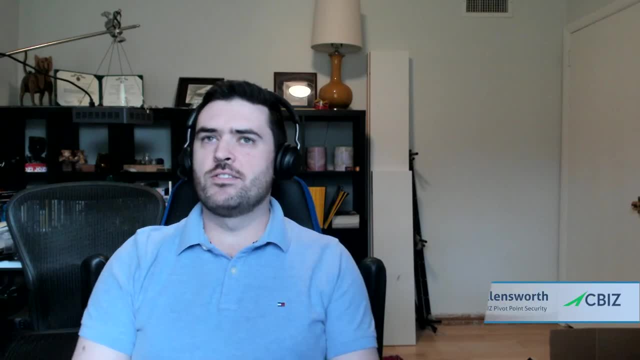 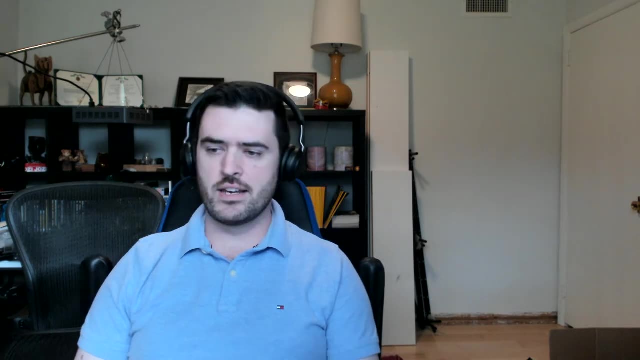 easy. Tell us a little bit about who you are and what is it that you do every day? Yeah, so again, Ariel Ellensworth. I'm an information security and privacy and AI consultant for CBS Pivot Point Security. And I'm an information security and privacy and AI consultant. 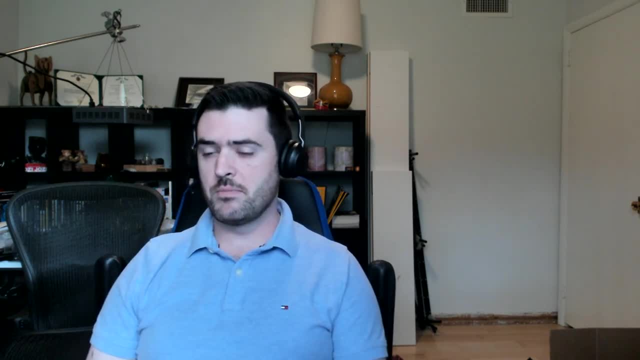 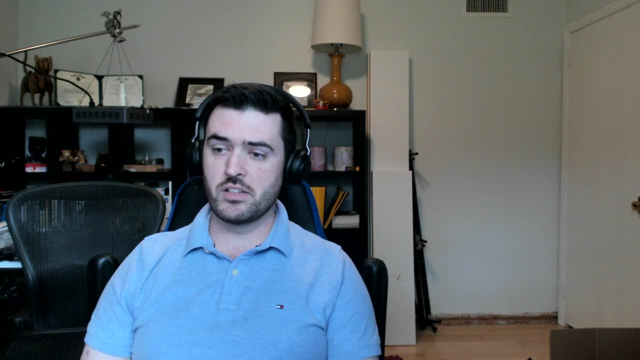 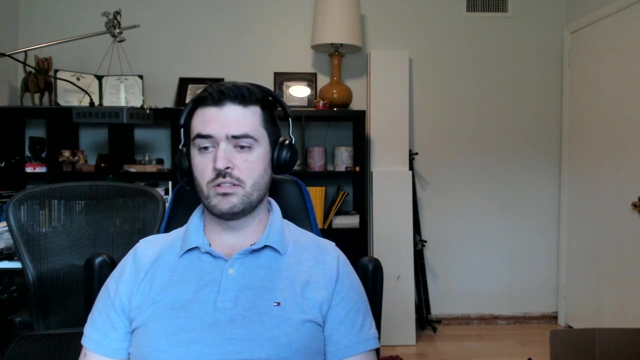 I help organizations implement frameworks that help them be provably secure and comply with their internal and external requirements. It can come from regulations or contractual requirements, or just the organization's objectives, And I also conduct a variety of risk assessments and internal audits associated with different types of frameworks. So essentially that's what I do. 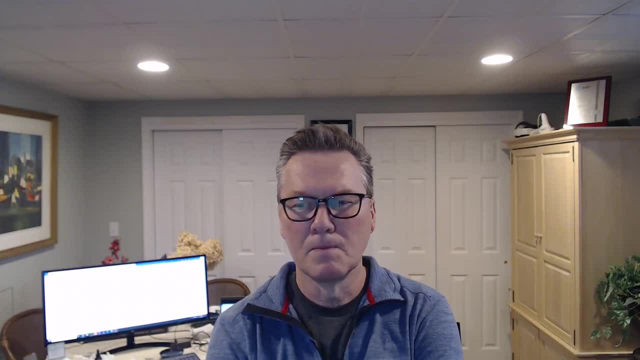 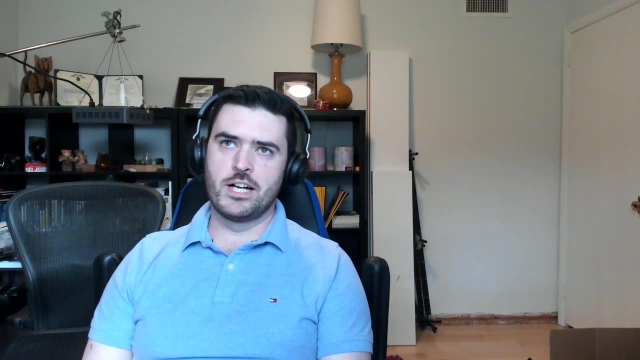 the majority of the time. Excellent, Thanks, Thanks. I like to ask, before we get down to business, what's your drink of choice? I really enjoy a good hazy IPA, But from time to time I'll also enjoy a vanilla porter. But I'm a. 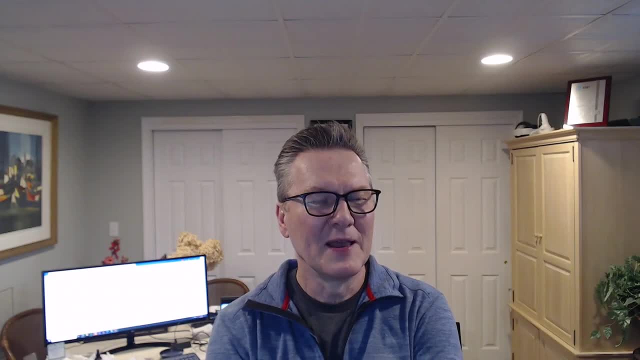 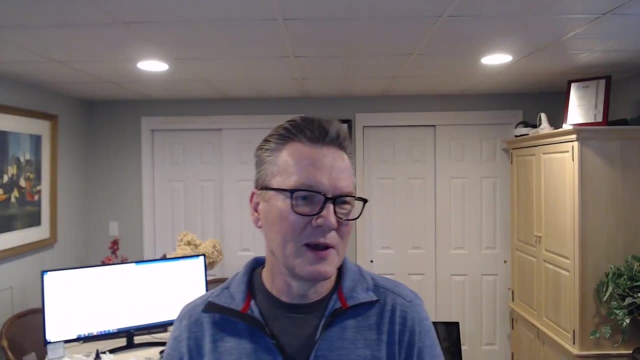 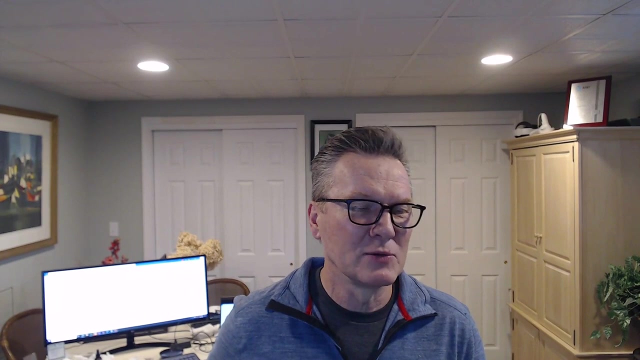 beer drinker? Yeah, I well have you had the Breckenridge vanilla porter. That's a nice little one. You can get it on, you can get on tap or you can get it in a bottle, But the Breckenridge vanilla porter is actually pretty, pretty darn good. I drink a lot of stouts. 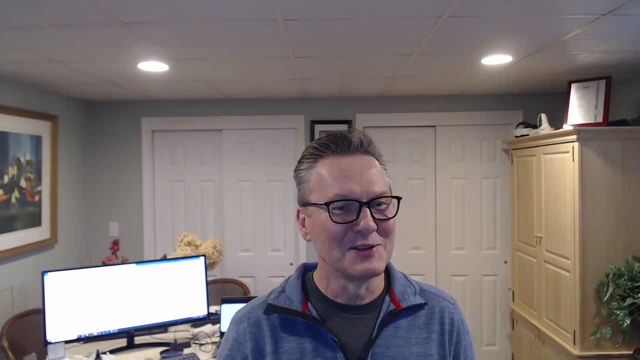 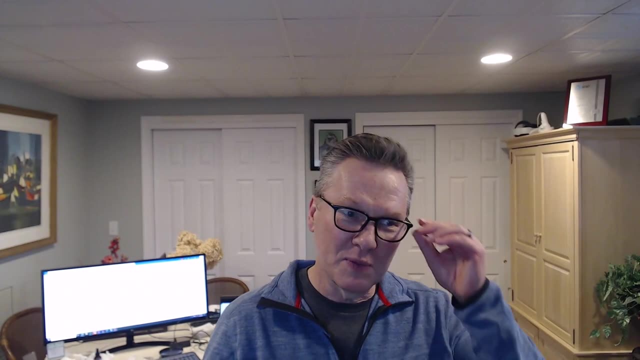 It's porters and stouts always confused me, despite the fact that I drink a lot of beer. That's yeah, there's such a subtlety between them that I don't really quite understand. Yeah, I always kind of tend to think of porters as being a little bit smoky, But then recently, 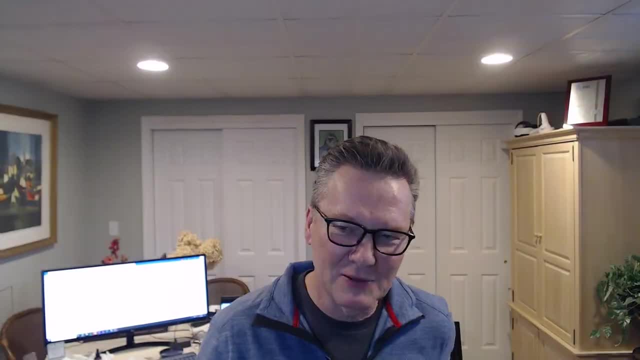 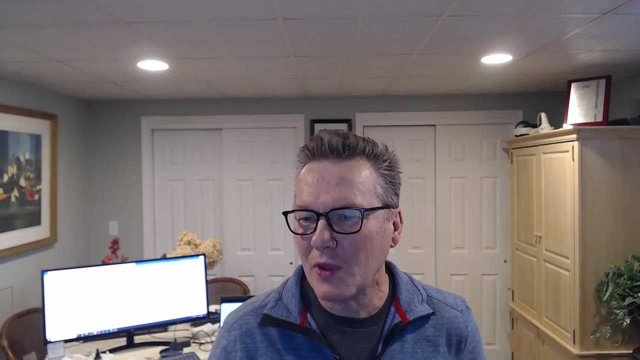 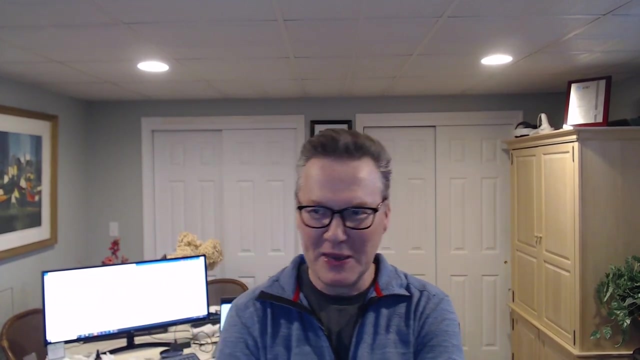 I've had a lot of porters that if I didn't look at the bottle I would have thought it was a stout. I figured that out between the two for sure. Yeah, so All right. So anyone over the last year that has consumed any type of media: 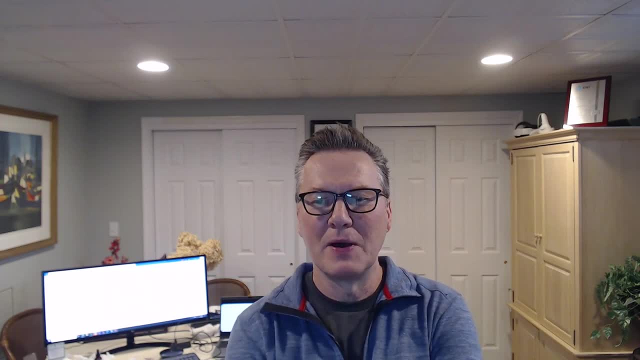 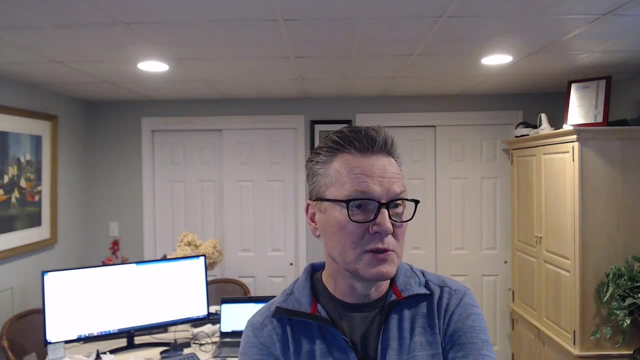 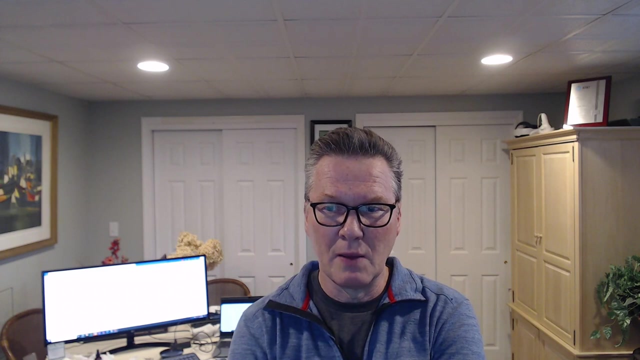 has probably gotten tired about seeing articles about AI and the way that it's going to. you know, the way that it's going to influence the next century, I guess For, I think, many organizations. it creates massive opportunities, right? New approaches, new services, new products. 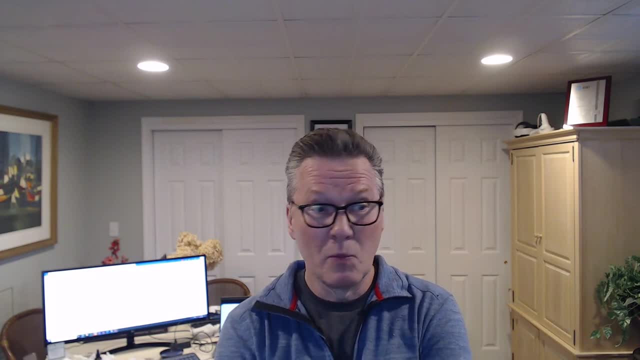 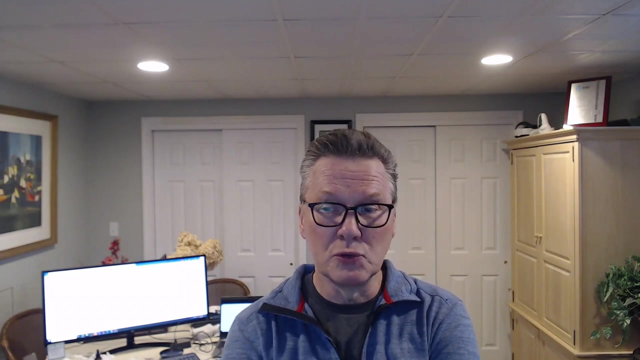 has the promise of driving employee productivity, But it also creates new types of risk that we really don't fully understand yet, And it also obliges companies to comply with relevant regulations and guidelines. So today, what I wanted to chat with you about is using AI in a provably secure and compliant manner. 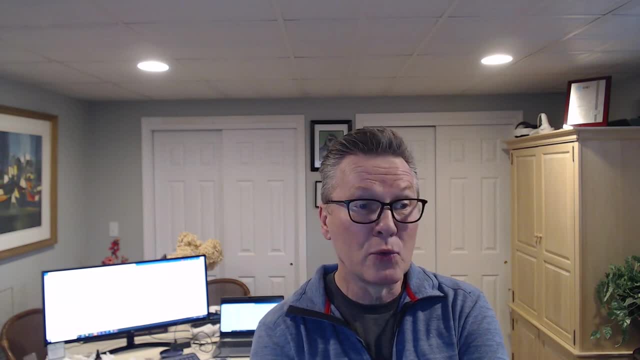 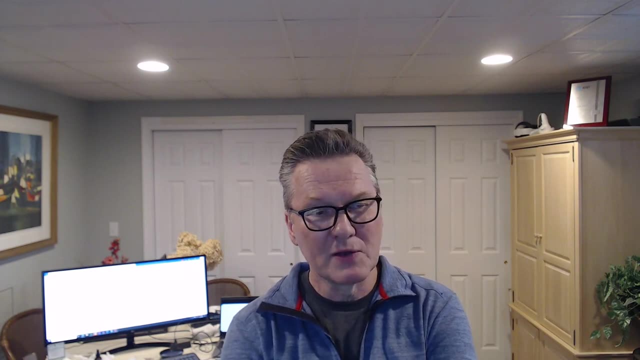 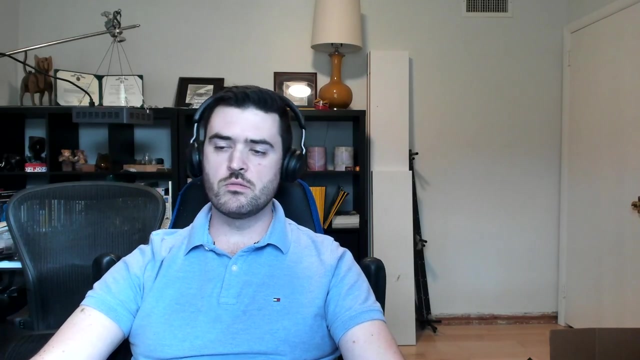 because that's suddenly become a contractual and or regulatory obligation for many of the organizations that we work with. So let's start simple. From your perspective, what are some of the risks that AI introduces to most organizations? Absolutely So. some of the ones right off the bat, and this has a lot to do with the large language models that we've seen come out. 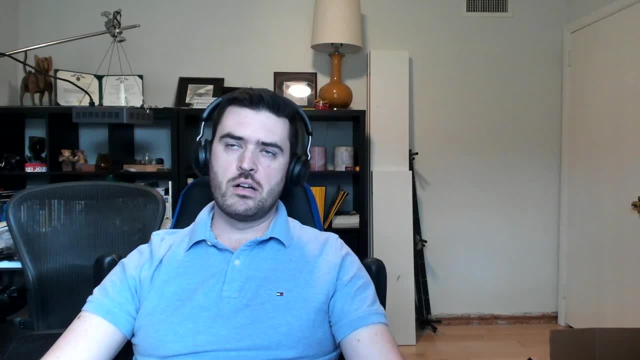 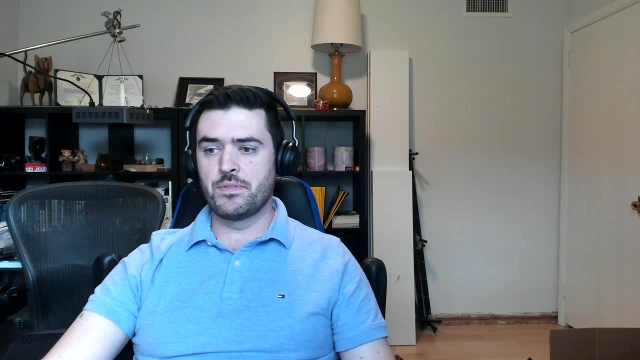 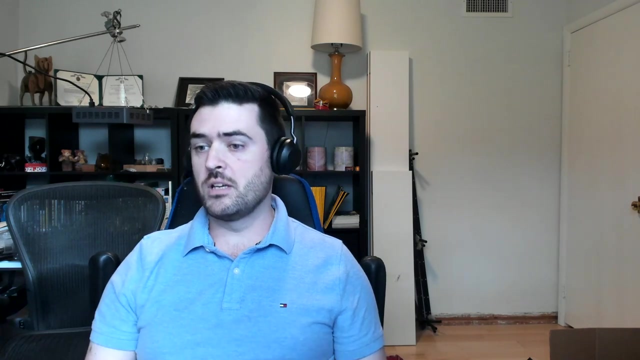 and become popular over the last couple of years, but misinformation caused by the models hallucinating, And for those who don't know what that is, the model can just output information. It doesn't mean it's correct, And so when organizations either formally implement a tool that leverages AI, or employees or people use a tool, 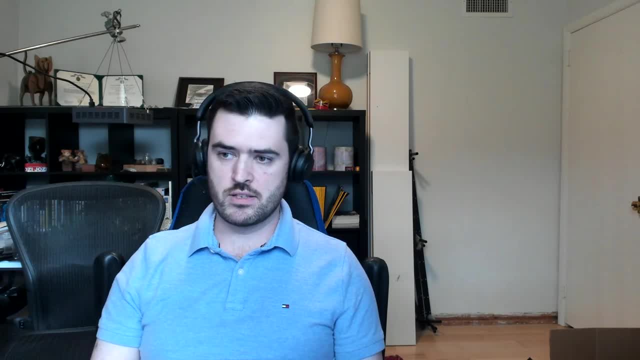 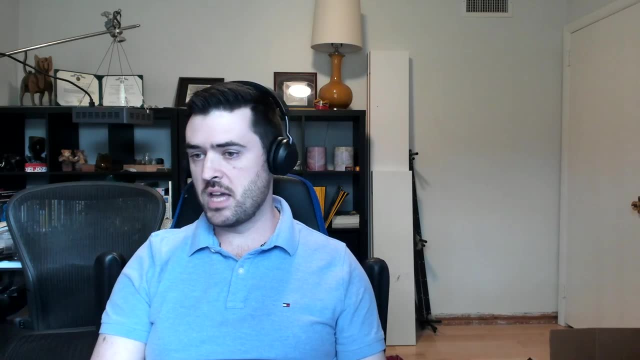 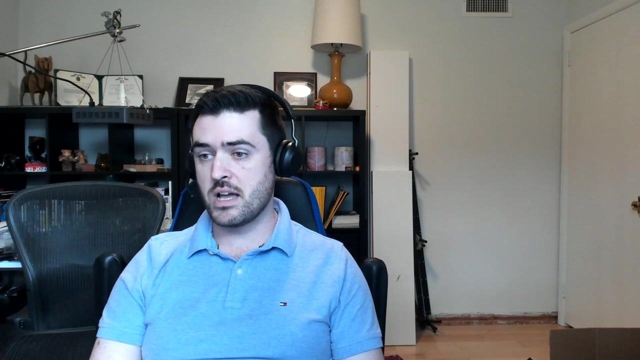 informally. sometimes they can rely on that information as if it's ground truth, And that's not always the case, And so, depending on the processes that the AI tool is supporting, you can have risky outcomes. You can have unnecessary bias or even potentially discrimination. 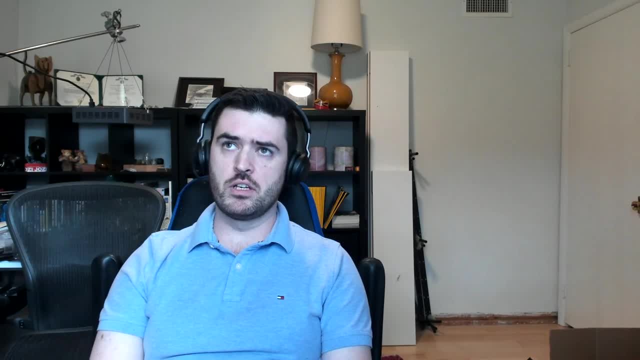 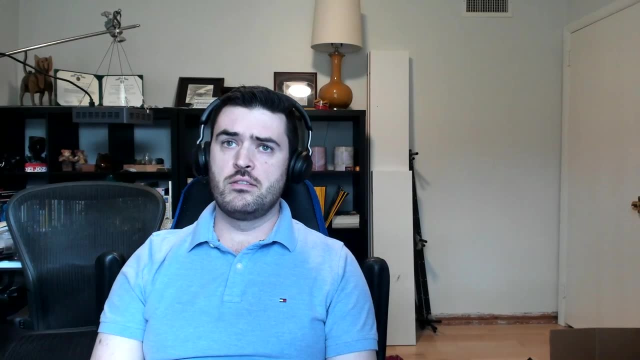 So hallucinations and misinformation is a huge problem if there's not verification done on the output of these models. And then also there's depending on how models are trained. it's possible if you haven't vetted and tested the model appropriately. 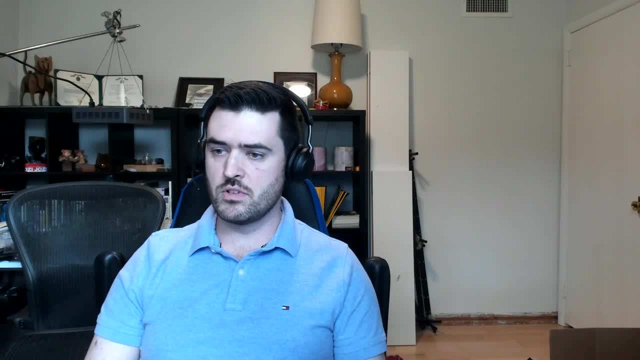 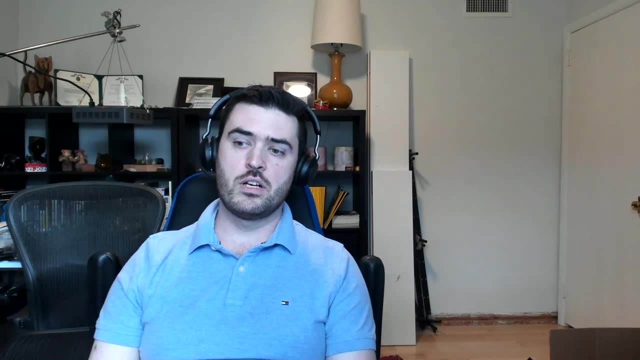 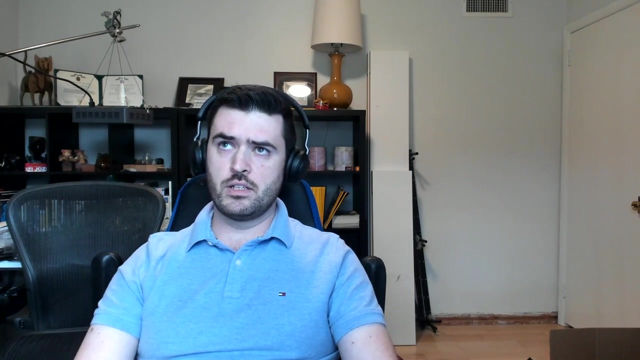 that you can sometimes extract some of the information that was used to train the model, And that's not always a good idea because it could be proprietary information, intellectual property, things of that nature. So those are really the two big ones, And then another one which has been really interesting is that there's a lot of information that's being used to train the model. 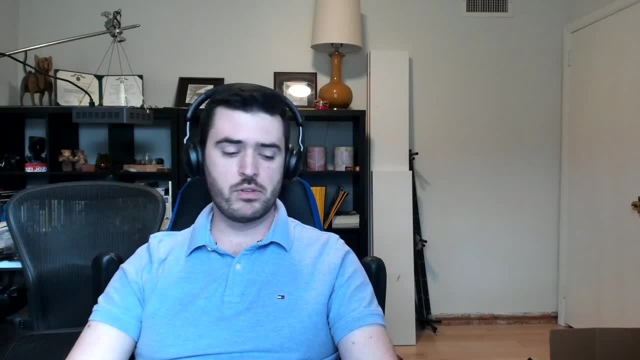 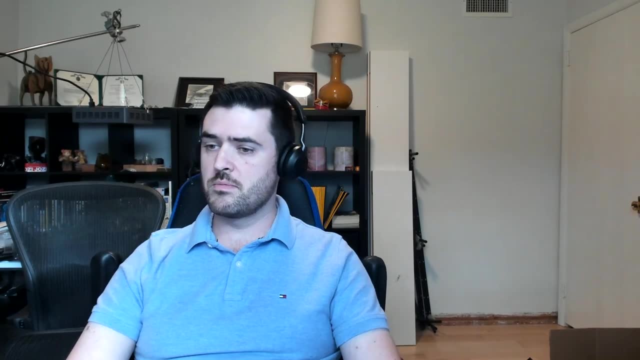 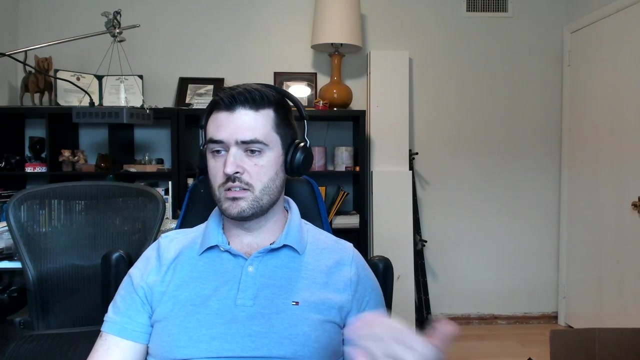 So one of the things that's been around for a while, but is just even more prevalent with the popularity of artificial intelligence recently, is automated decision-making risk. So this has been something that's been out for a while. So, for example, when you go to apply for a loan, in many cases there's an artificial intelligence that uses the variables from your application. 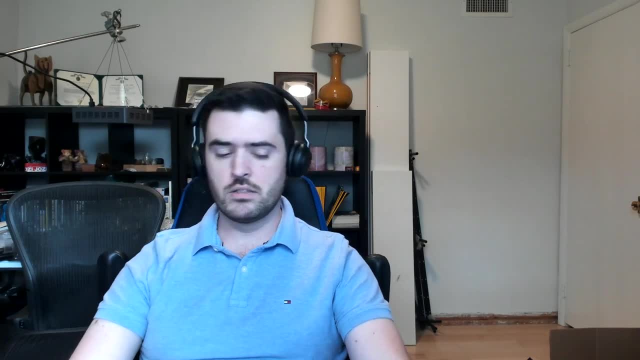 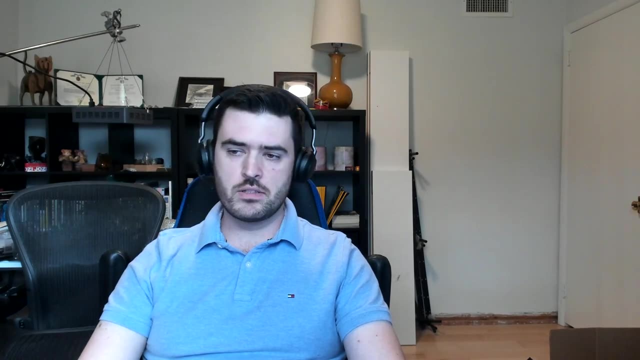 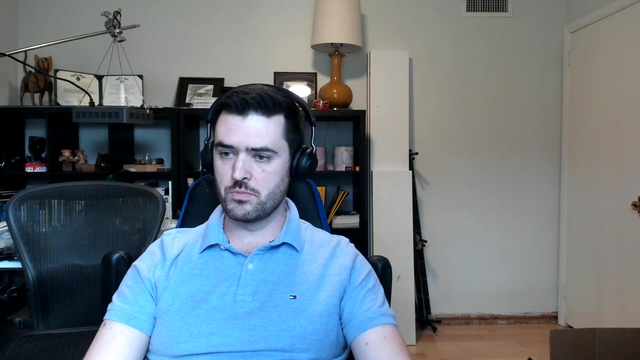 to determine the amount of risk to the bank of you defaulting on that loan, and it applies a specific interest rate. Okay, Now if the model is faulty or trained on data that is biased, sometimes that can cause discriminatory outcomes for certain groups of individuals. 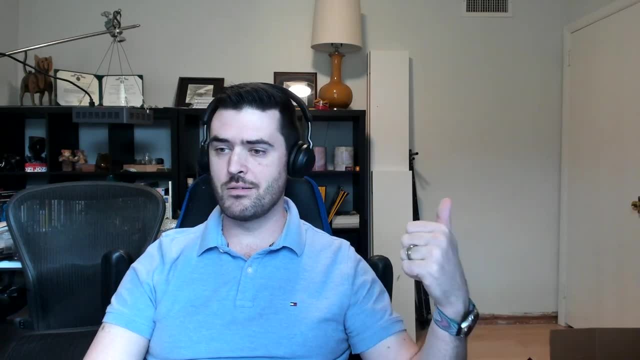 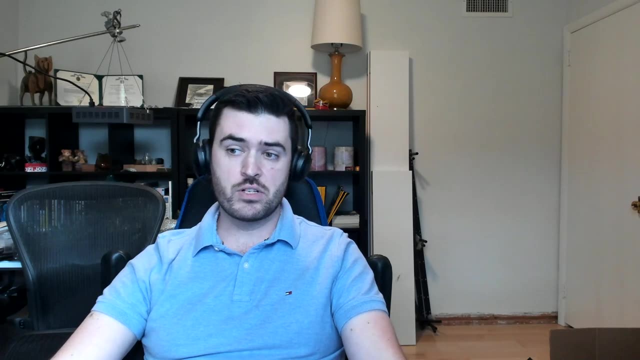 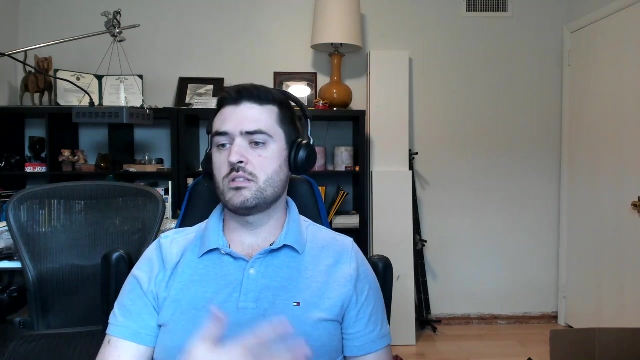 So some people may get a different interest rate based on faulty training data, when really they should be getting a more fair or perhaps a much higher interest rate than the model predicts. And this can apply across many different areas, things like insurance and finance and loans. 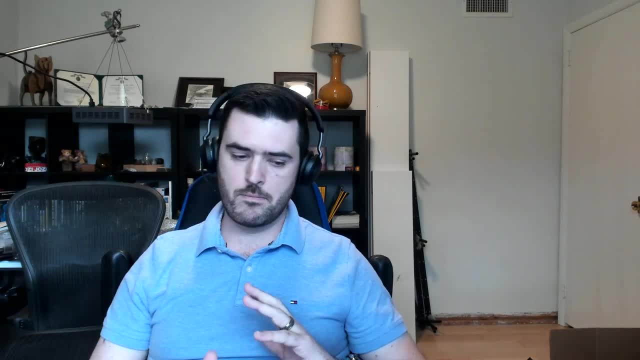 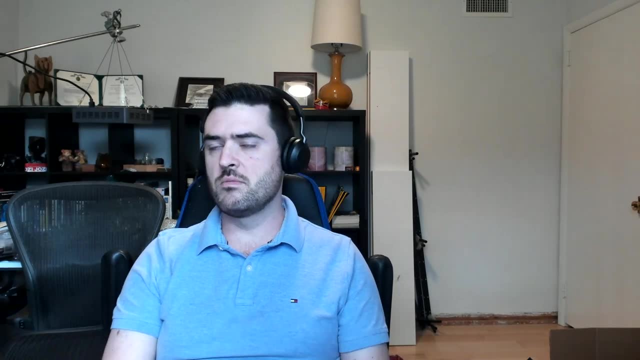 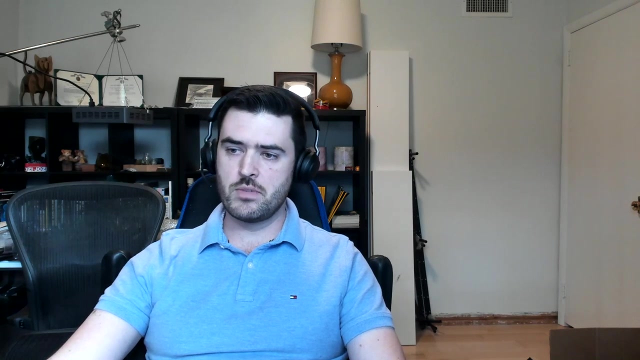 It's a really good example of this that's been implemented long before these large language models. But anytime an organization is trusting a model to make some sort of decision or even a recommendation that the organization is going to take into account, they have to make sure that they are not introducing bias, because they're going to be accountable for the discriminatory outcomes. 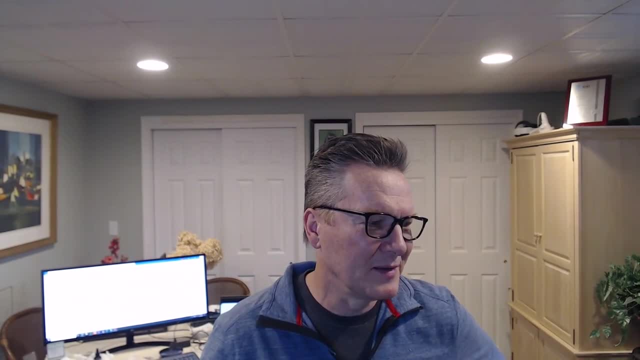 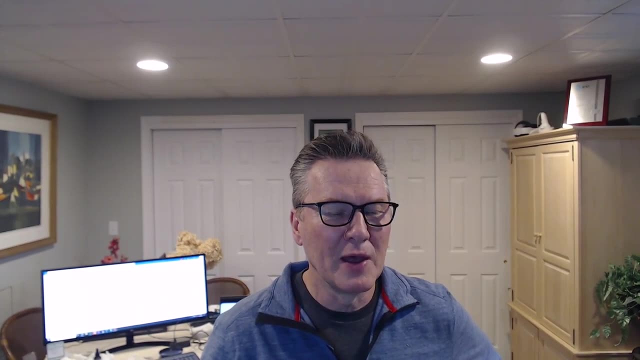 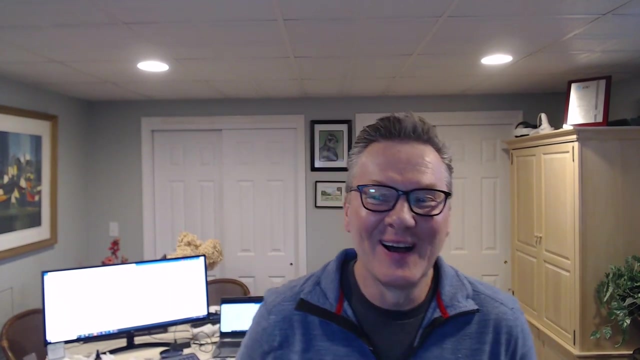 Yeah. So on that hallucination risk, I think the most famous, The most famous incident was the gentleman, a lawyer, who goes into court and he argues case law that the AI engine completely made up. So he cited up a legal precedent that the you know whether it's chat, GPT or whatever, it was actually hallucinated. 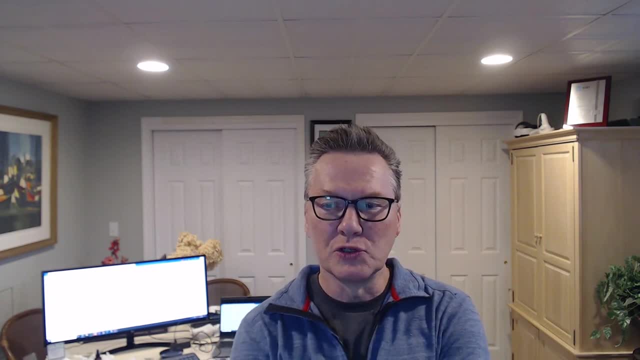 So yeah, that's scary. And then you know, on the usage side, right, one of the things I don't know: if you see, when you chat with people, when I start to talk about AI risk with some people, they're like no, no, you don't understand. 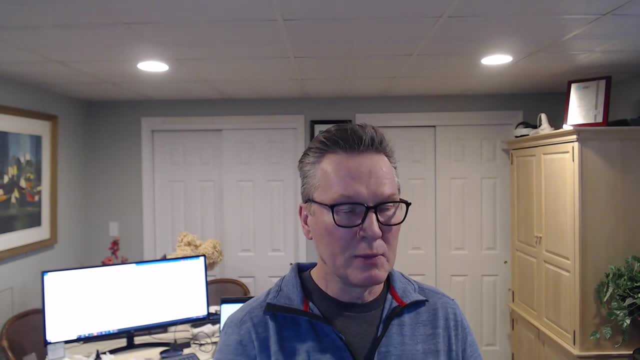 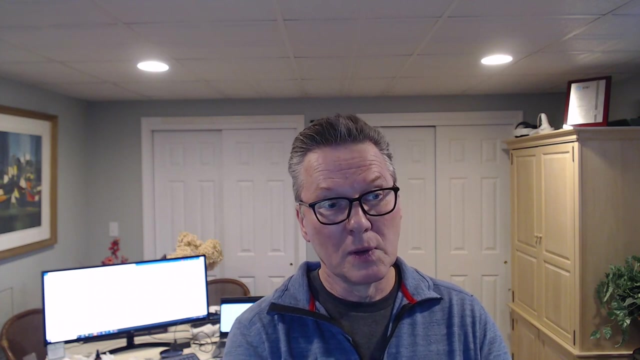 We don't, We're not doing anything with AI. We are not- And they mean they're not- developing AI-enabled applications, But I think people forget that AI is sort of becoming omnipresent in our lives and that, you know, they and their employees are using these tools provided by third parties that are using AI. 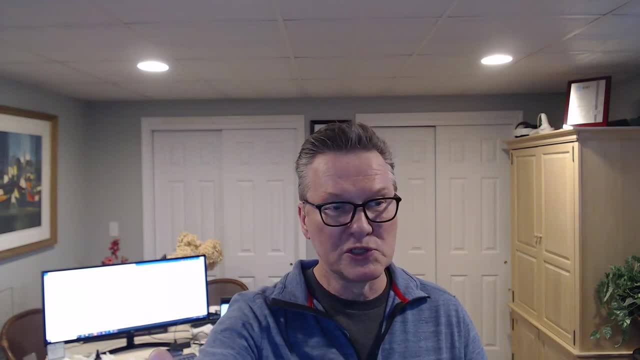 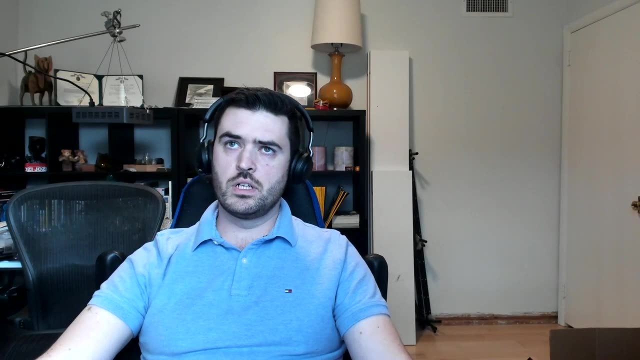 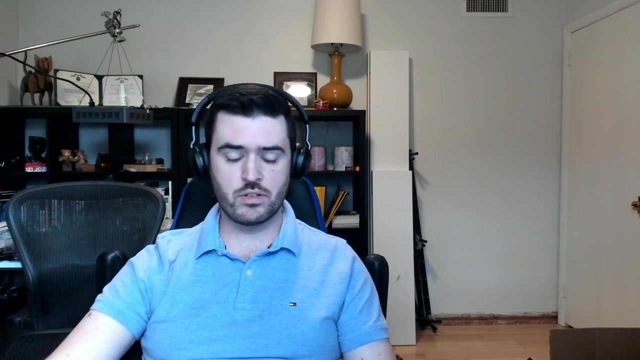 And I think that theoretically right. that imposes them to many of the same risks that they would if it was even their own tool. Yeah, absolutely, There's definitely a risk of Of data loss, for example, from employees putting proprietary information into chat- GPT, for example. 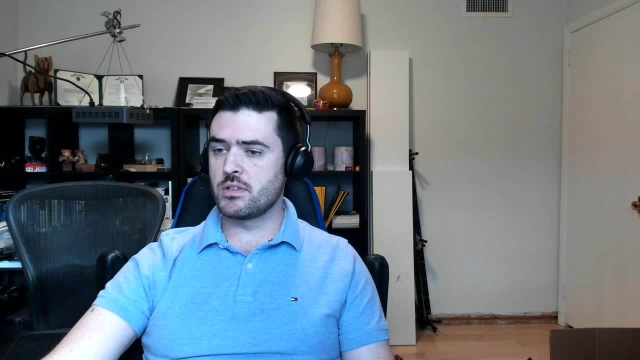 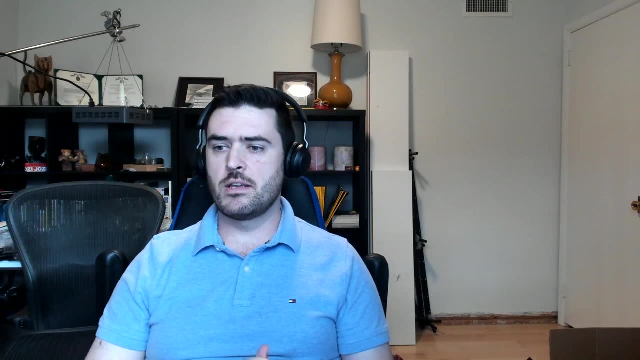 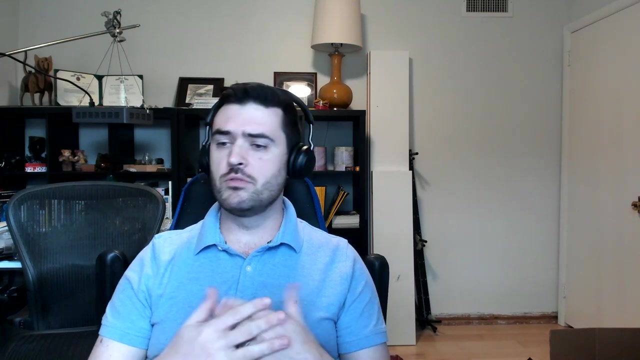 So let me talk about a similar scenario. right? So it's hopefully common knowledge and there should be training within most organizations that tells employees you don't send proprietary information to an email address outside the organization or you don't type in proprietary information into Google, right? 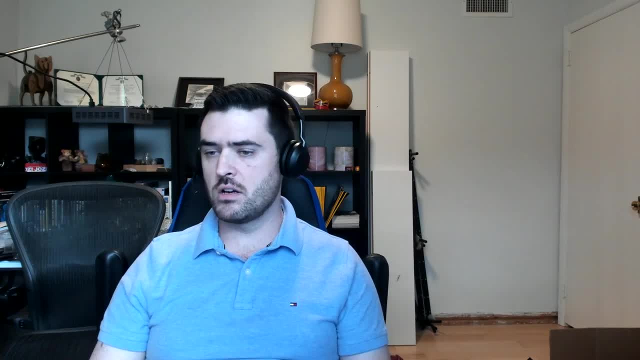 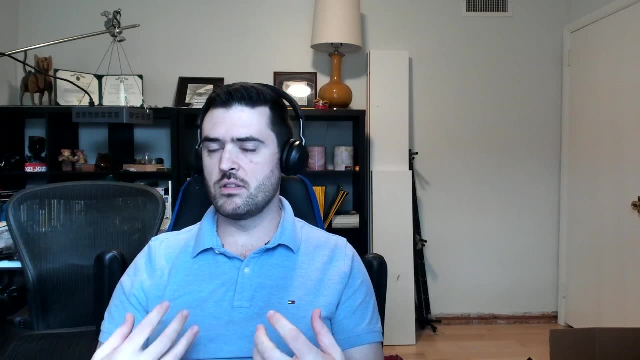 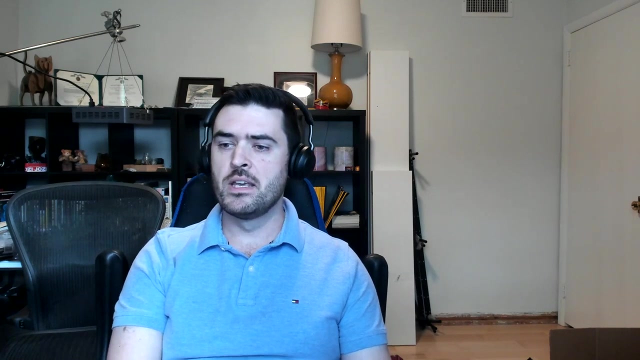 And so neither of those things are explicitly artificial intelligence, but there are policies on that and there's training so that employees know that the best practice is not to share that information. Well, artificial intelligence in large language models especially introduces this new type of risk, and people may not necessarily understand the activities that cause risk for the organization. 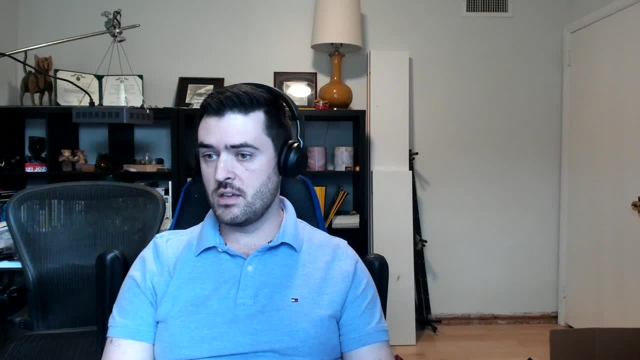 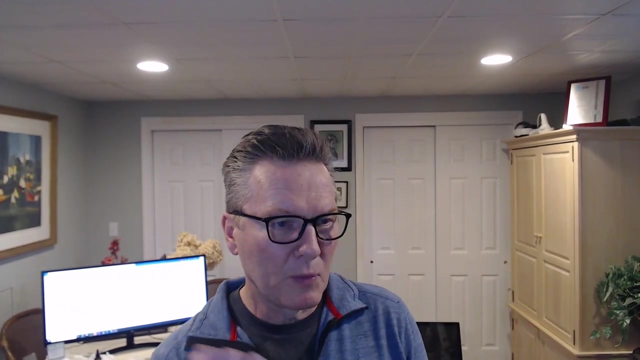 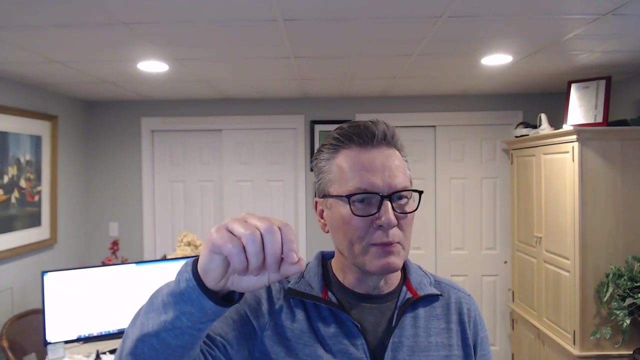 There may be excitement around improved efficiency, There may be excitement around the quality of the data that's being shared, And so there's a lot of risk around the quality of the data that people will be able to access and use right. So if it's an example that someone is typing into their phone or someone is trying to make a call to an email address, they may not be able to access that information. But if it's an example that someone is typing into their phone, they may not be able to access that information, And so there's a lot of risk that can be caused by that. So there's a lot of risk that can be caused by that. 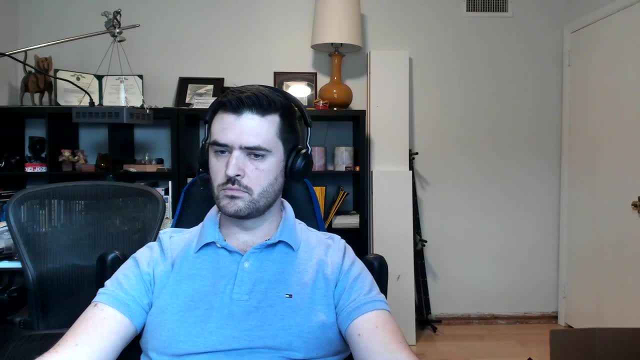 And sometimes that can cause people to miss the risks, like data loss, from inputting proprietary information into these models. Right, So as an example, correct me if I'm wrong. you know more than I do- become part of the large language market. Exactly, And not just ChatGPT, but the different. 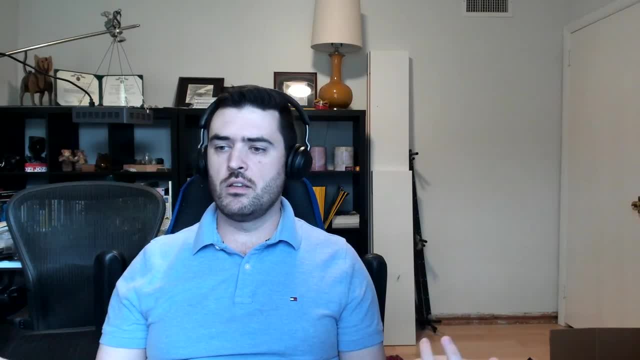 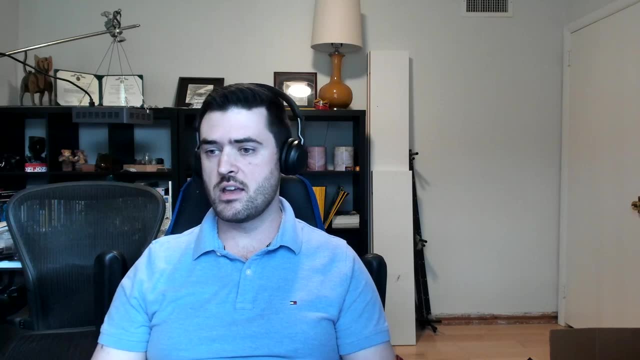 models that are available and different tools that are available. You have to review the terms and conditions and the settings and features of each of these tools to understand: are you going to be compliant with your organization's policies as they are? And it creates a very ambiguous 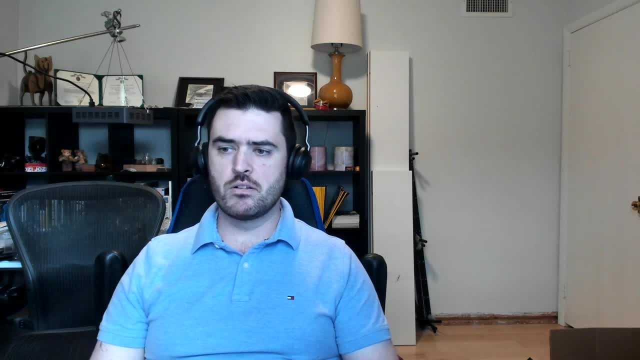 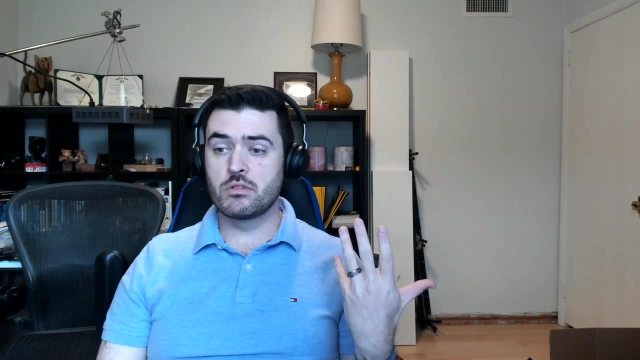 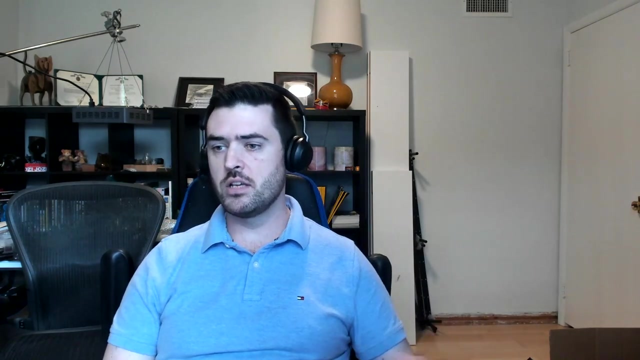 landscape of how to use these tools, And so it can be really difficult for organizations to address this, because this came on so quickly. And, for example, I use ChatGPT all the time. I don't put proprietary information into it at all. I use it for more creative type work. But 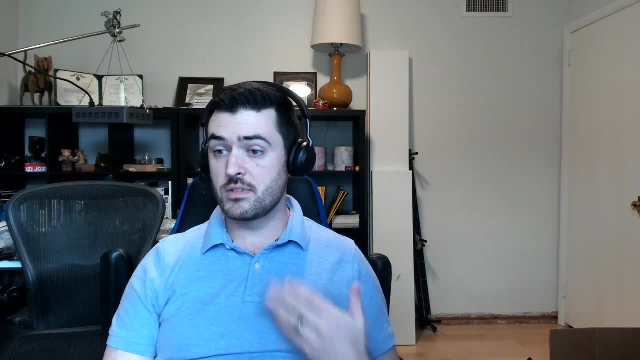 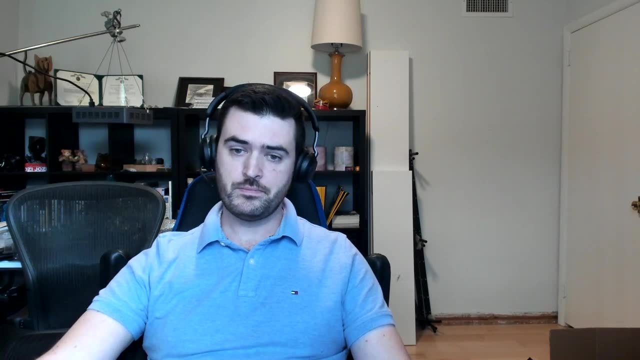 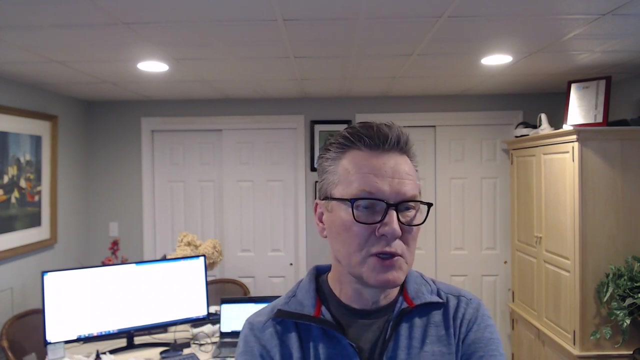 at the same time, I've read and understand CBiz's policy on the use of artificial intelligence. Not every organization has a policy like that. Great, All right. So let's talk about something which is driving a lot of the conversations that I'm having with 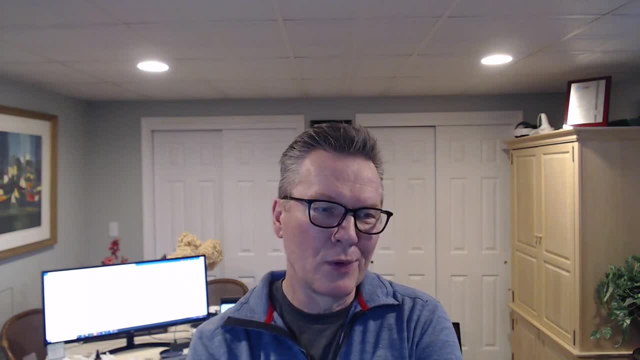 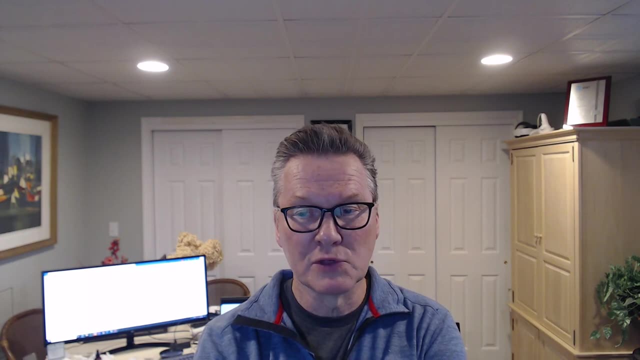 our audience, and I'm sure you as well- Regulatory and what I'll call semi-regulatory guidance. We've got the EU Cyber Act. We've got NIST, AI, RMF, the Risk Management Framework, The Presidential Executive Order- I think it's called on the Responsible Use of AI. What is it that? 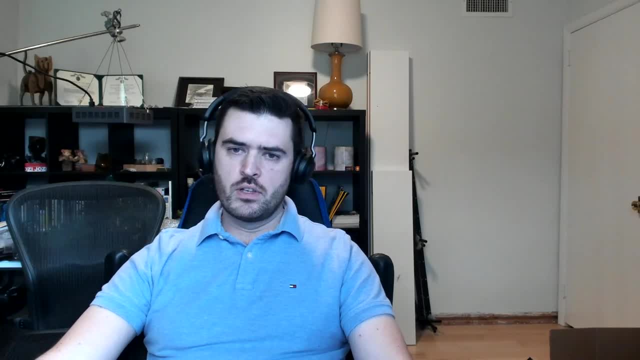 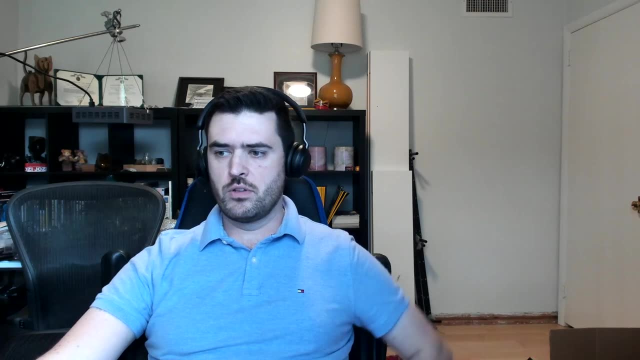 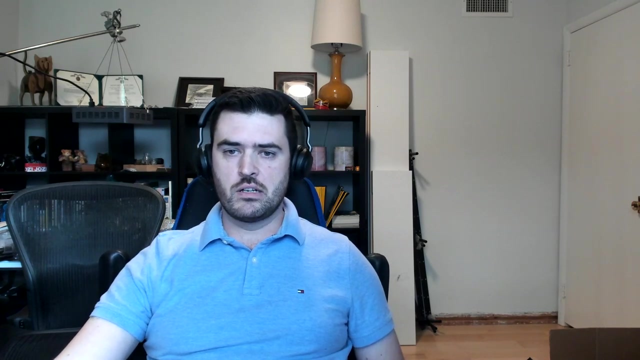 they specify. Are they all pretty similar? What are people up against? I'll start with the EU AI Act. I believe that's the one that you're referring to, because there's also Okay. Yes, So the AI Act was actually adopted by European Parliament on March 13th of this year. 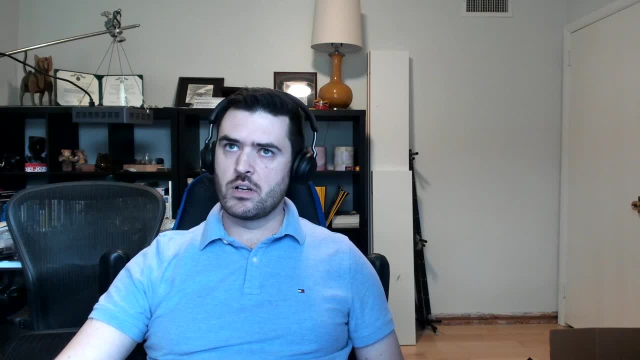 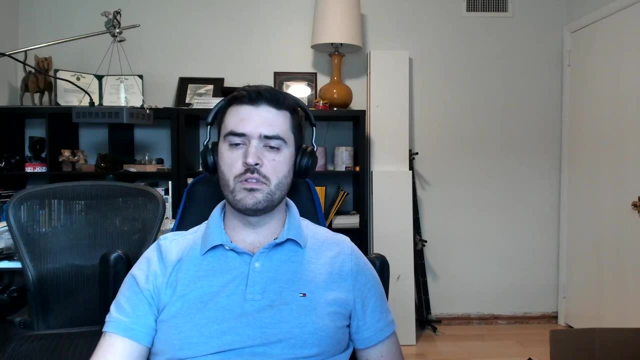 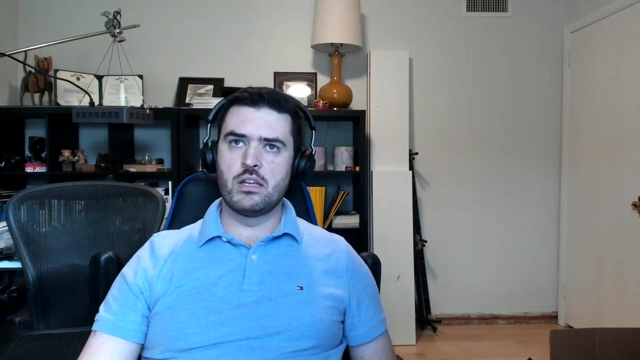 So that establishes a regulatory framework on the development and use of AI within the European Union and that affects citizens of the European Union, And so it's very similar to the GDPR that has been out for many years, and so, while this is, you know, a regulation within the eu, it applies in. 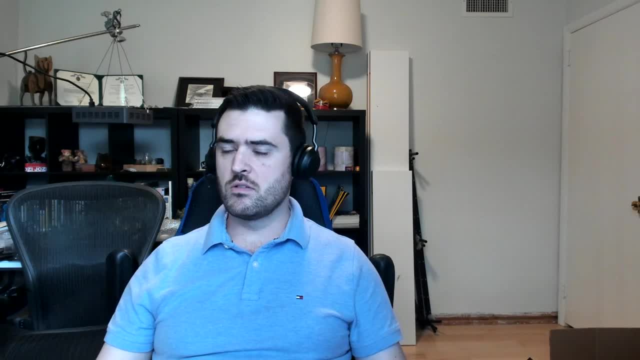 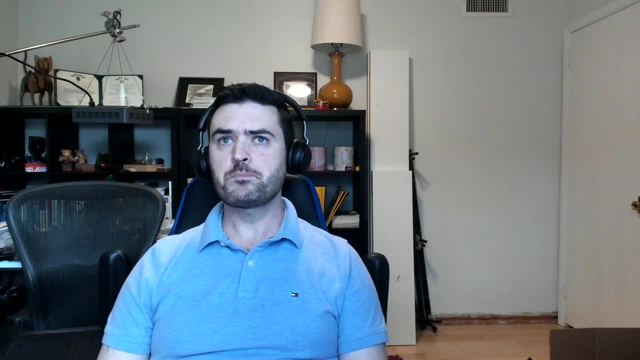 much the same way as the gdpr, and so at a very high level because it's a quite large um piece of legislature. but it requires that organizations classify their ai systems into specific risk categories and then, depending on the outcome of that categorization, they have specific requirements. 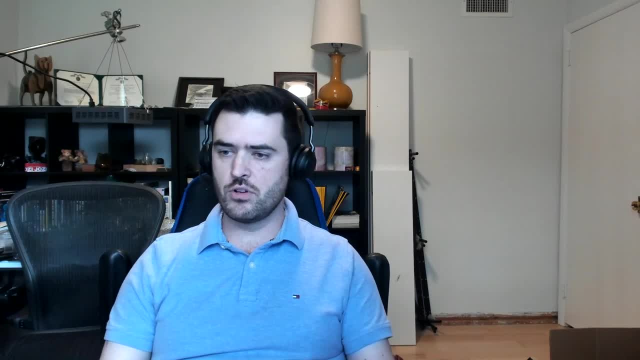 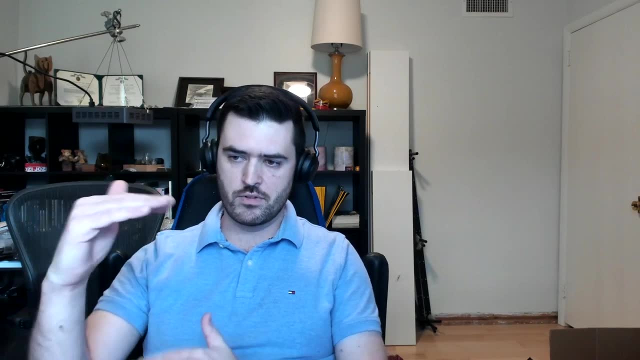 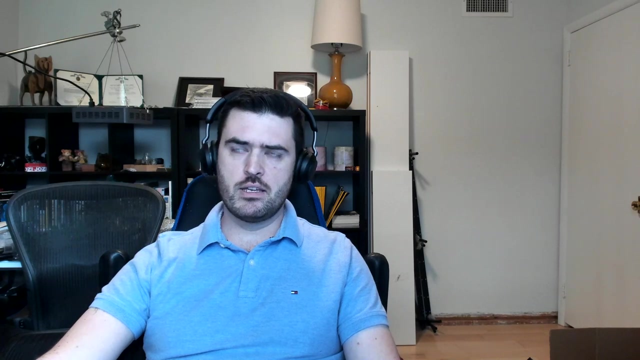 they have to meet within the law. and then, how do you know this is applicable to you? well, there's a variety of criteria, but fortunately they've developed a tool- it's kind of a quick questionnaire- that allows you to evaluate whether or not this applies to you or not. um the nist ai risk. 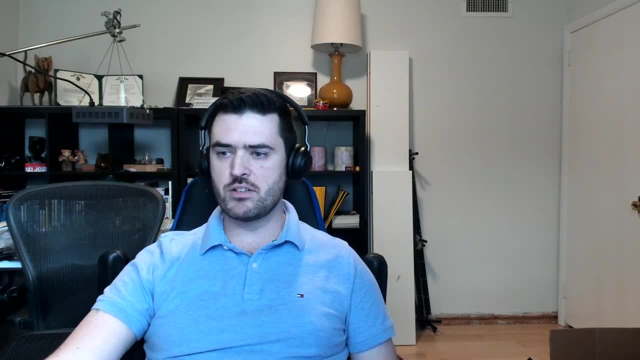 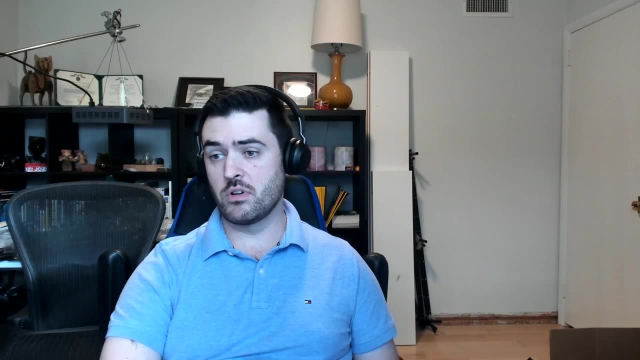 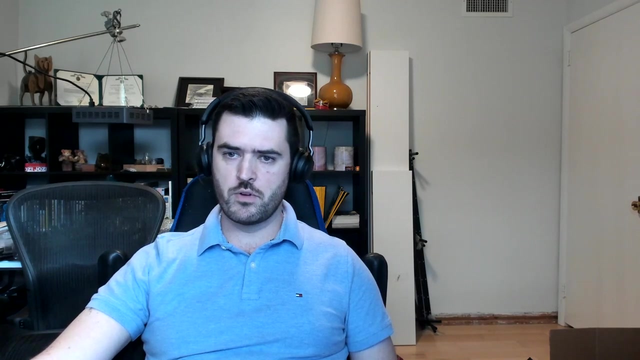 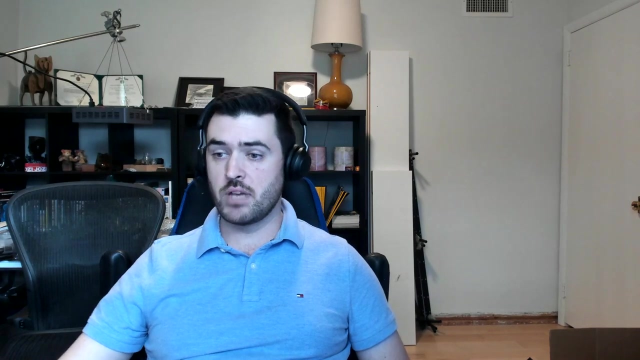 management framework. that is not regulation at all. that just provides really good targeted guidance on how to implement a risk management framework for artificial intelligence and so that uh specific framework focuses on four areas. it uses a govern, map, measure and manage model. um, and that's just really um. 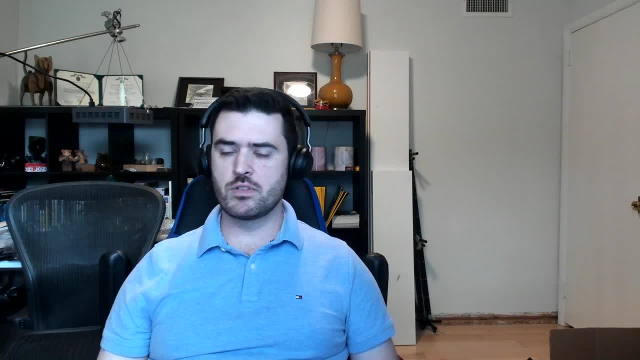 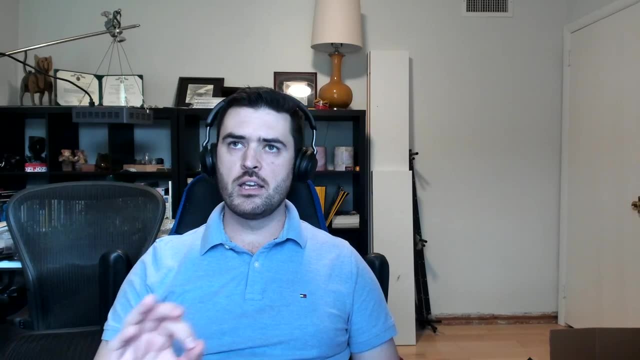 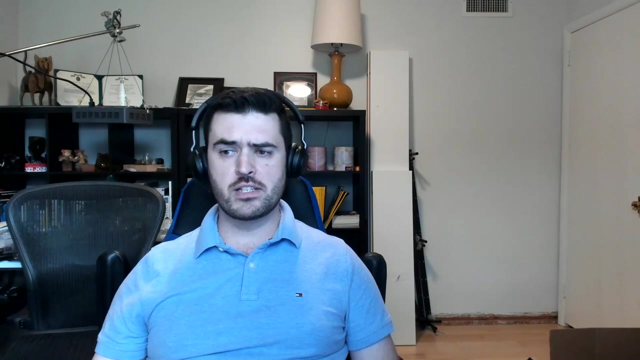 again has very targeted guidance in each of those areas. it's it's one of the the pieces here where, if an organization is saying what can i do to address the risk around ai, it's incredibly helpful because it's specific, it's prescriptive and it has um really good examples and 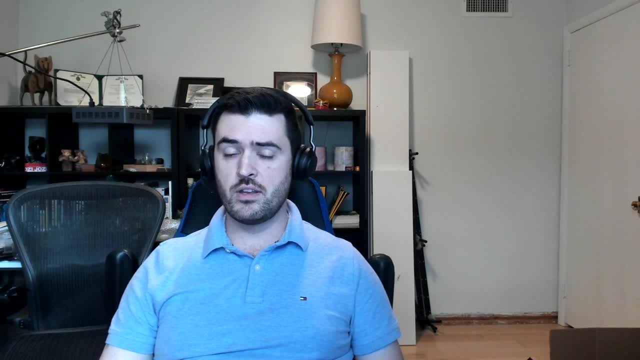 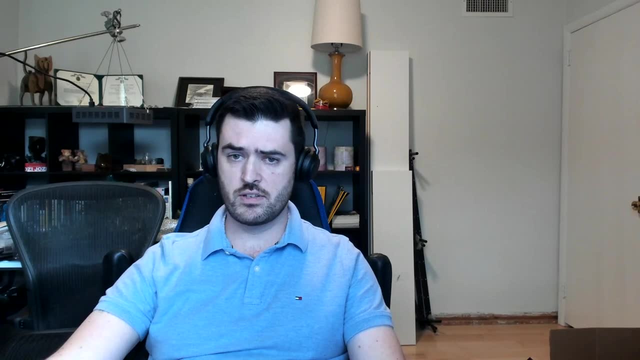 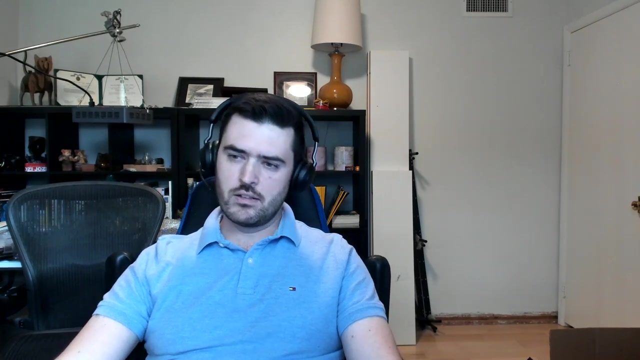 it has an accompanying, accompanying playbook to go with it that helps you understand how it applies to specific types of companies and specific types of artificial intelligence risk. and then finally, uh, with the executive order, that is a little less applicable. i would say, um, as far as like. 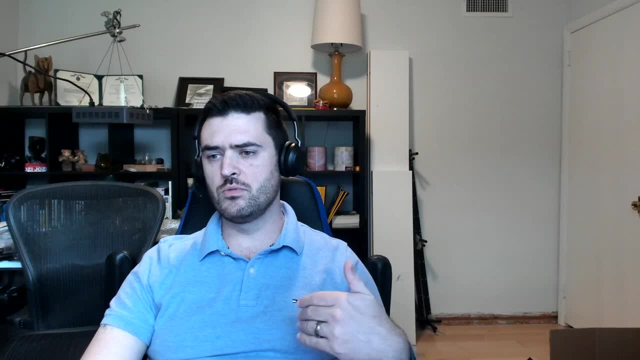 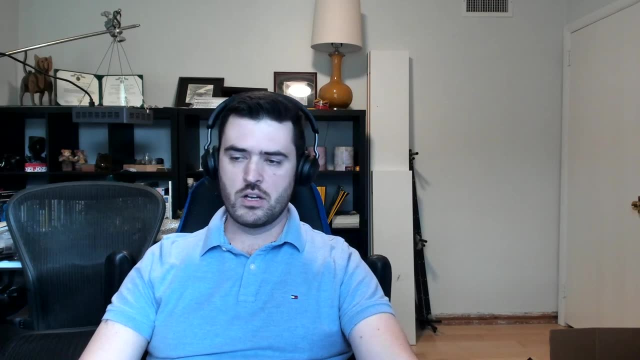 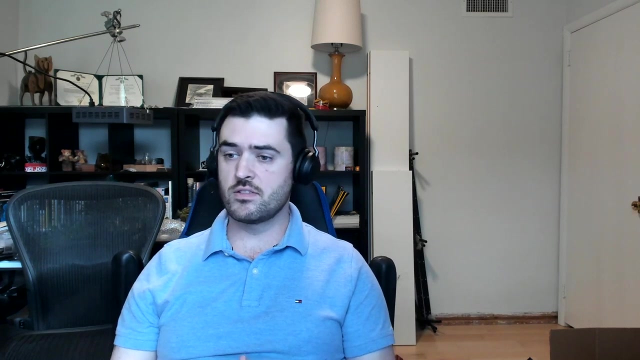 a regulation because it's more of a target model, but it is something that's more of a in order to government agencies to develop standards and develop regulations on the use and development and governance of artificial intelligence. so it's the executive branch recognizing that there are significant risks and opportunities associated. 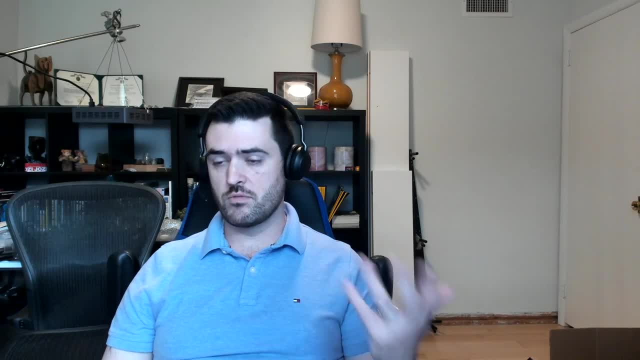 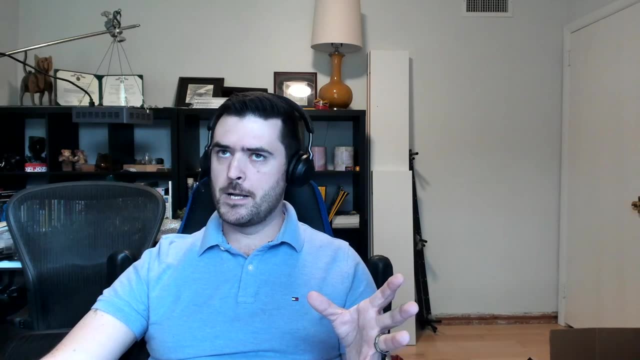 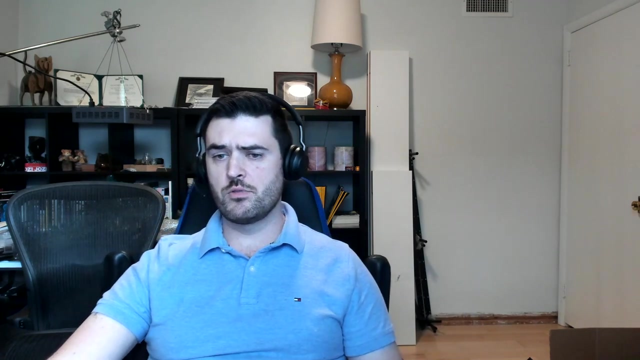 with this, and so we need to put some significant resources towards understanding what those are, can take advantage of the opportunities. So they're not really similar, but they're all in a response to this rapid development of artificial intelligence and large language models and for it being incredibly relevant to a much, much larger group of people. 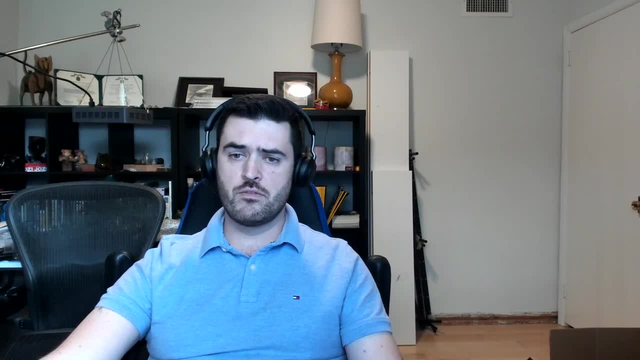 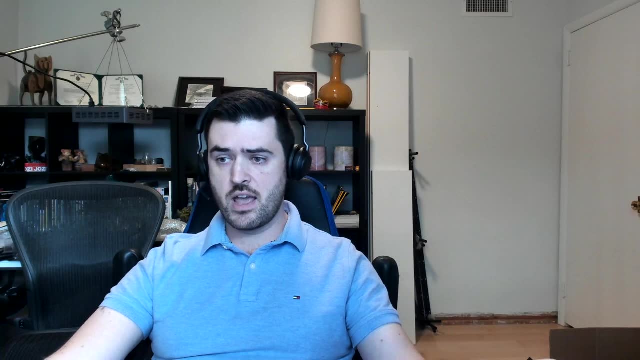 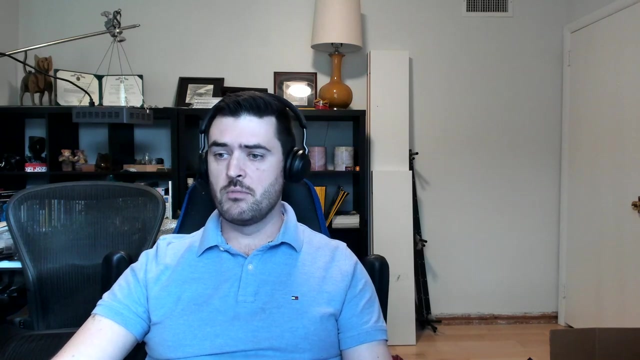 and with people having a general knowledge of it, And so organizations should definitely just watch this space. leverage NIST, AI, RMF as a really good resource If you want to understand how to manage AI risk. pay attention to the EU AI Act, see if it applies to you, And then, of course, 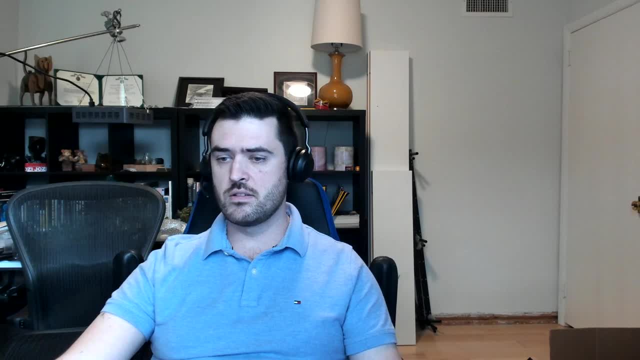 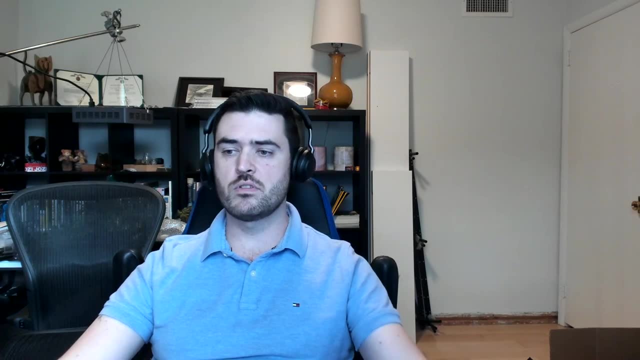 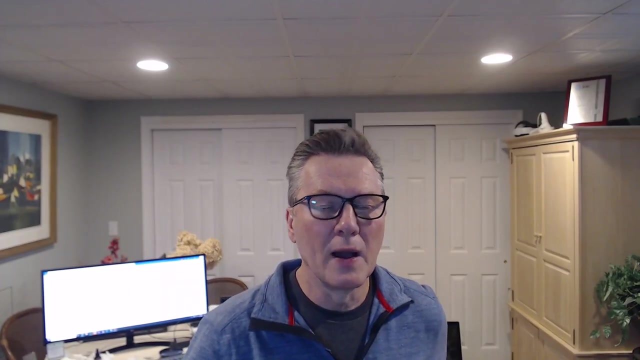 just pay attention to the executive order and news and updates around that, because you may find there are new regulations or new standards that come out as a result of the orders that's been given to the different government agencies. Robert Leonard, Yeah, I would argue that the presidential executive order, while not yet important, 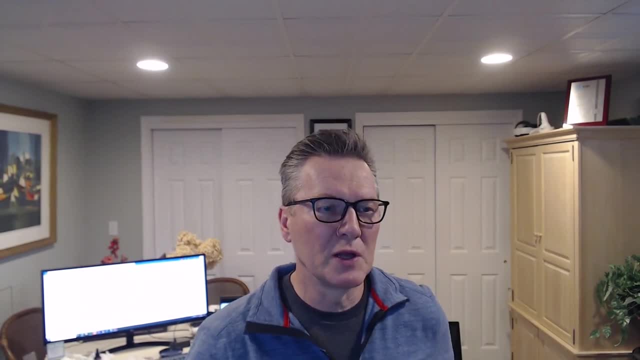 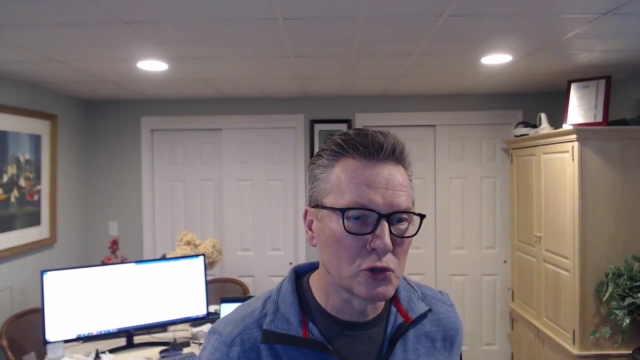 what it portends is because we know from previous presidential executive orders what happens is. this was an example with the NIST 800-218, the secure software development that stemmed directly from a presidential executive order on said issues. So I think 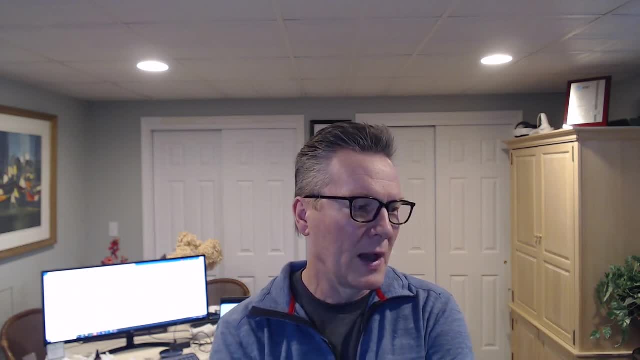 we're really what we look at when we look at the presidential executive order. I think it gives you an idea of where our government is going. And then we know that our government is increasingly flowing down regulations, you know, to organizations within the United States. 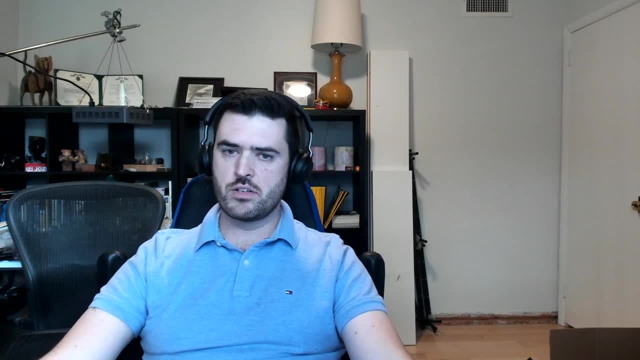 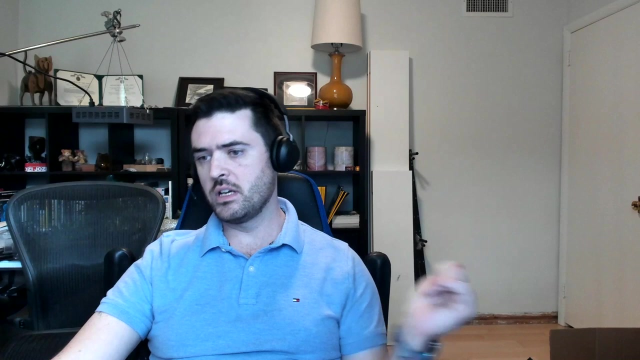 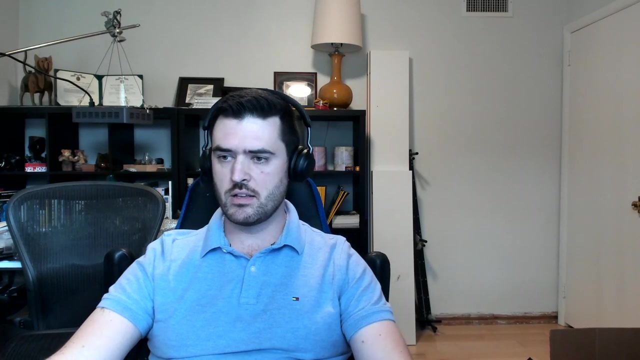 It's really good. It contains some excellent information as well to understand how the government views specific risks around AI and opportunities around AI and maybe where the government falls short. So what's interesting is, as this space moves very quickly, there may be portions of the order that are becoming more relevant in areas that tend 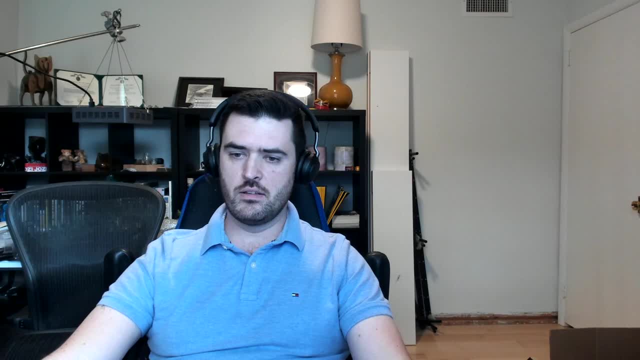 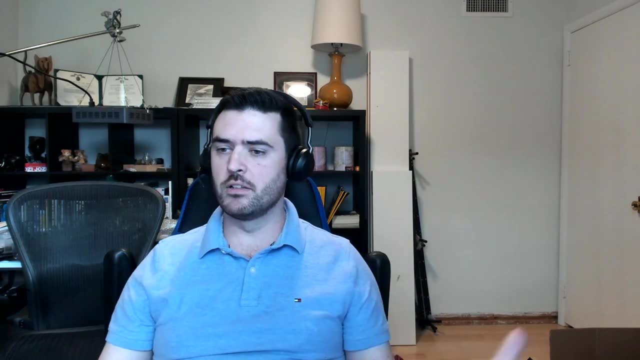 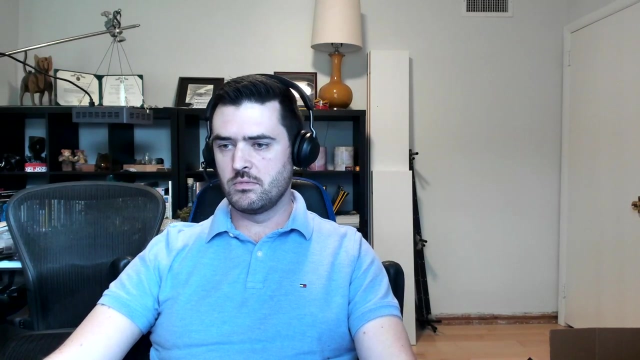 to be gaps, But it provides really good direction And, you know, a pillar for organizations to understand if there are requirements within the United States government that apply to organizations for some reason. David Fubini, Yeah, Robert Leonard, Okay, We can understand at least where this is going. 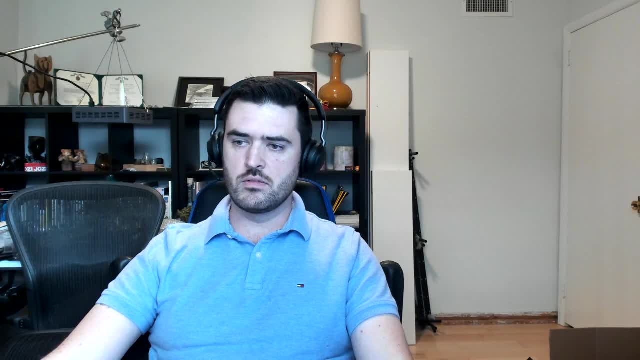 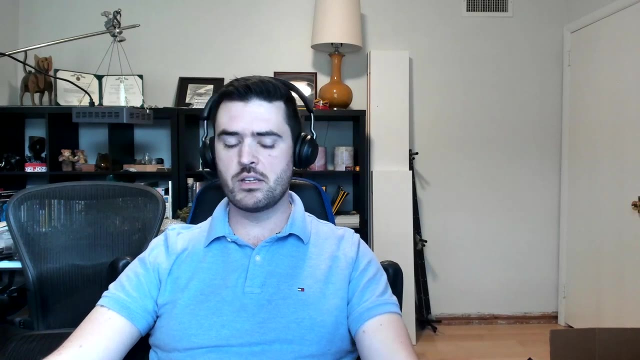 I think it's going to take some time for these government agencies to develop the guidance or standards that the Biden administration is calling for. But if anyone is curious about the executive order, I highly recommend reading a summary of it, because there's a lot of very, very relevant information. 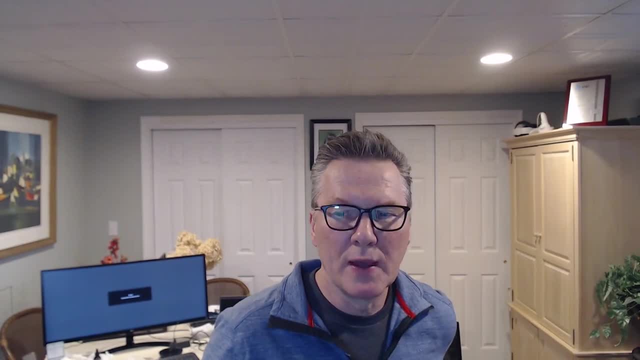 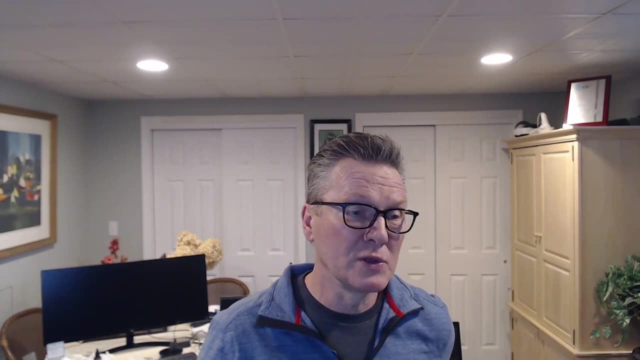 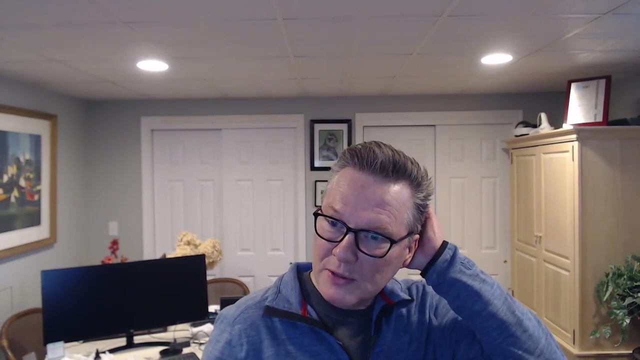 Yeah, I agree completely. So I know that we as an organization, and you personally, are pretty excited about the new ISO 42001 standard. It's a certifiable standard relating to IAI. Tell us a little bit about what it is and how can it be used to address the risks and the compliance requirements that we've just discussed? 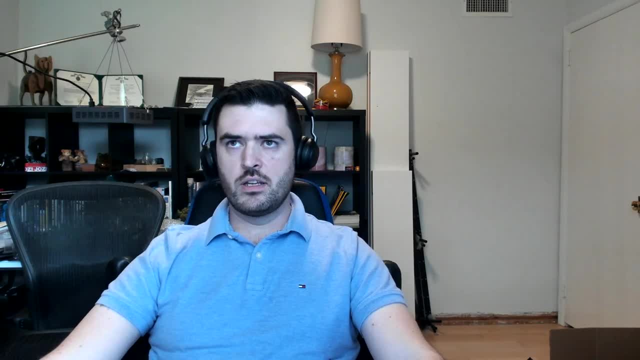 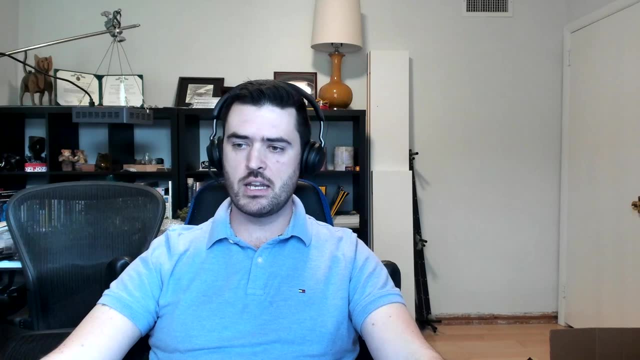 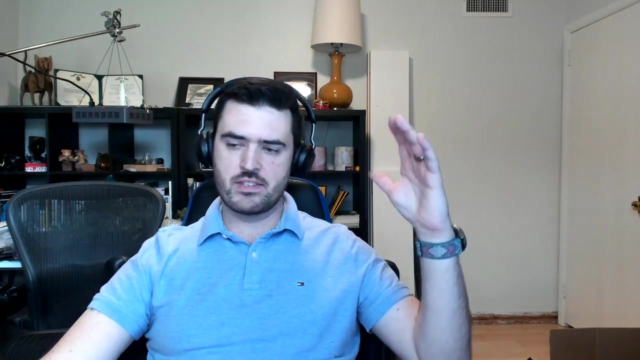 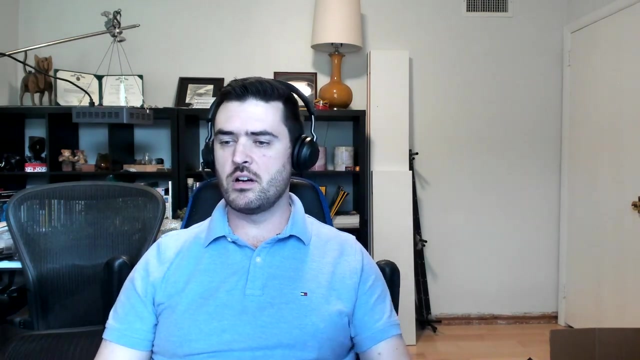 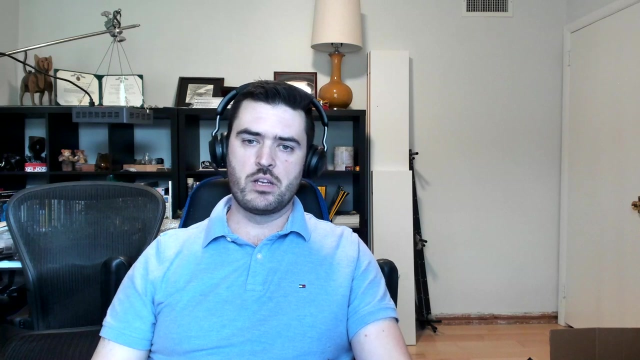 Absolutely So. ISO 42001 is internationally recognized. It's a recognized standard for implementing and maintaining an artificial intelligence management system. And so there are essentially there are seven main clauses that establish kind of framework requirements, And then there are a set of controls unique to artificial intelligence that help support those management requirements. 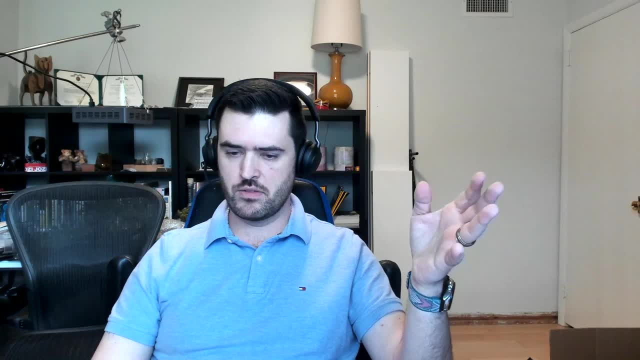 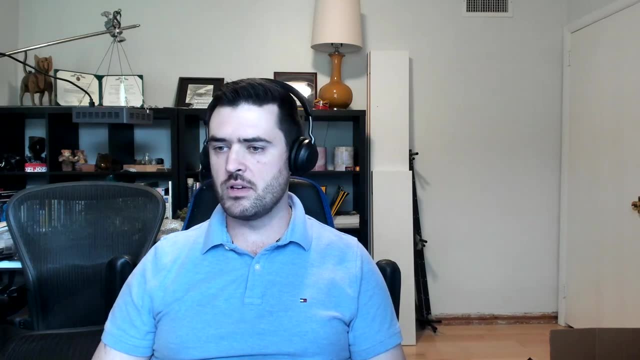 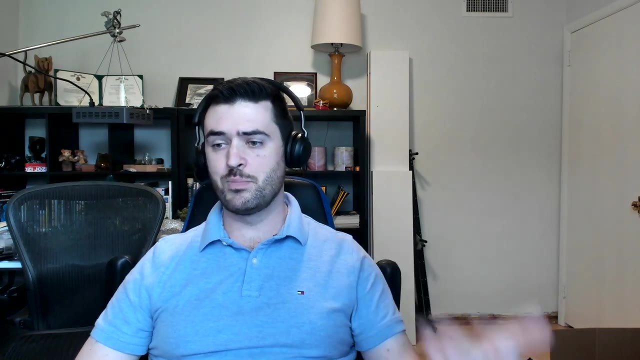 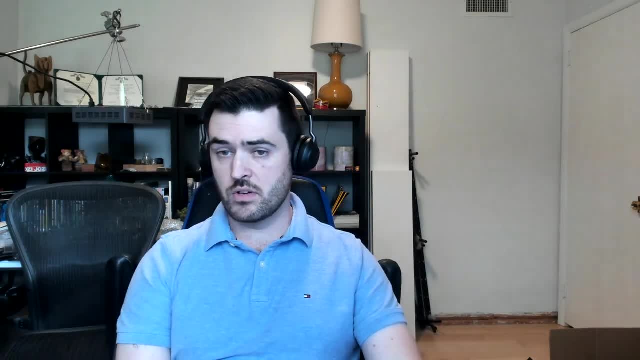 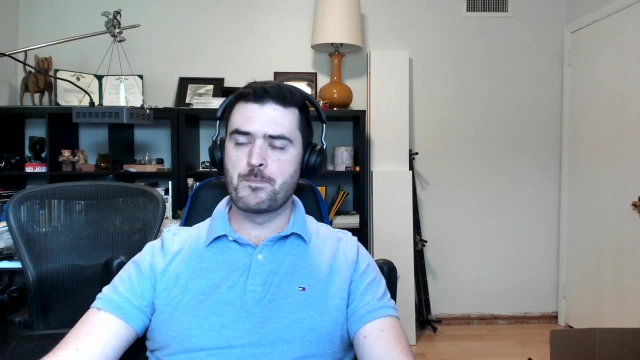 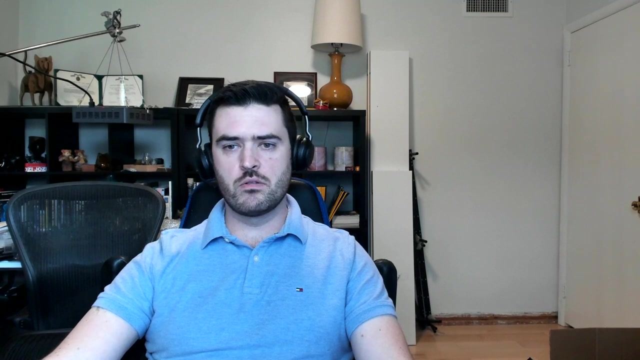 Also legislative and regulatory requirements, as well Organizational objectives, And so it's. it's a fairly- It seems like- a lightweight standard, because there's only 39 controls. Okay, however, it's, it's quite unique. so organizations that haven't uh taken a formal approach to. 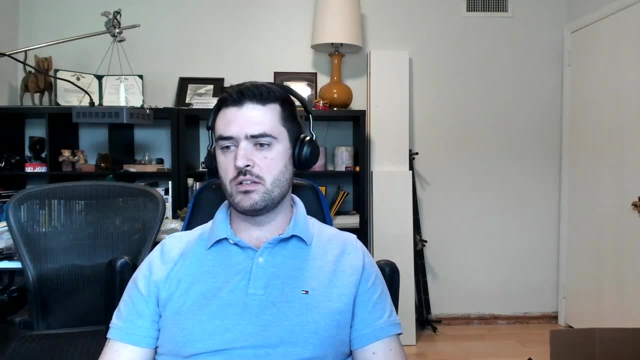 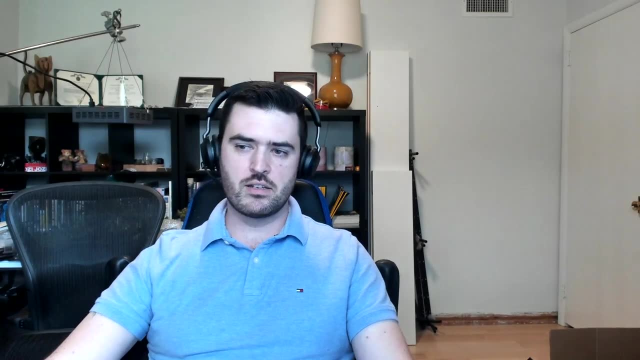 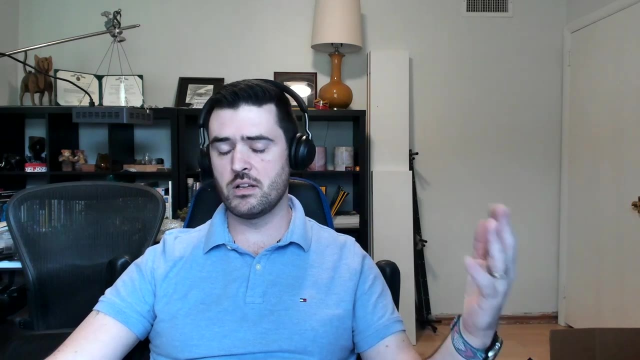 governance with artificial intelligence. yet they may find it challenging to implement some of the requirements because it requires just new knowledge, new experience and doesn't necessarily um act as just an extension off of another standard like iso 40, uh, 27001. yeah, it's interesting you say. 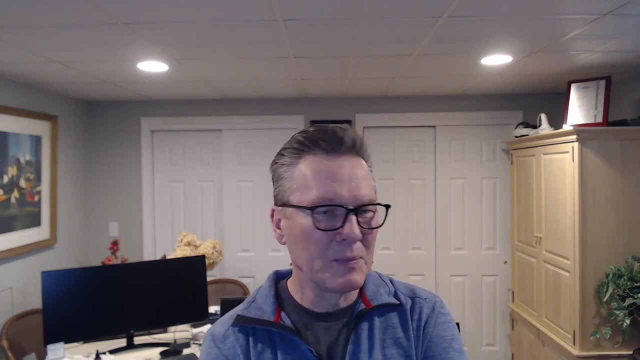 it's only 39 controls. i was a little surprised at first when i thought about that, but in and of itself the clauses, you know, contain quote-unquote controls themselves. they are controls and there are multiple controls within each clause. effectively, so you know, i think, if you kind 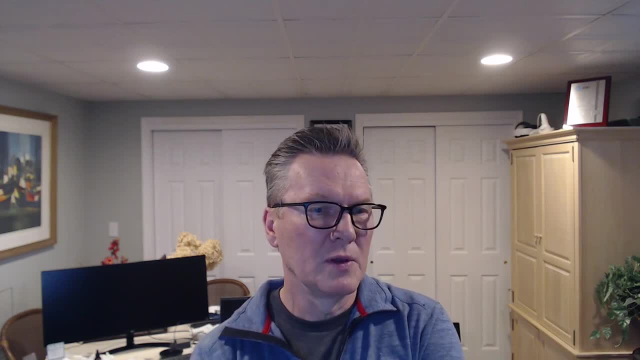 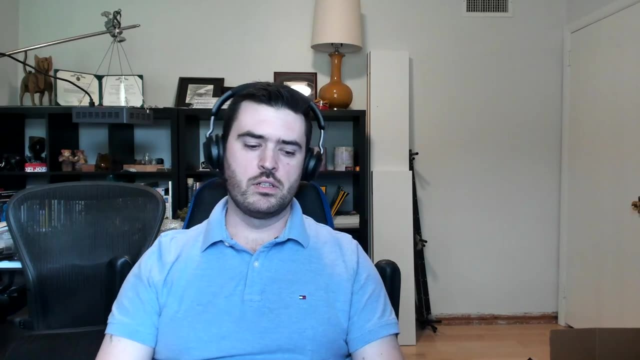 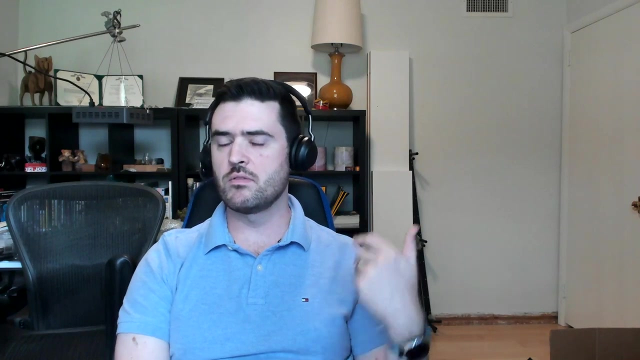 of looked at the sum total, it's probably you know twice that or so you know of things that, uh, prescriptive forms of guidance that it suggests that you consider and potentially absolutely, um, there's, you know, elements within each of those clauses that says you have to do these specific things. and then, of course, there's some language that says like you said. 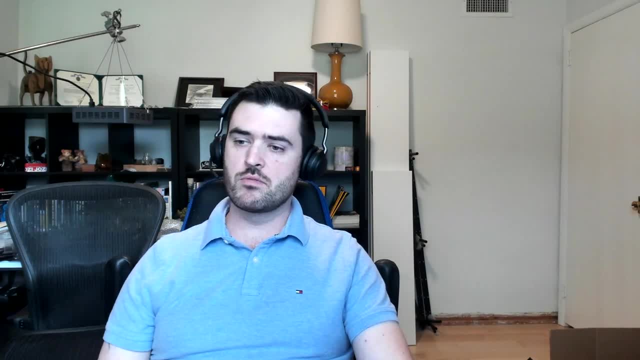 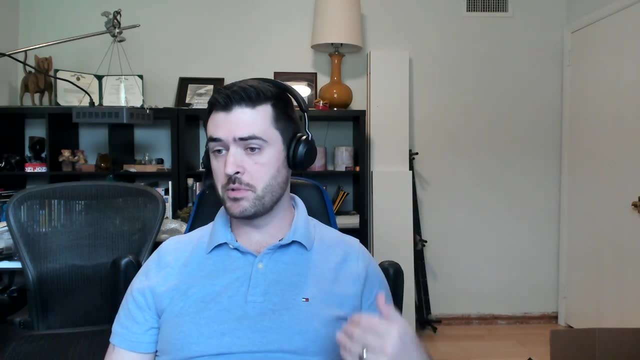 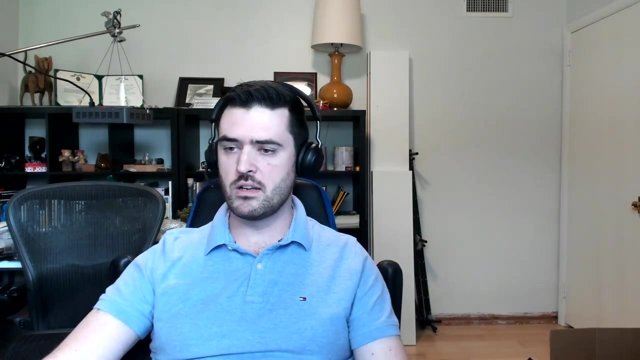 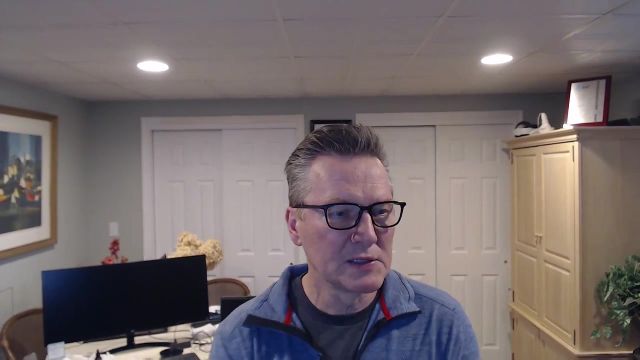 consider this, or you should do this. and one thing that's really nice about this standard is that it comes with implementation guidance and some informative annexes, so that you're not just left with these requirements and no guidance on how to actually implement them and comply. yeah, so one of the things that i was excited to see, uh, when 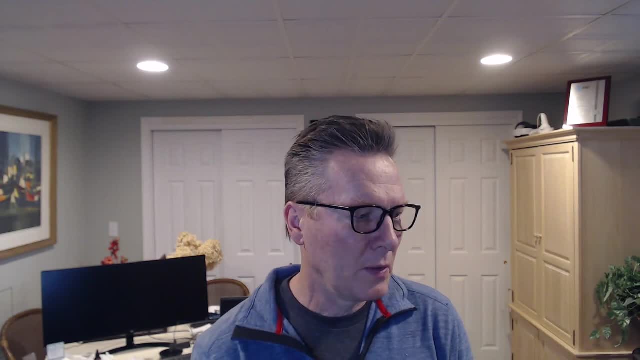 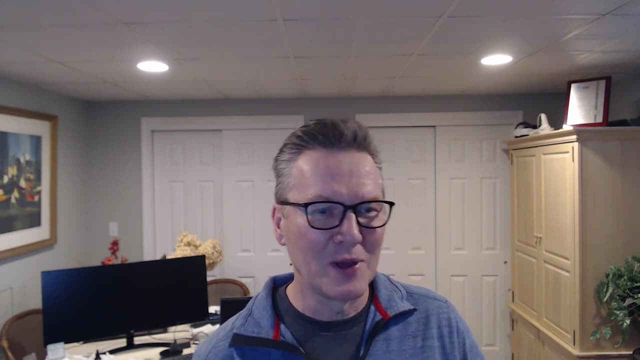 i first read the standard: uh, is that in much the same way that iso has been doing, the international standards organization has been doing for a while, actually the international organization on standards. i don't know why it's iso. it's that ios. let's, let's not delve into that right now, um, but 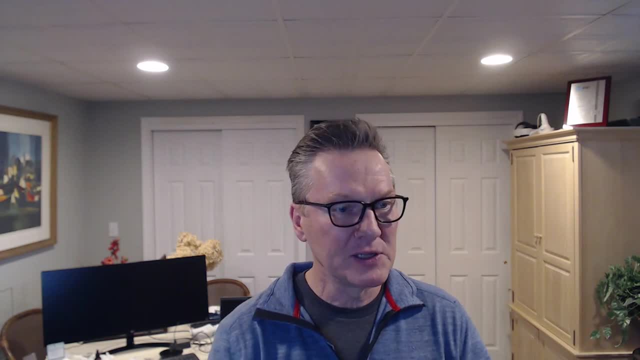 you know, i like the fact that they've maintained a consistent management system approach right. so clause four through ten has now been standardized across many of the iso standards, like iso 9001 and iso 27000, iso 26.. 7.1 and now iso 42 thousand. 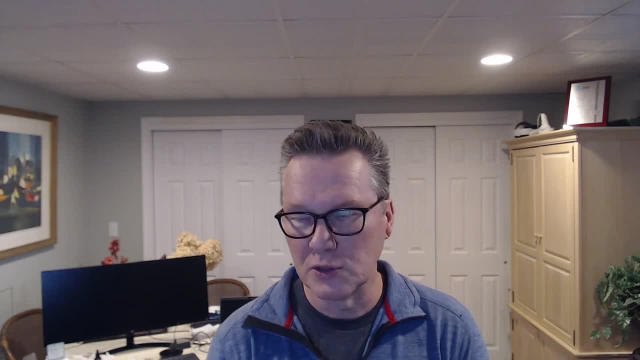 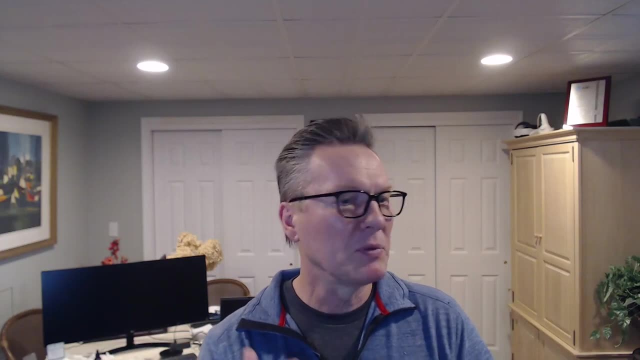 um, so you know you mentioned clause 4 through 10, those seven clauses. can we just touch on them briefly? maybe we'll walk through each of them. i'll throw one out and can you just give us a couple sentences on like what that component is, what that, what that involves, because i think 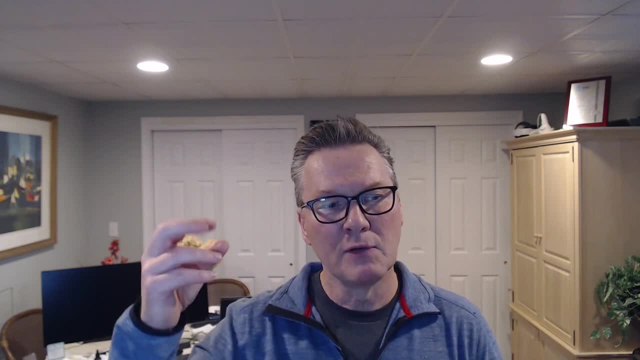 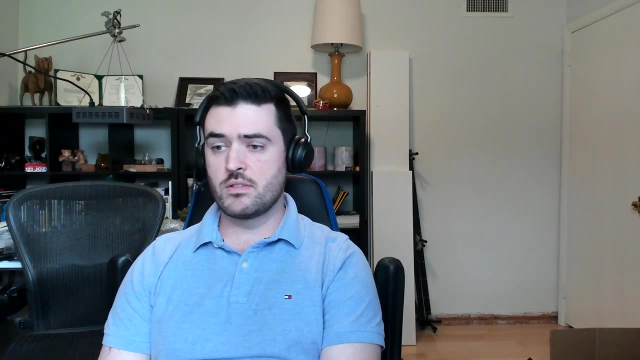 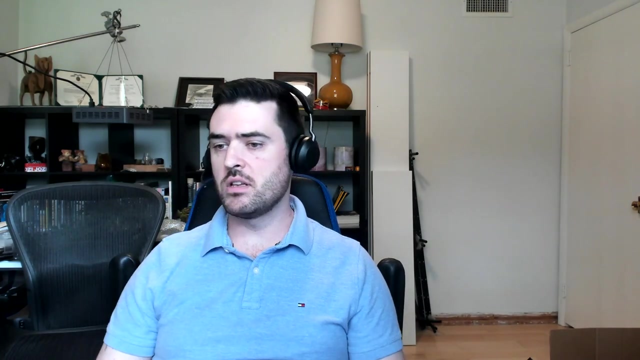 it'll give people a decent idea of what iso 42001 really is. uh. so let's start with, uh, the clause context of the organization. this i know. i will talk about most of these as they apply to 27001 and 42001, and then, of course, i'll make call outs that are specific to 42001. so this one. 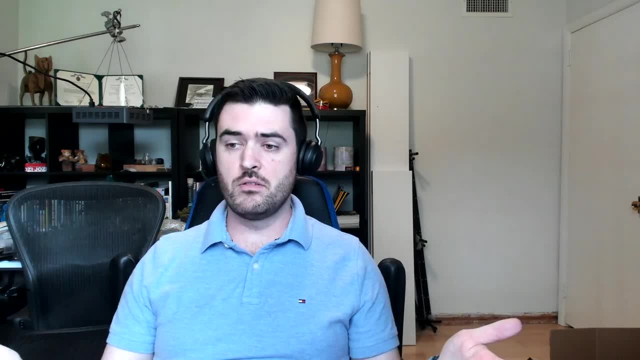 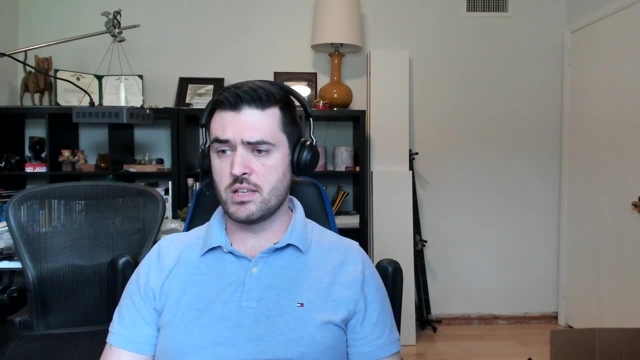 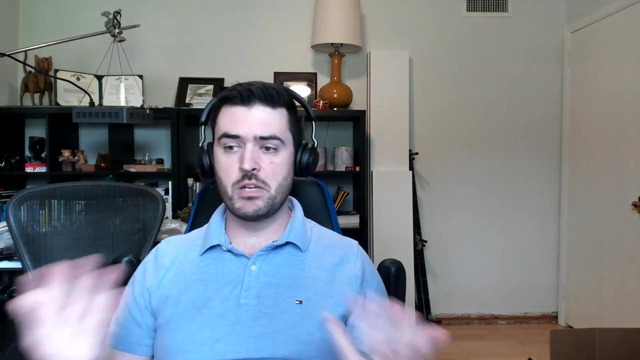 is. it's pretty much equal for both. you have to understand the context, like within information security. why does information security matter, or ai matter, to your organization? well, it could be. there are specific internal and external requirements. um, it may be that you're developing a product that you need to secure or that you need to leverage ai, uh, in order to use um and it. 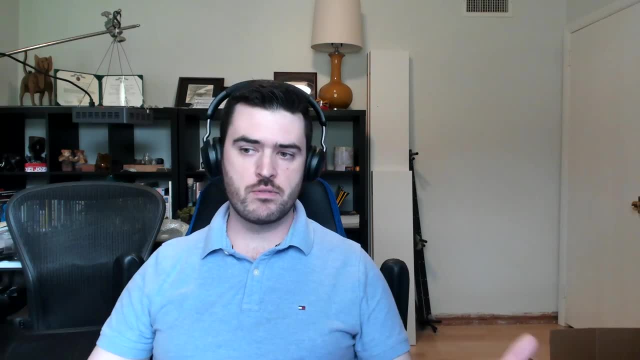 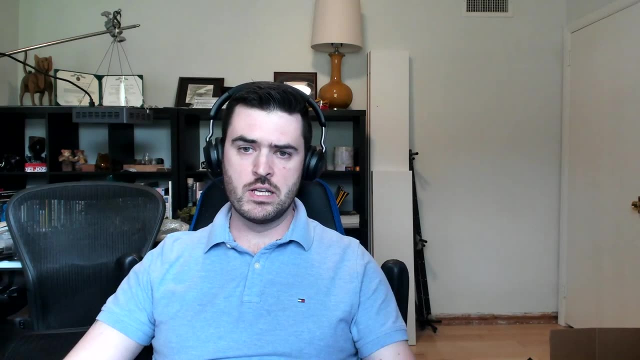 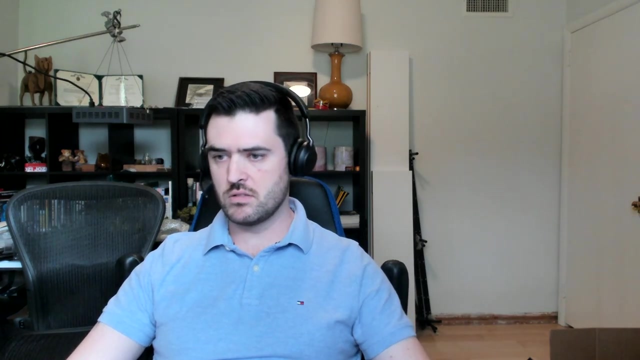 helps establish really the scope and the boundaries of the management system, both for information security on the 27001 side and ai with 42001 um. so, yeah, this is really all about scope in the management system, the internal and external stakeholders and what are their requirements. 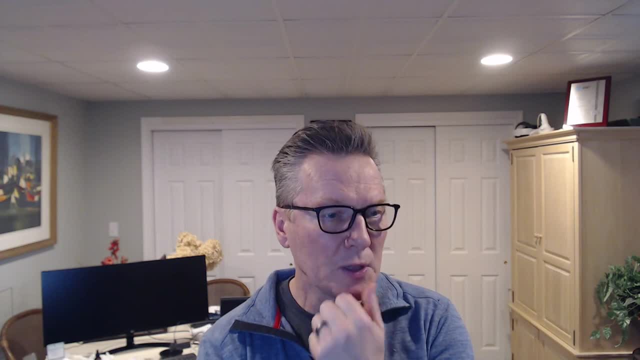 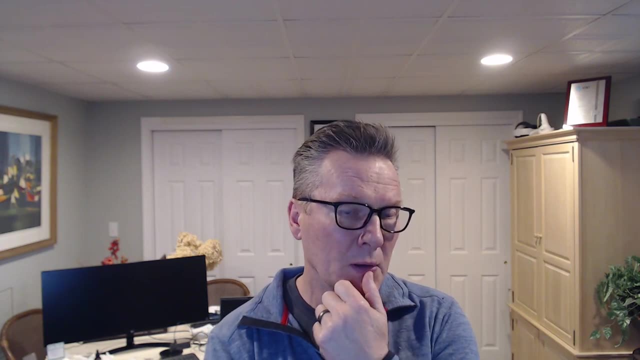 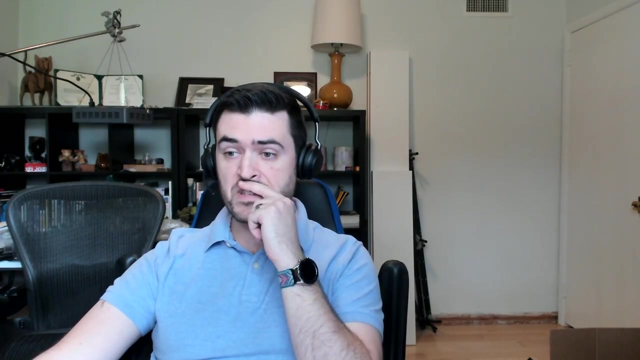 um, um, Yeah, increasingly- like we've already seen it with one of our customers- become a contractual obligation, and now we're going to see it become a regulatory, uh, a compliance requirement, right, uh, regulatory compliance, like with the eu exactly, and you may have uh suppliers that you may get a questionnaire from a supplier that you have had for a long time, and they may be. 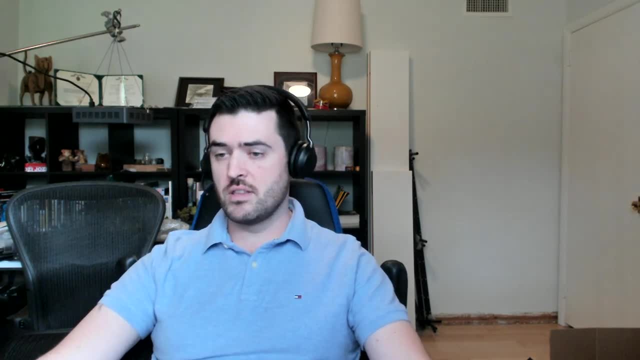 asking you: um, do you use artificial intelligence? and you may be somewhat blindsided by these things, but, um, if you were to get that, that would be something that you would be able to do, something that you would want to document as an external requirement is that your suppliers? 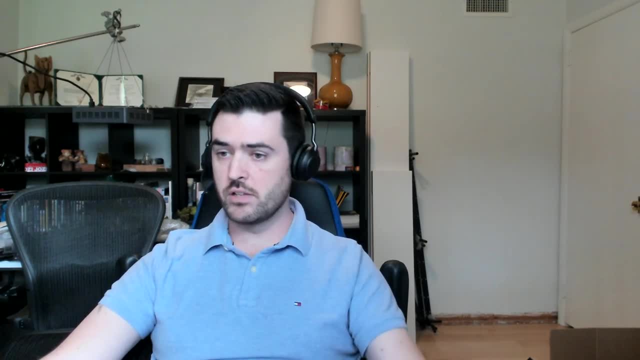 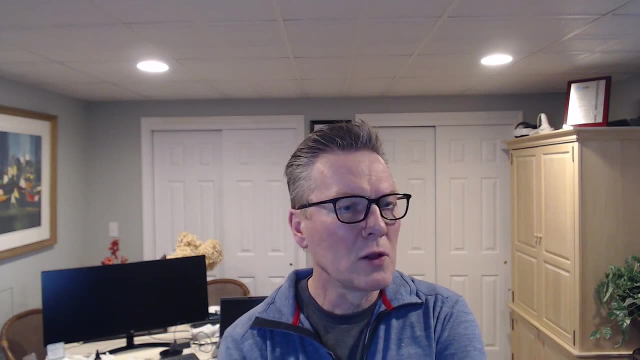 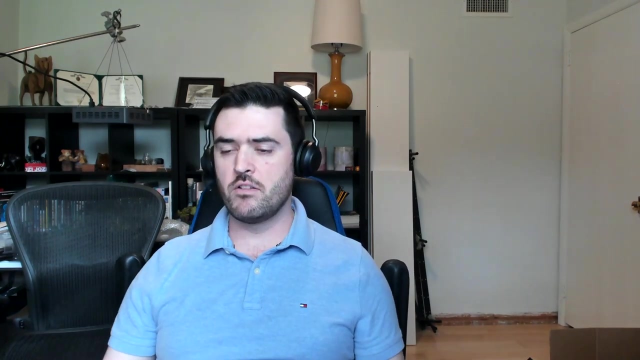 um, or your customers or your regulating bodies have these requirements for information security or artificial intelligence? yeah, class five is around. leadership: what does that entail? you can establish a management system. how is it going to be managed? you need to have leadership, involvement and commitment. um, in a strong tone from the top in order for the management system. 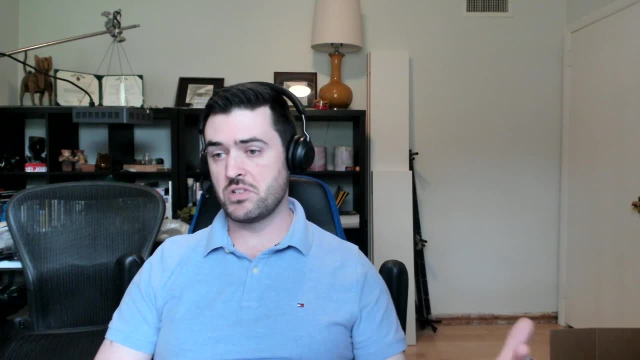 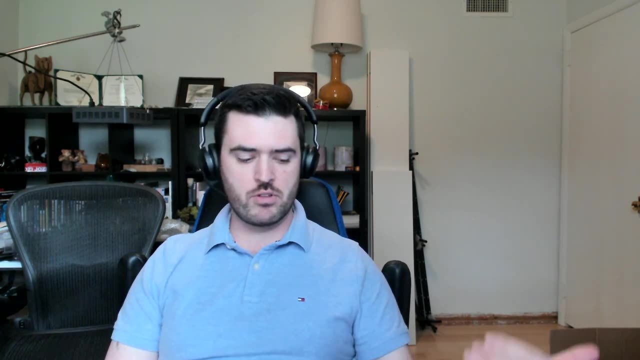 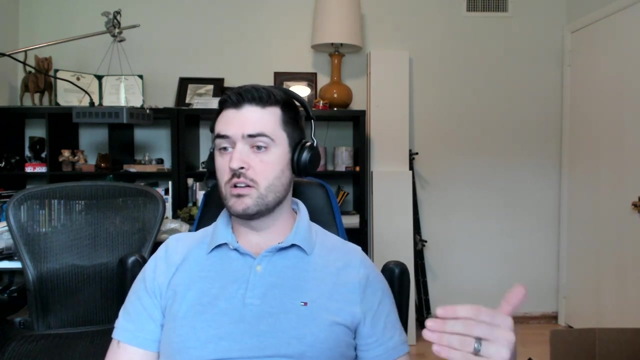 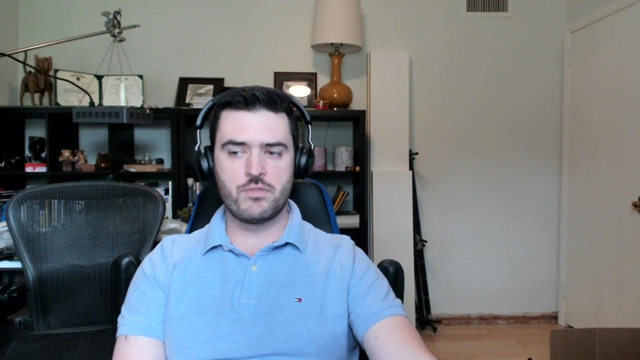 to be effective, to have effective governance of information security and all of these things um you and artificial intelligence, effective risk management, um, and so this is establishing how leadership is committed. what are they committed to? um developing, uh, an artificial intelligence policy? so this is specific to 42001- is identifying the artificial intelligence policy. 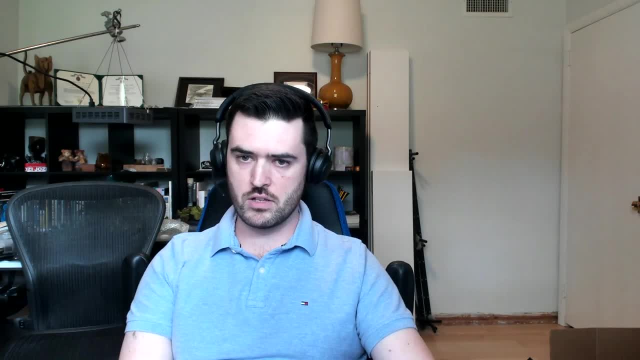 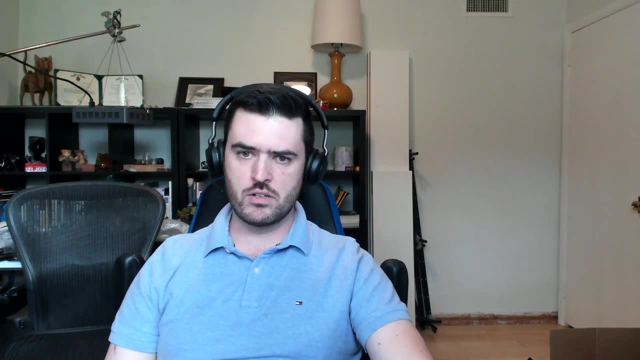 what is the organization's objectives for artificial intelligence, because this can drive a lot of the subsequent or topic specific policies unique to artificial intelligence. and then, of course, it also establishes the relevant roles and responsibilities within the organization to ensure um that the management system can achieve the objectives. 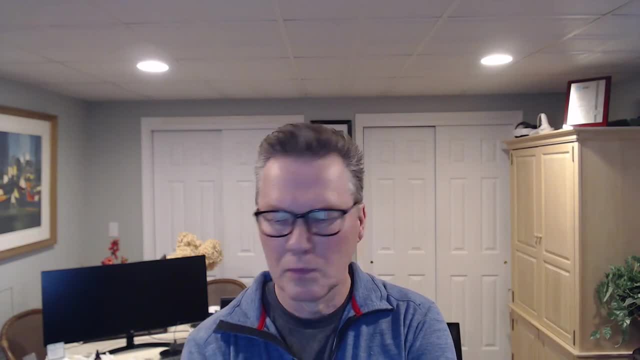 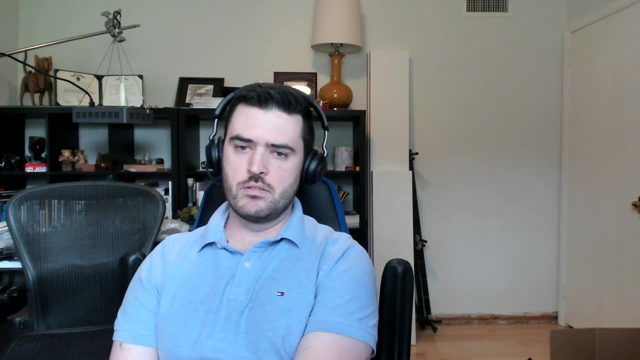 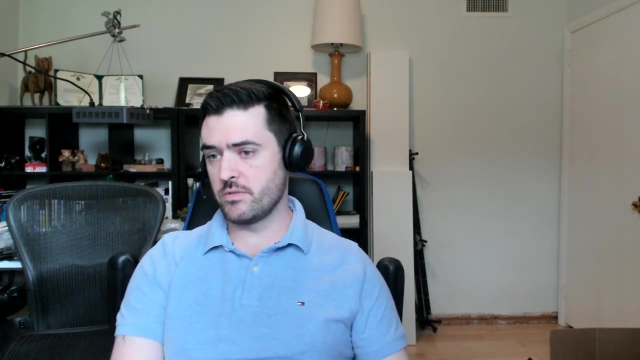 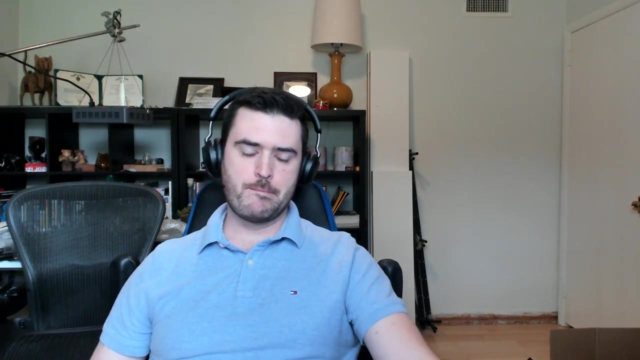 set by leadership. gotcha uh close. six is planning. this is about how can the organization uh assess artificial intelligence risk and treat that risk um, and so this is establishing the processes for doing that. what are the criteria with which organization needs to um, you know, assess and treat that risk um? there's an additional component here. 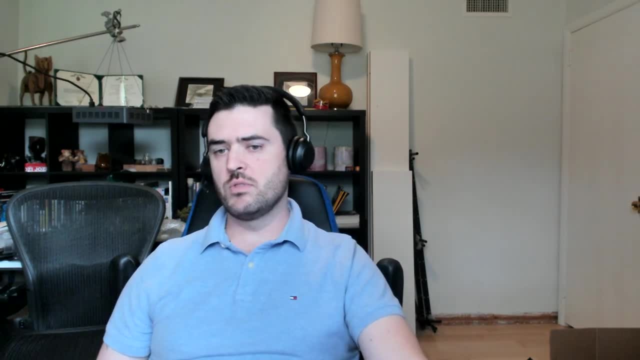 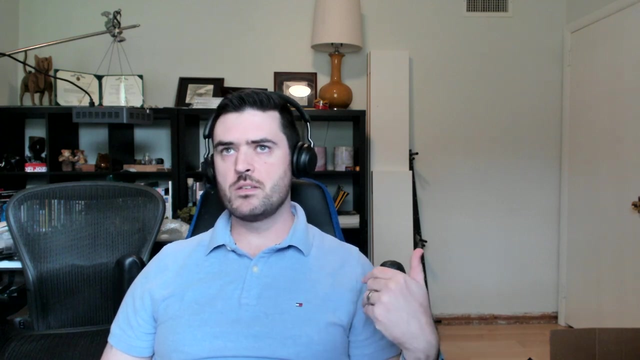 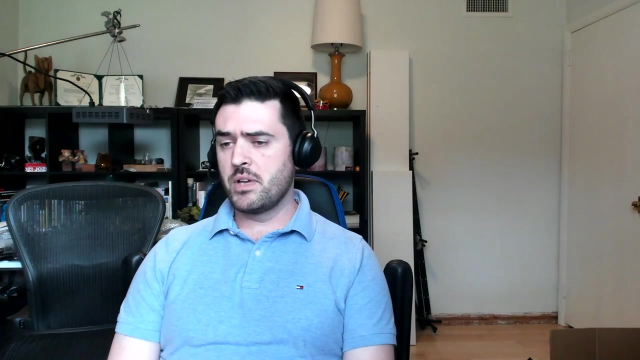 that is not seen in iso 27001 and that has to do with an artificial intelligence impact assessment as well as establishing artificial intelligence objectives. so the ai impact assessment may be something that could be um informed by iso 27 701. so organizations a lot of times implement a privacy impact assessment. 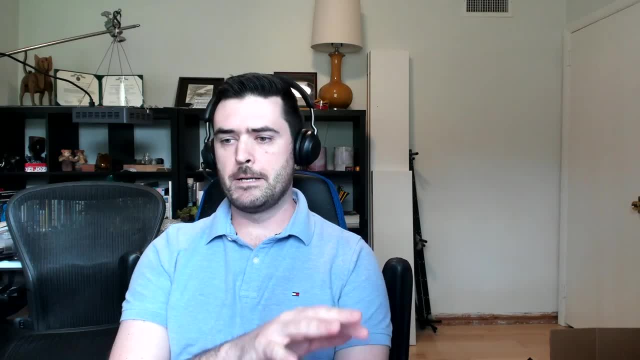 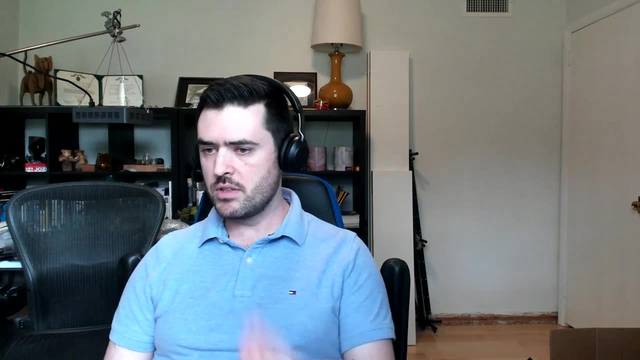 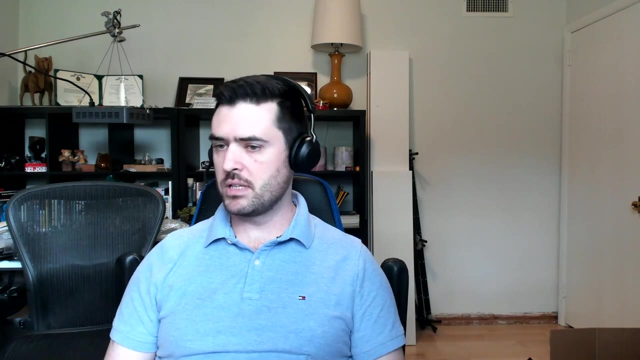 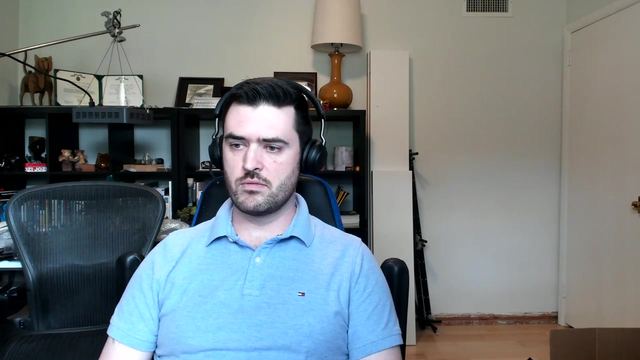 to understand specific risk unique to um, privacy, pii, personal data. so that is a similar approach here with artificial intelligence. how are these systems going to impact individuals, groups of individuals or society? you know it depends on the application of the artificial intelligence system, um, but this is something that is new here is making sure you have a risk assessment, a risk treatment plan. 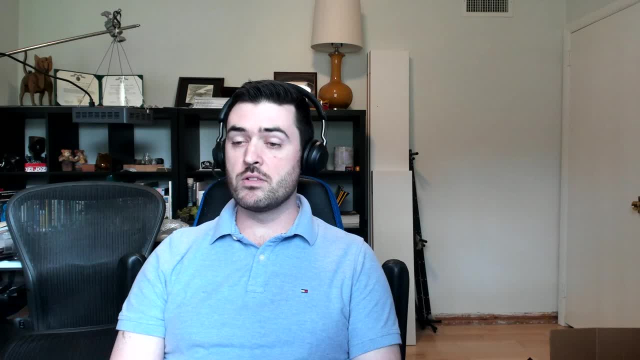 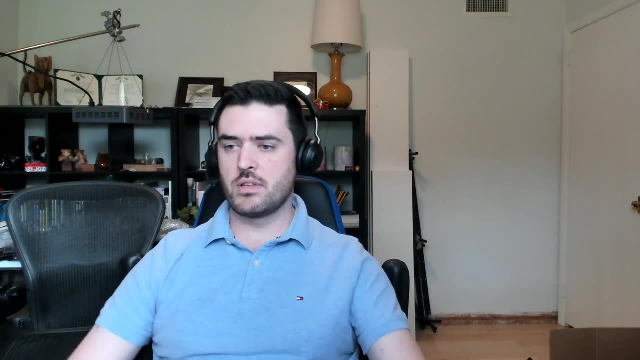 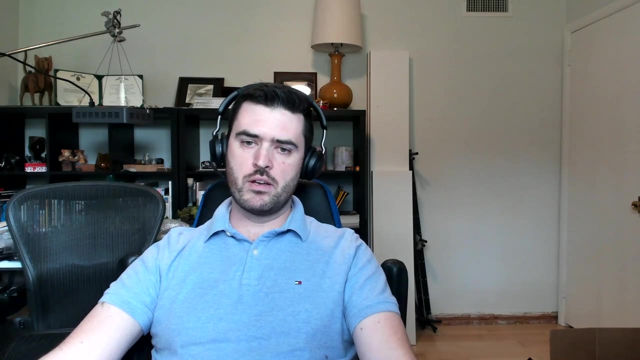 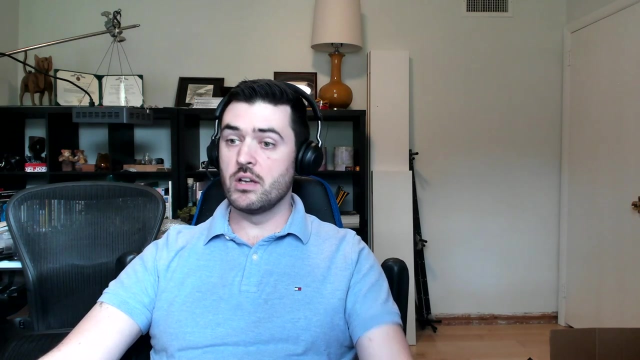 for artificial intelligence within the organization, but also that you conduct specific AI impact assessments and those can be used to inform your risk assessments Support. So this is important because it helps the organization establish you know what are the resources that are required in order for you to achieve your artificial intelligence objectives. 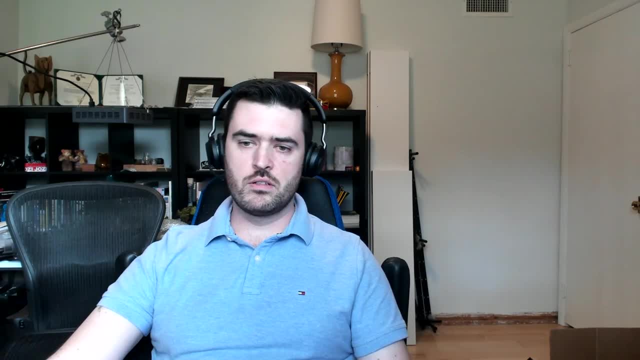 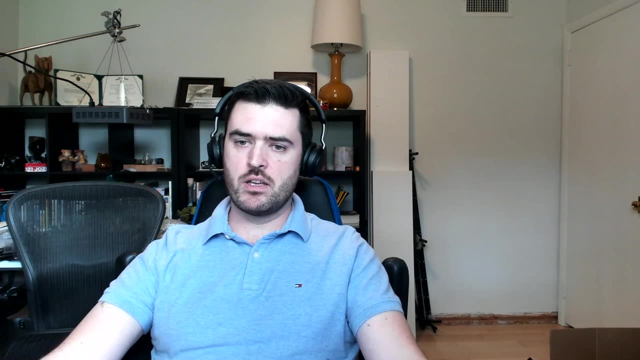 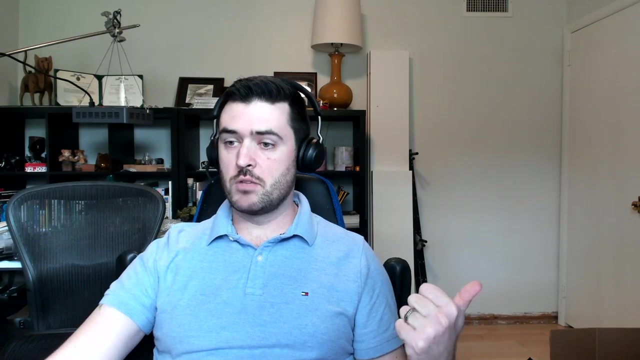 for the management system. So establishing the human and capital resources system, resources, things of that nature- and then also ensuring that you have the right people, the right knowledge, the right assistance to develop the management system, maintain the management system, and then making sure that you effectively communicate. 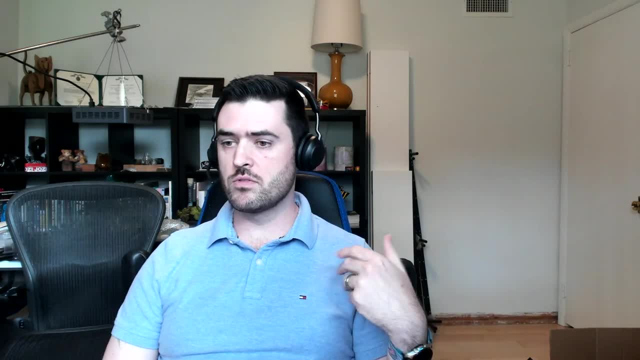 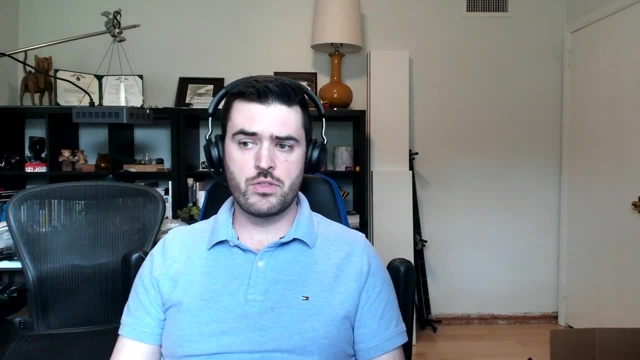 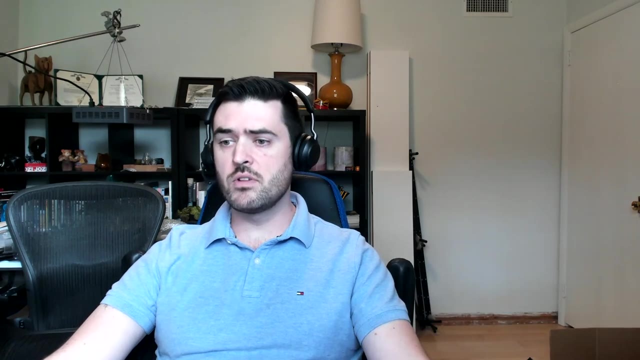 the management system, The implementation and maintenance of the management system, so that all of those roles and responsibilities that were identified in the earlier clause, that all of those people understand what their responsibilities are and what their roles are. So, effective communication of that, effective communication of policies relevant to the management system. And then 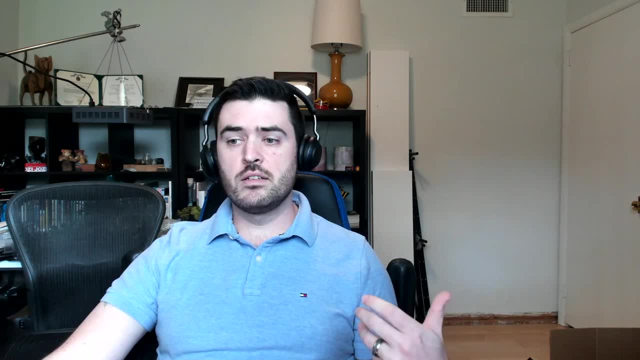 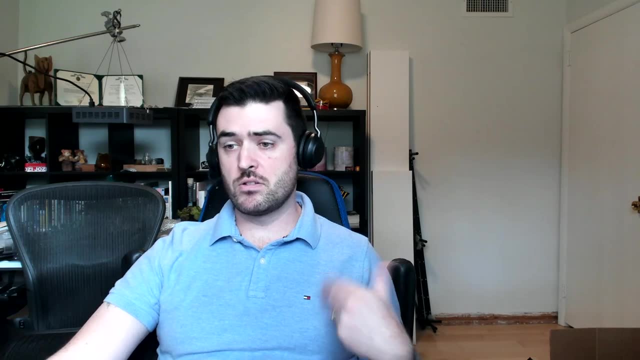 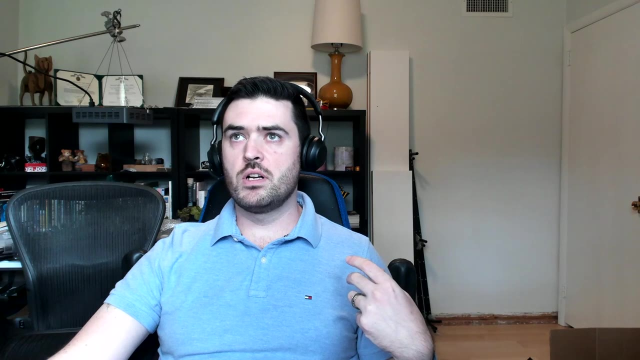 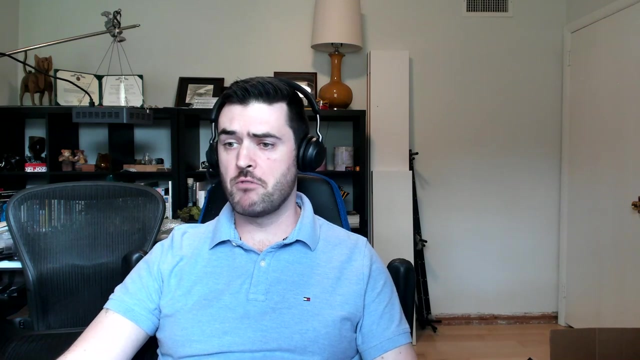 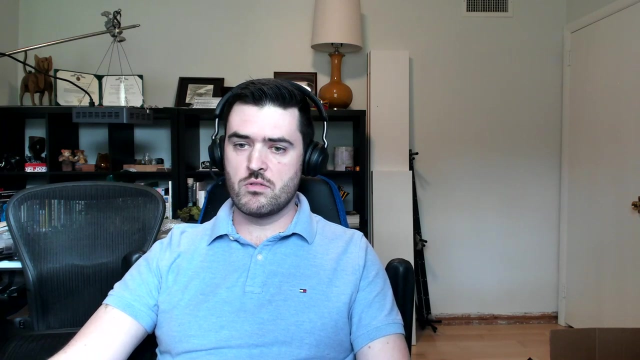 of course, recording and maintaining any documentation, both required by the standard, but also required by the organization in order to implement Ensure they're compliant with this standard. So something that may not necessarily be required by the standard is you measuring how many users interact with your AI application every day? Standard doesn't specifically require that, but it does require that you maintain metrics and that you monitor the AI system, And so, in order to do that, you would then have required documentation because the organization chose that specific metric. 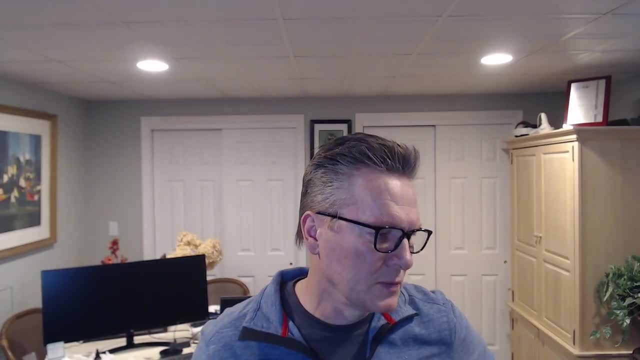 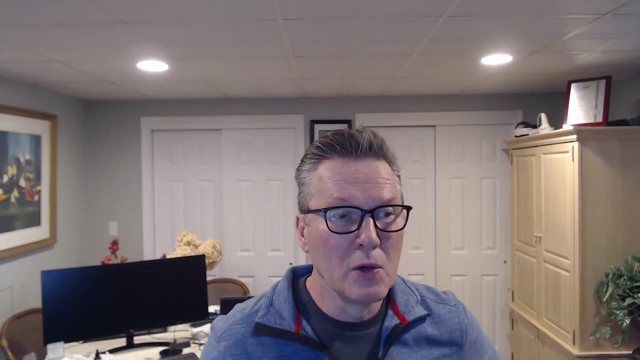 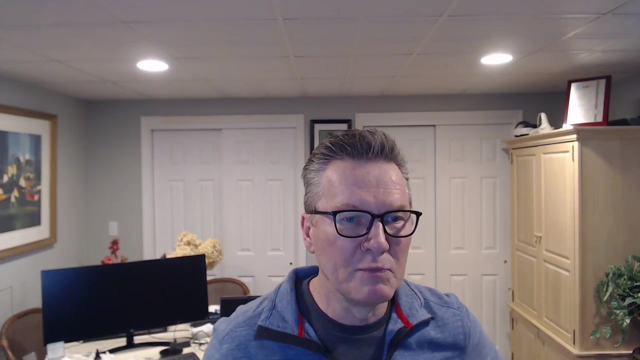 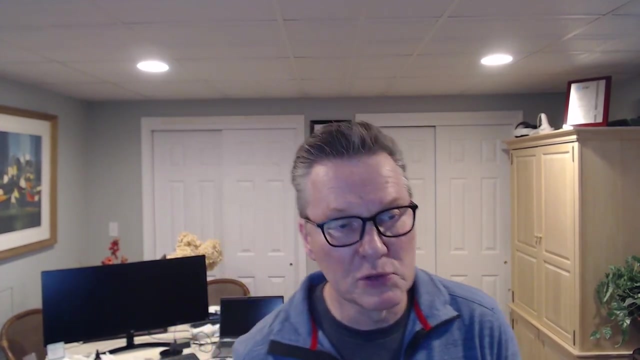 Yeah, And under seven they cover. what I think is critical around AI is awareness right, Because if everyone isn't aware, like you said, we can encumber somebody. can you know, procure a new SaaS application that's making some type of business decision on our behalf, And if they're not aware of the implications and what our acceptable use of said applications is, what processes they need to go through? 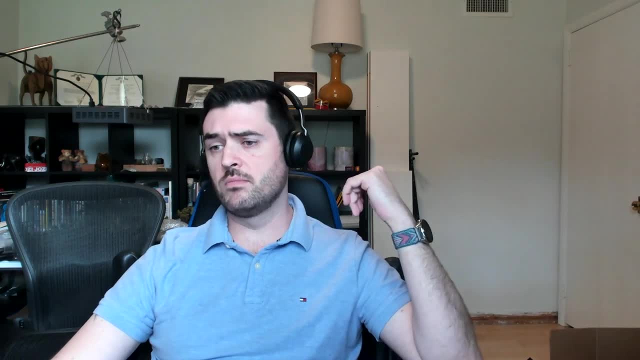 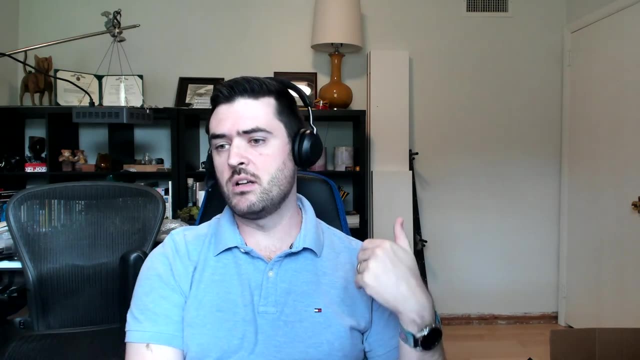 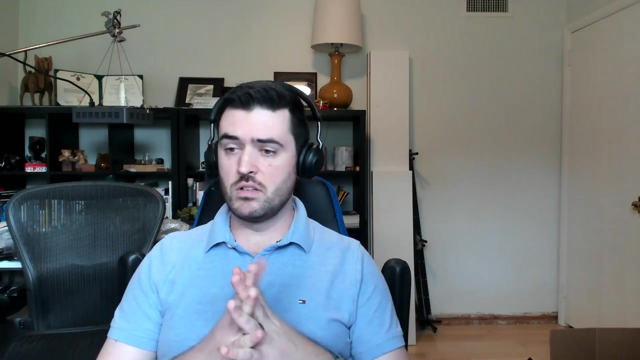 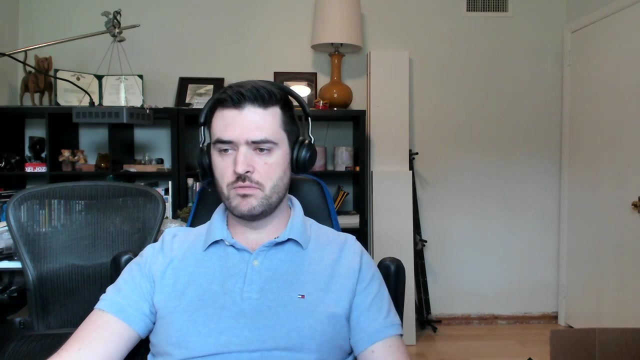 Exactly, And those roles and responsibilities Exactly. And those roles and responsibilities can span from top management all the way down to end users. It can spread to customers, external users of the artificial intelligence systems, developers and engineers- just a variety of people internal and external towards the organization, And if those are not communicated effectively, then the management system is going to falter. 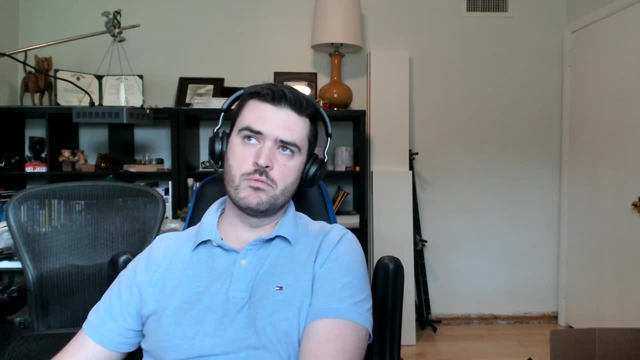 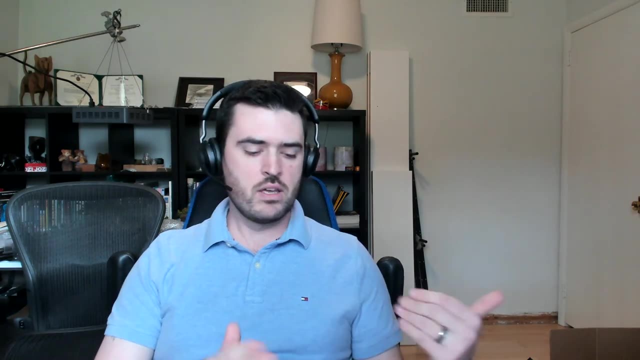 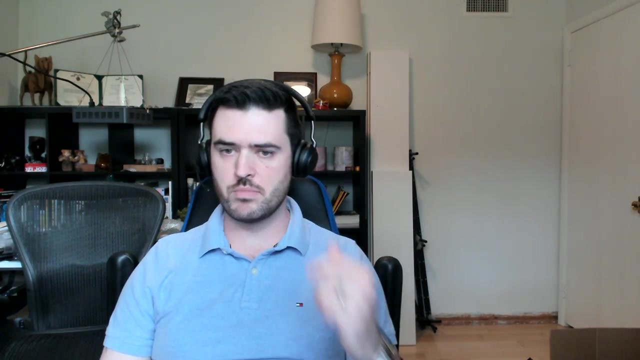 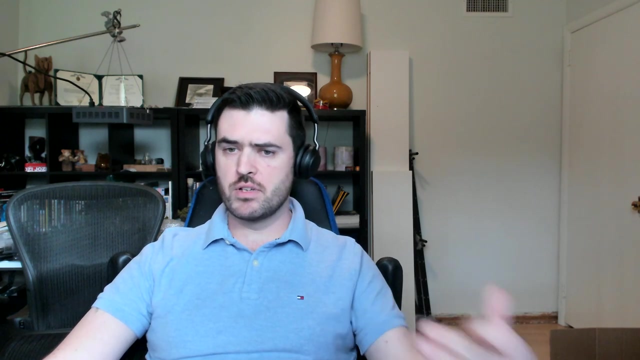 So this one is: how is the organization applying the items that we described under the planning phase right? So, is the organization conducting their AI risk assessments and treating AI risk based on the methodology that was established in the planning phase? Is the organization conducting the AI impact assessments? Is risk being effectively treated? And then, of course, 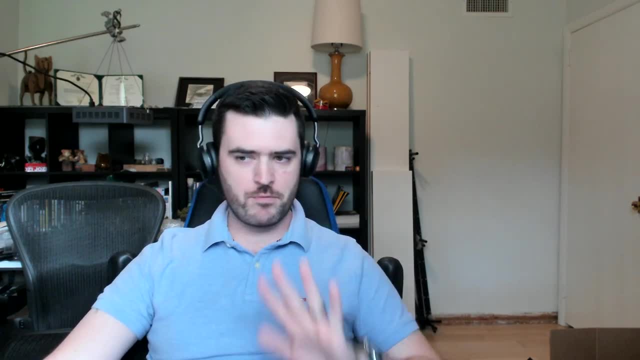 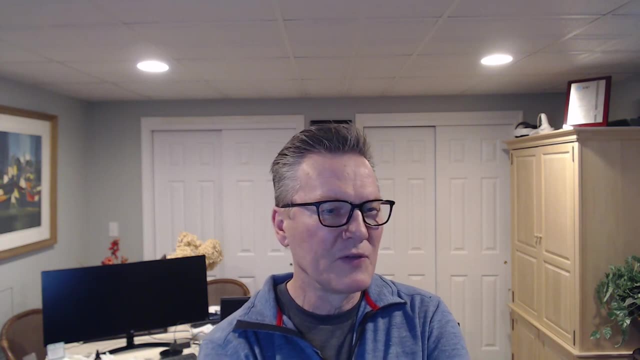 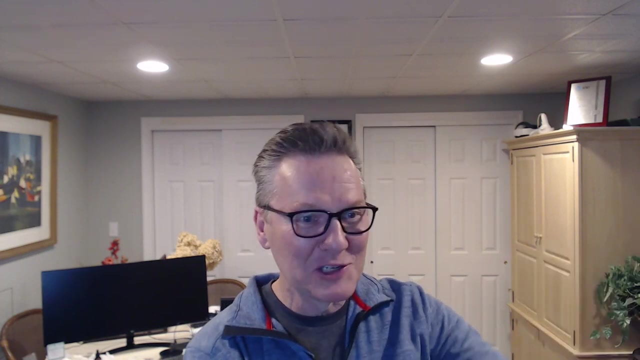 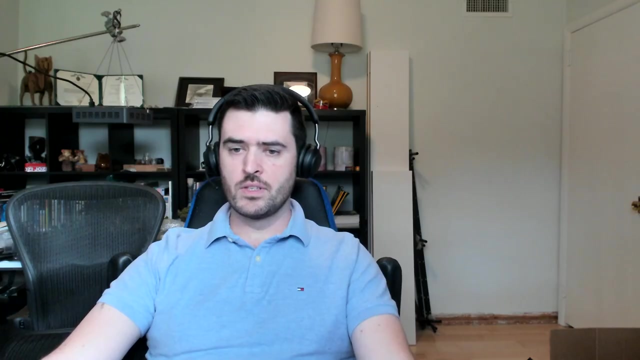 there's always a measure of continuous improvement, but I'll kind of hold off on that until we get to the last clause. Yeah, and if you think about it this, if you remember the old early days of ISO, we used to call it: plan, do, check, act. Yeah, so you talked about planning operations of the do, and now we're about to go into check and act, right. So the next one, clause nine, is around performance evaluation. 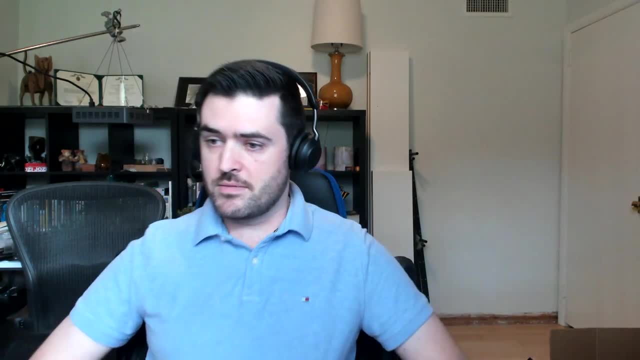 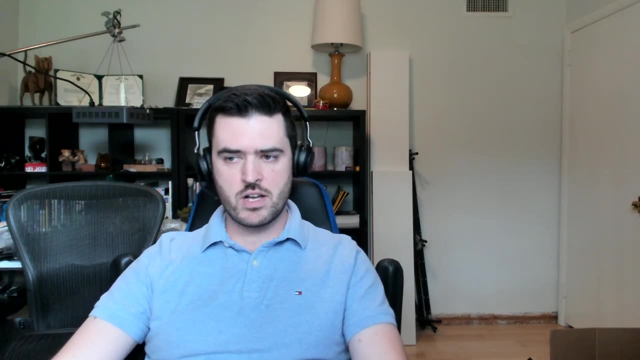 Yeah, so how do you know that your management system is performing As intended? right? What are your objectives that you established in the previous clause, And are you meeting those objectives? In order to do that, you need to monitor specific metrics that map to those objectives, And then you need to evaluate those measurements and then make sure that you're communicating those measurements of effectiveness to top management so that they can adjust the management system as needed to make sure that you're meeting those objectives. 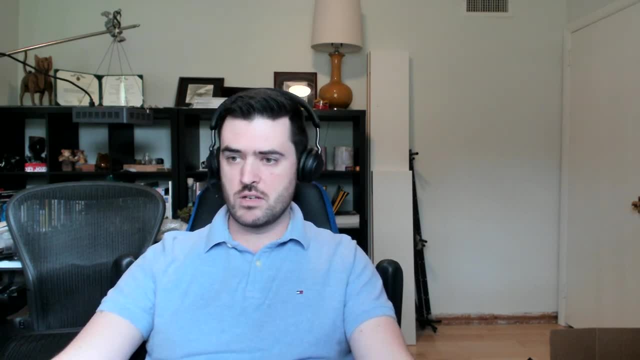 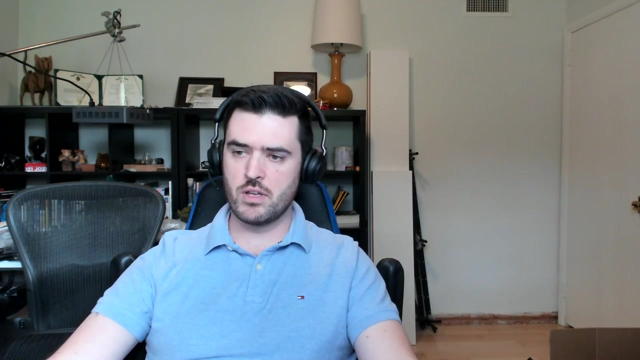 Yeah, They're achieving those objectives, or maybe changing the objectives or changing the metrics themselves. And then it also establishes requirements for making sure the organization has an internal audit program, And that's part of that monitoring and measurement requirement. You can have metrics, but you also need to have an independent internal audit of the management system and the methods used to maintain that management system. And then the final, 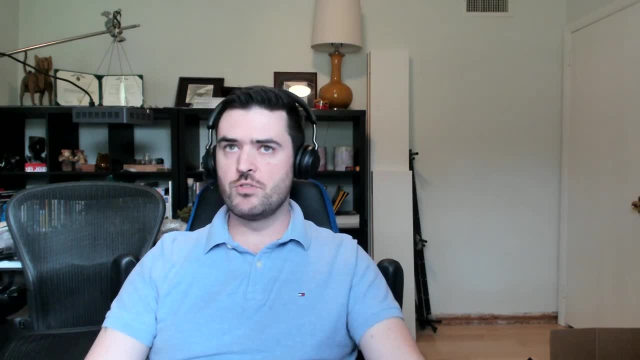 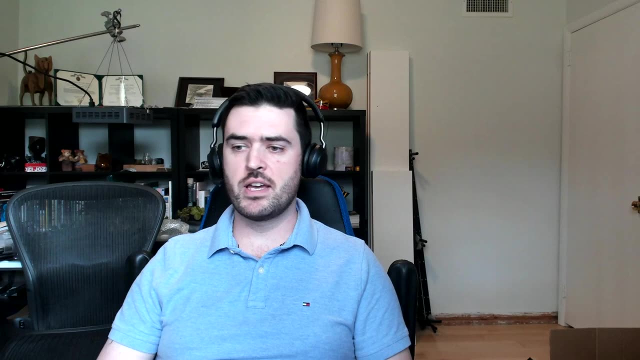 Yeah, the final piece of that is that management needs to review, There needs to be a management review of the management system on a regular basis, And so they'll review things like audit findings, results of a risk assessment, any internal or external changes that might affect the management system, And then, of course, just input, and that that management review should be conducted by a committee of top management that includes relevant stakeholders. So for artificial intelligence managementеры. 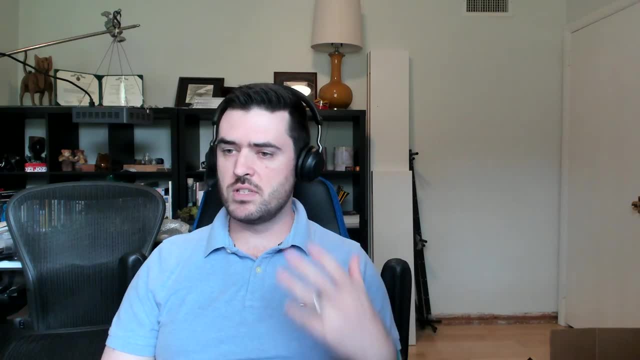 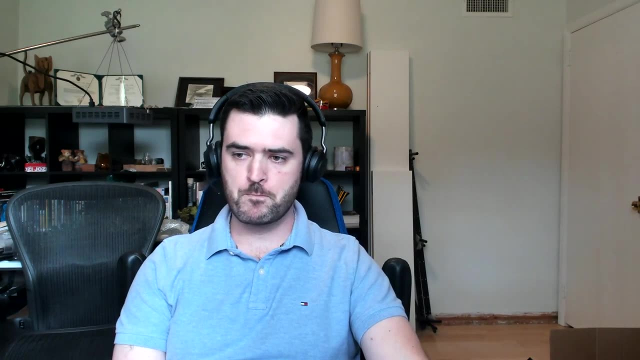 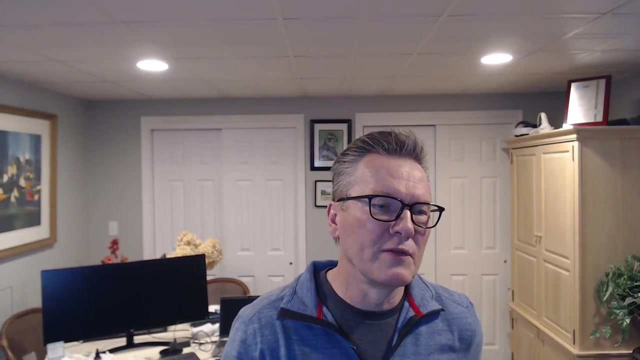 This could be your CISO, it could be your CIO, your CTO. business stakeholders, artificial intelligence experts, for example- Yeah, your developers. I mean, if you are developing your own large library models, right, it's going to be the people that are the machine learning experts that have to be integral to this right. 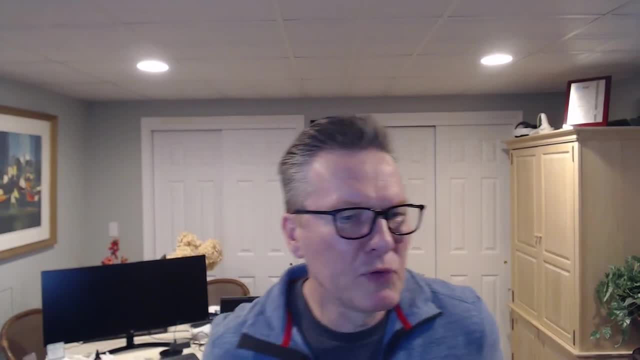 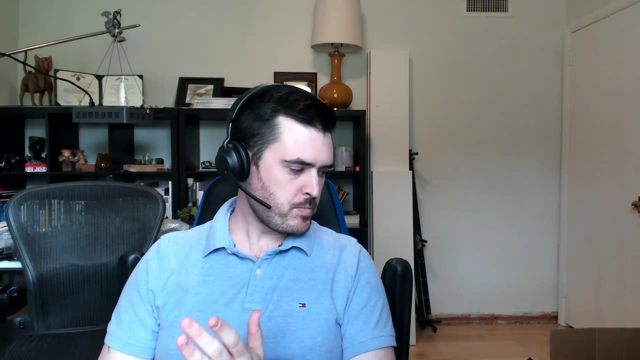 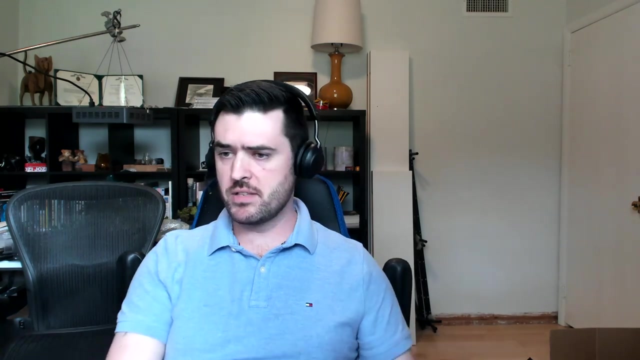 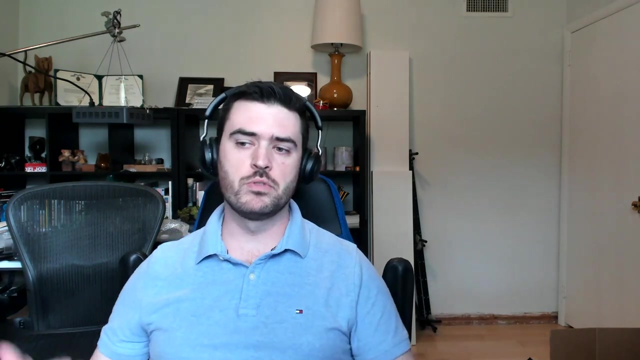 Yeah, And then, last but not least. So this one ISO has a strong approach for continuous improvement, right? This isn't really like a pass-fail of this standard. It's that you can implement something, identify gaps, identify the effectiveness of the management system and then just continue to improve it. 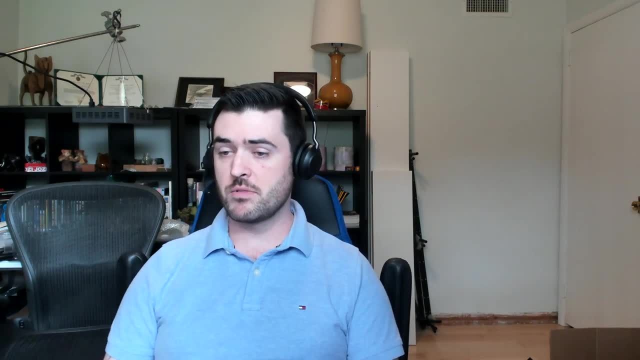 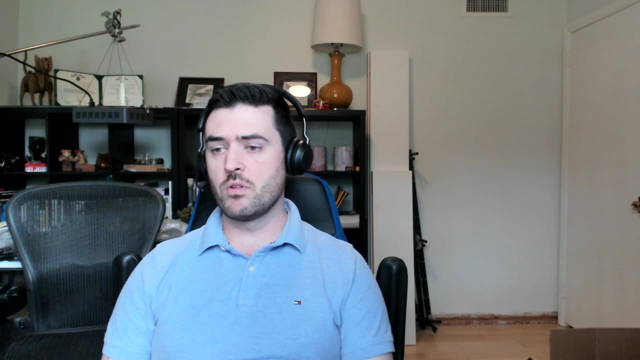 Strengthen your implementation of management clauses, strengthen your implementation of controls, And so This clause establishes requirements for the organization to do that continuous improvement. So If there are audit findings, management should review those based on the requirements of the previous clause, and then document what's being done to address those findings. 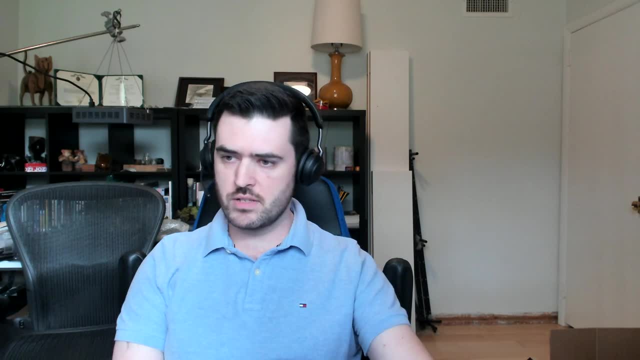 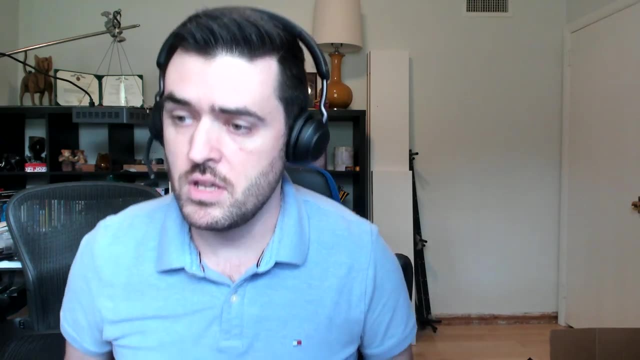 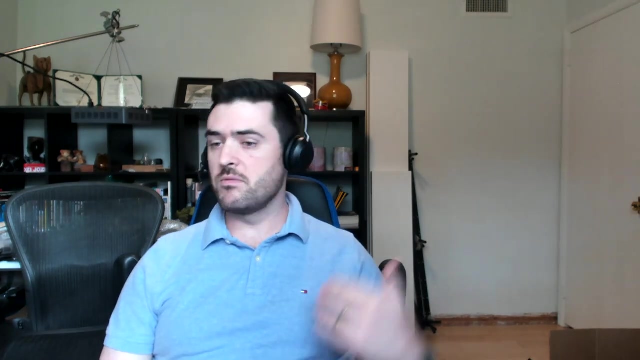 What is being done to address new risks that are identified or to potentially treat existing risks that have changed? Maybe the impact or probability has changed, or there's changes within In the organization that reduce the effectiveness of existing controls, So there needs to be. 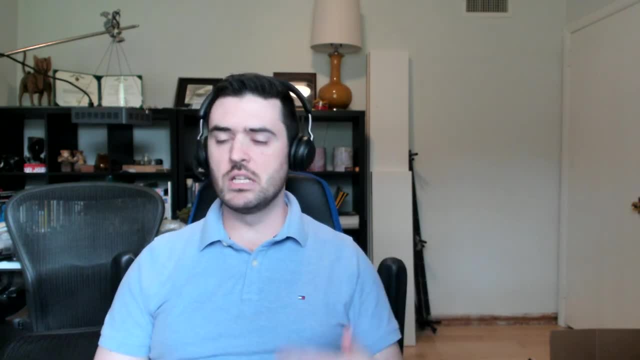 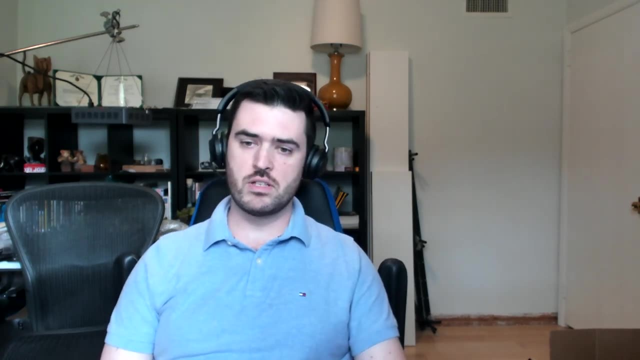 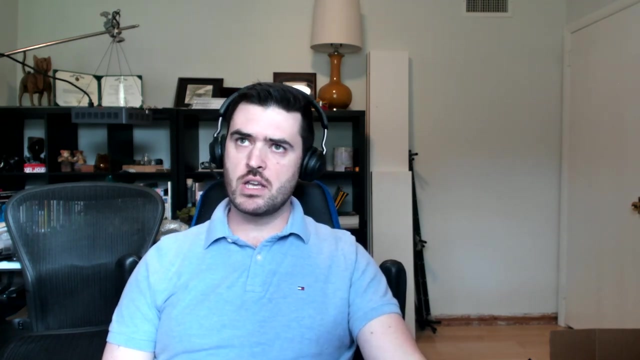 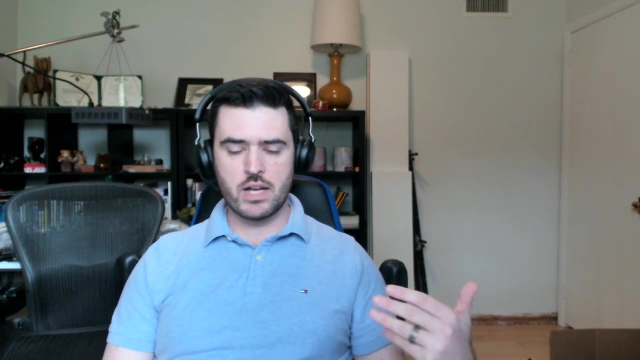 Processes put in place to ensure the organization is continuously improving the AI management system and the information security management system, as is the case in ISO 27001.. And then the second component here is that the organization understands and establishes a methodology for identifying non-conformities to the standard. 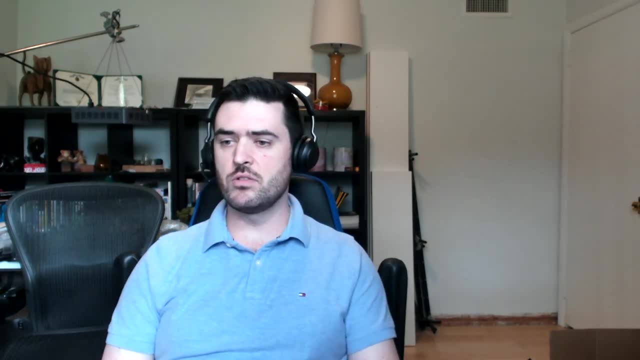 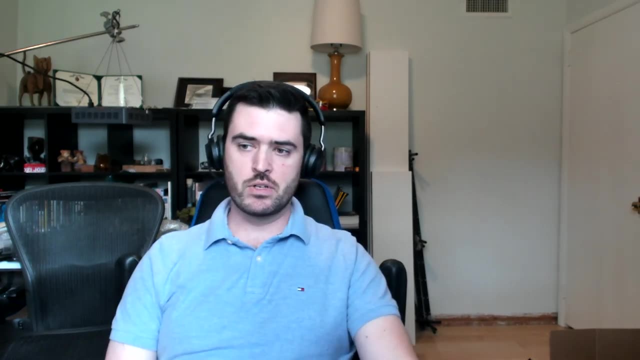 and then what actions to take in order to address those non-conformities. So this is similar to the audit findings, because that's where these non-conformities are going to pop up. But the organization needs to have a formal process for what to do when non-conformities are identified. 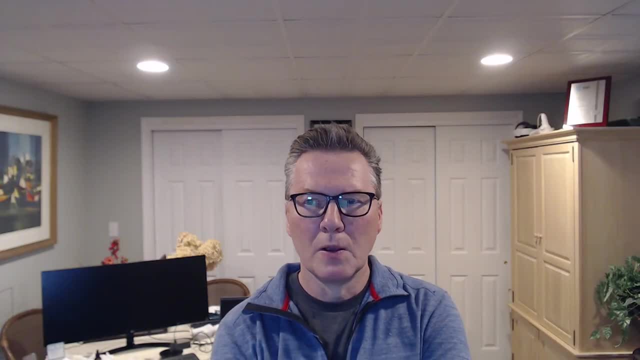 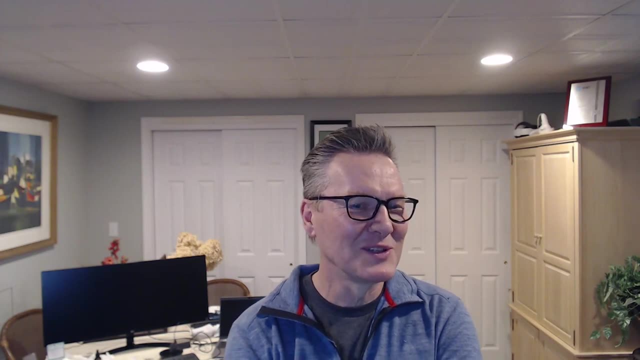 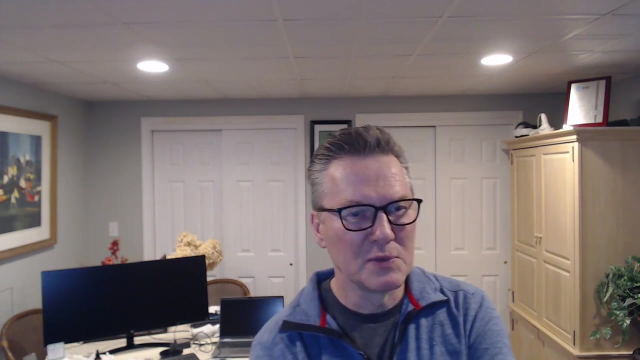 So for any of our listeners that are ISO 27001 certified, this is probably pretty comforting because it all sounds darn familiar. You know, effectively what we're just doing is replacing- you know it's now- instead of an information security management system. 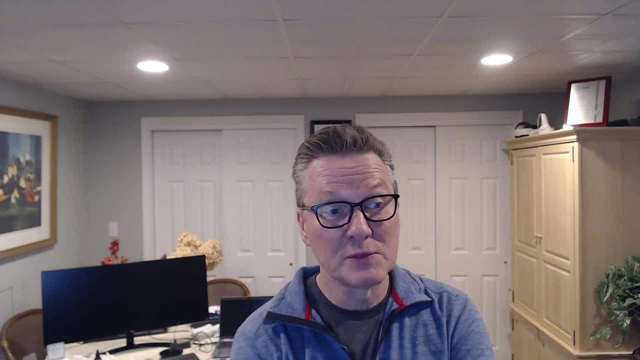 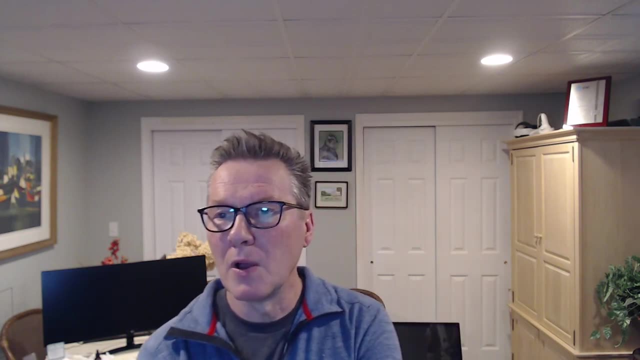 it's an artificial intelligence management system, with the vast majority of the components of it being very similar, to near identical. So you mentioned earlier that the organization needs to have a formal process, that we've got these controls. So it was interesting to me. we have Annex A- controls. 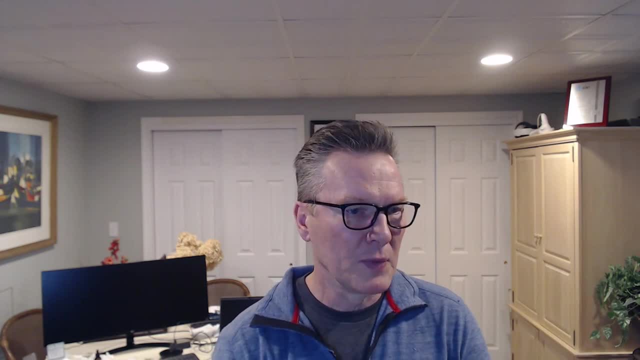 like. we have Annex A, controls in ISO 27001, you know which are, you know, like you said, 39 fairly prescriptive forms of guidance to help us understand. what does it mean right And how do we control the risk associated with AI. 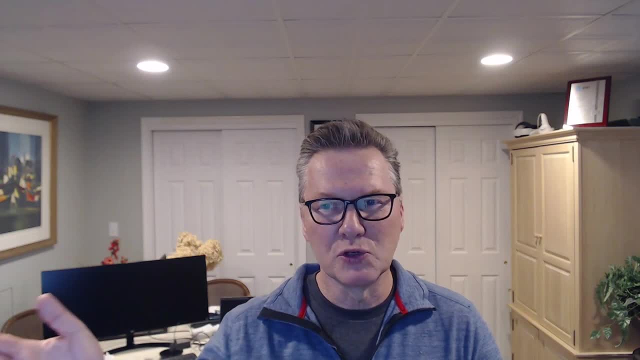 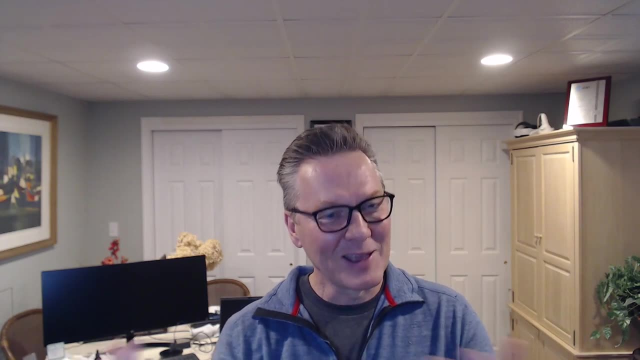 And then what I thought was interesting is that they added the Annex B which you referenced before the implementation guidance. You know, that was sort of like a shorthand version of ISO 27002, right, Like from an analog perspective. Yeah, I was pleasantly surprised. 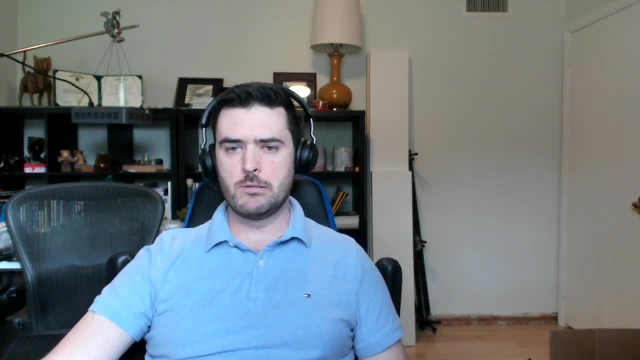 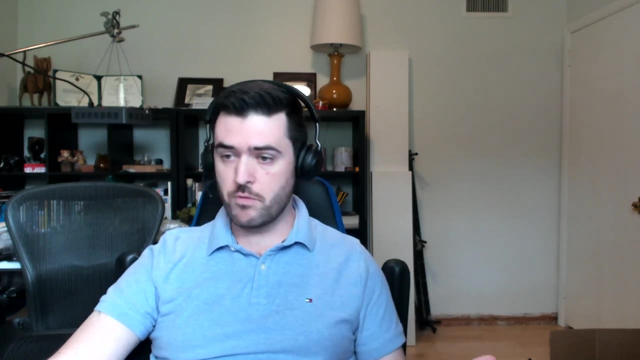 when I first read the standard, because a lot of organizations don't know that ISO 27002 is out there. Hopefully they're informed over time. but I've definitely spoken with organizations that they've implemented 27001 and just have not really leveraged the guidance from 27002.. 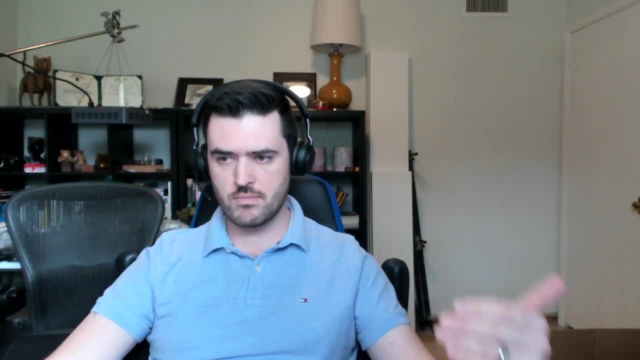 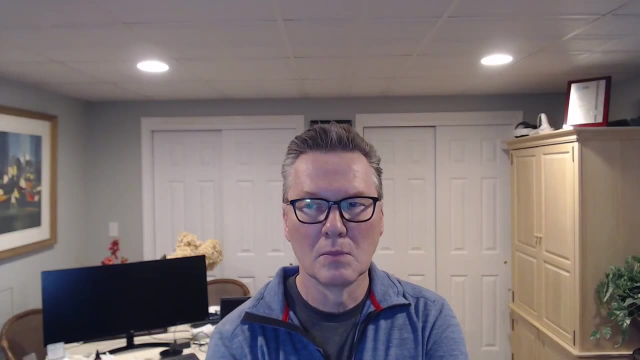 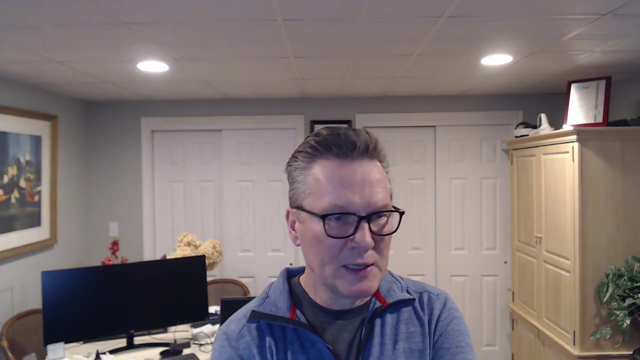 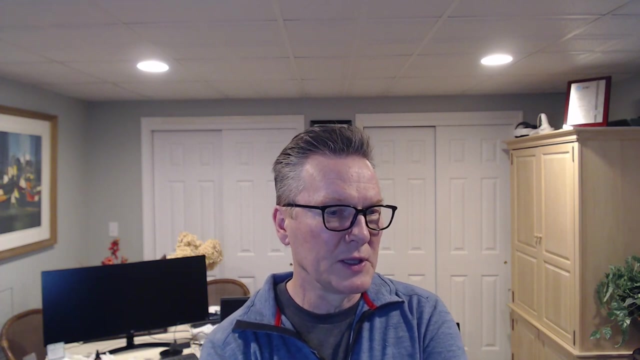 And so for ISO to include the guidance in the same document is incredibly helpful, So pleasantly surprised. So, as you know, GPT- at least based artificial intelligence- by definition, involves massive training, data sets, And increasingly, these data sets include personal information. 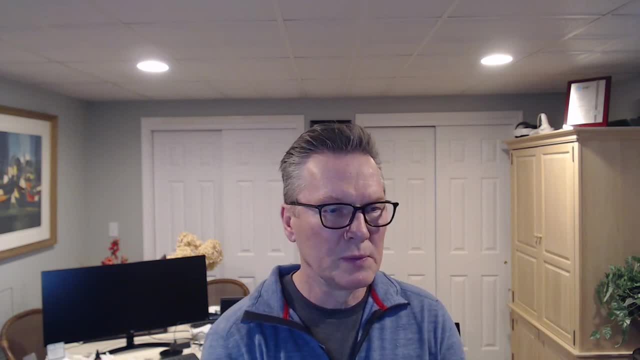 Can you talk a little bit about how ISO 27001, ISO 27002, ISO 27001, ISO 42001, in my mind, for many organizations they're ultimately going to form like sort of the holy trinity of you know? 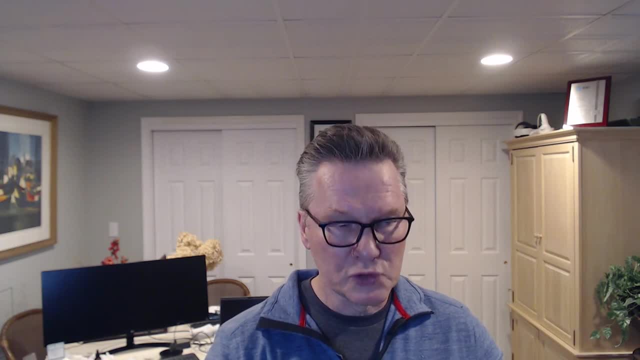 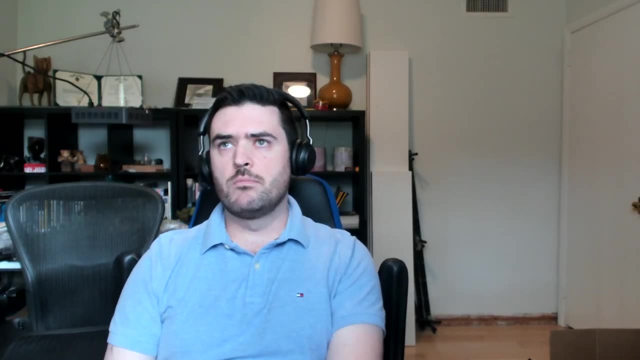 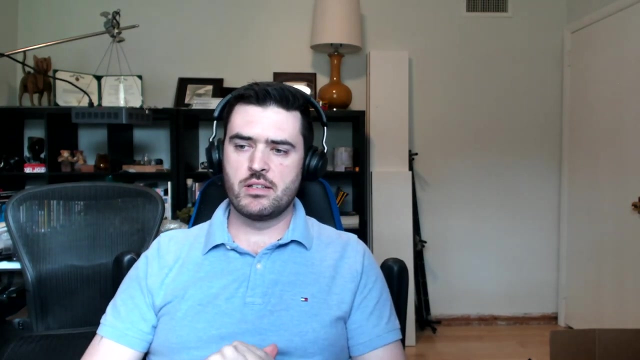 provable, demonstrable security around privacy, personal information and artificial intelligence. Yeah, exactly, So the combination of those, or even just ISO 27001 and 42001, is that it's an integrated management system. So when we went through the clauses, 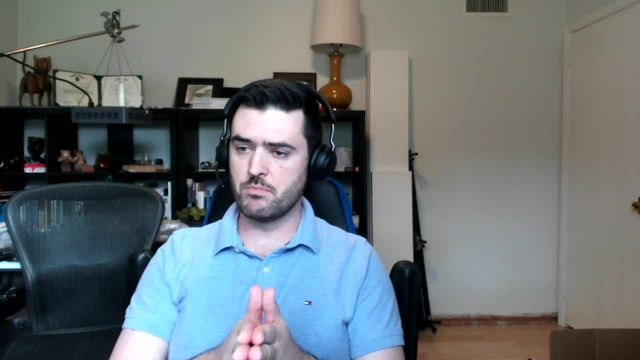 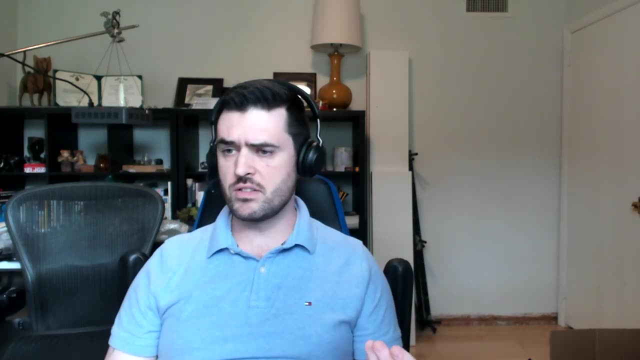 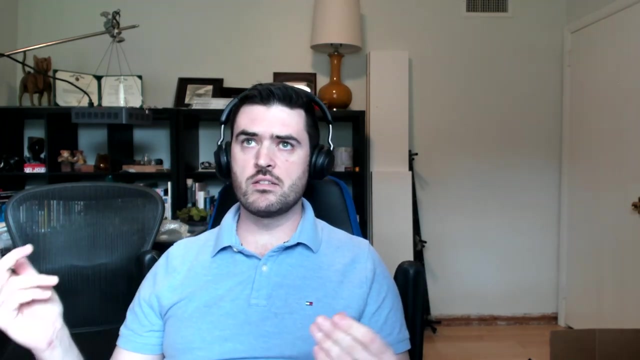 those were. the majority of that information was applicable to both 27001 and 42001.. So for organizations that are looking to address information security, privacy and artificial intelligence risk and internal external obligations, it's much more simple to do an integrated management system. 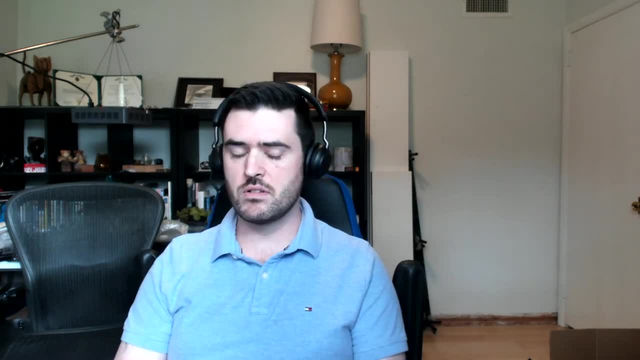 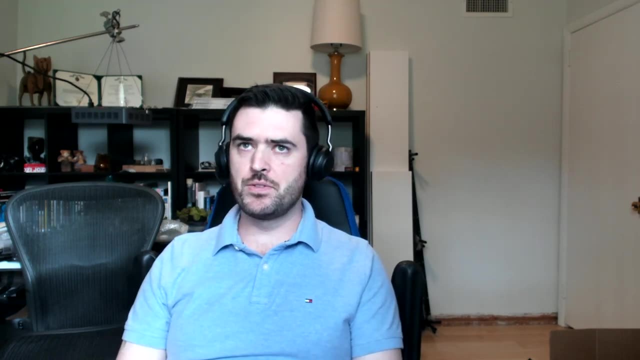 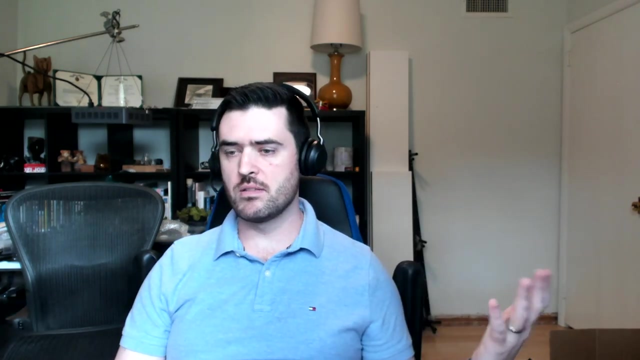 because you can enhance- let's say, you're ISO 27001 certified- you can enhance existing documentation, existing processes to set the framework for the AI management system, because you already have a lot of those things in place. You have a management committee. 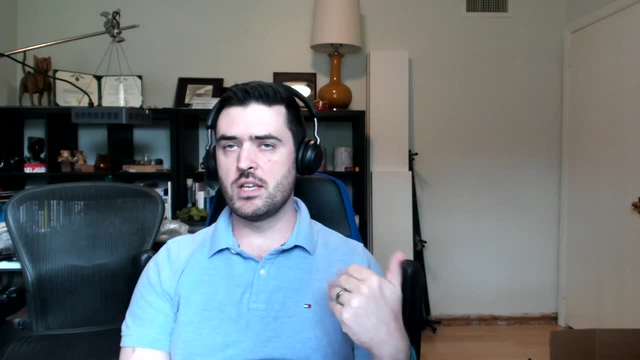 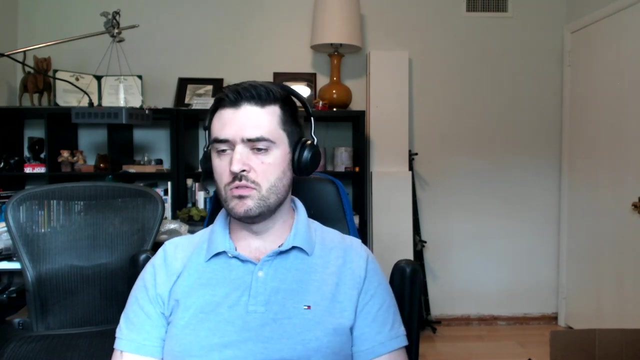 management review and some relevant policies, And so then you just have to do some of the work. that's very specific to ISO 42001.. And then a lot of the concerns and risks associated with artificial intelligence can have something to do with the security protection of personal data. 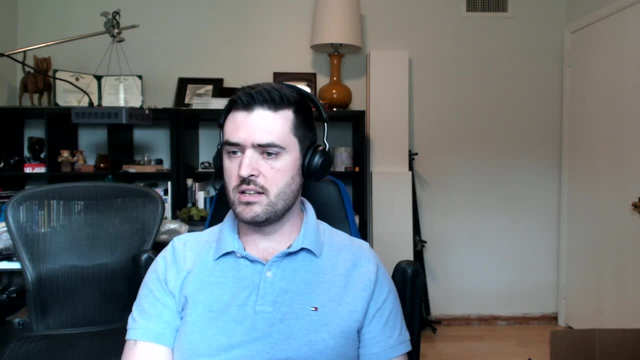 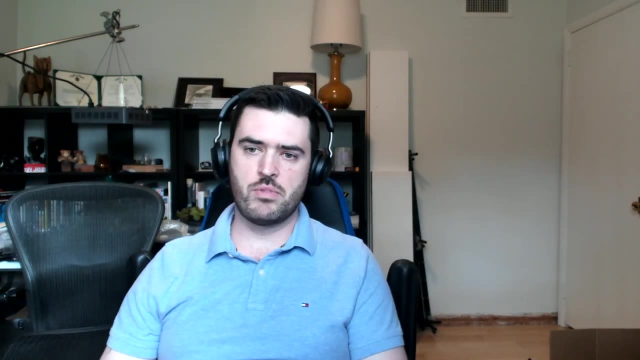 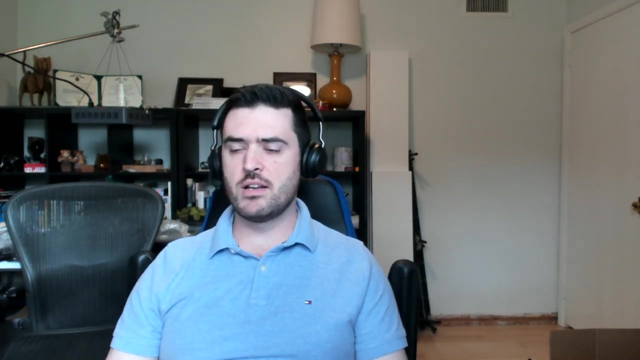 because you're right- a lot of times that's included in the training data sets, or a lot of times that's included in information that's collected and processed through an artificial intelligence application. So that's one of the amazing things about 42001 is not only is there, a fairly small control set, but the clause requirements align so you can really be able to run really well with ISO 27001.. Quick question for you: I hadn't thought about this prior. So ISO 27001 and 27701,. 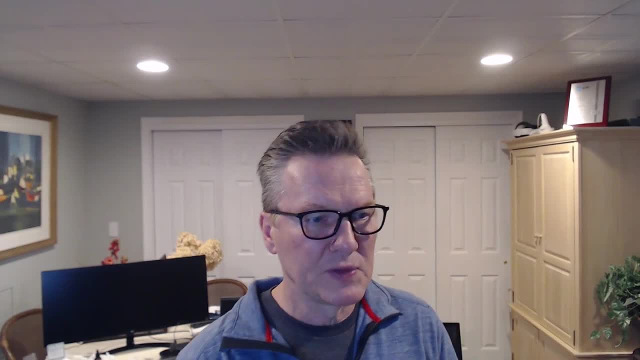 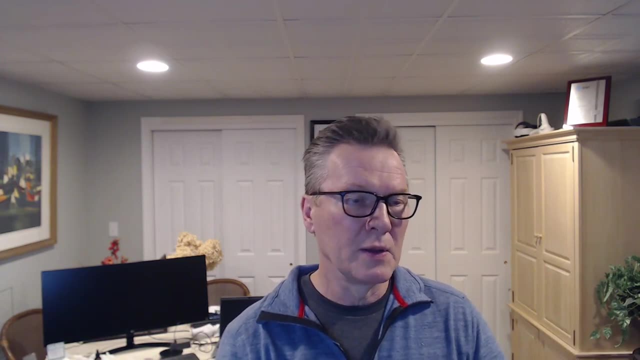 27701 actually alters the construct of the 27001 clauses And it's intended to run in a more unified way, right? Instead of having information security and a privacy management system, you'd have a lot of people call them PIMS, right? 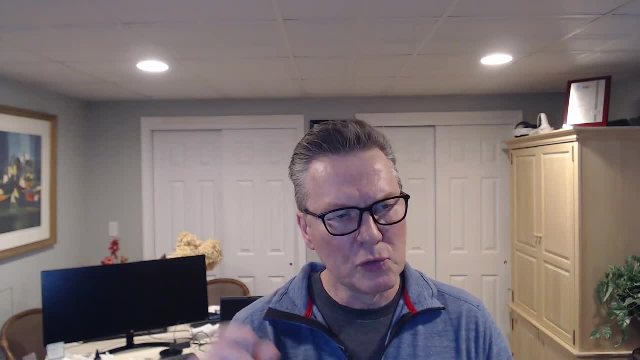 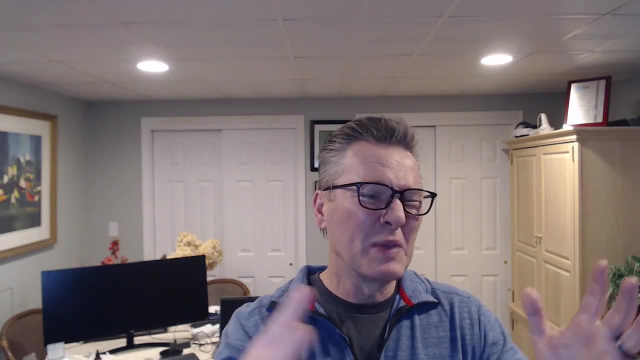 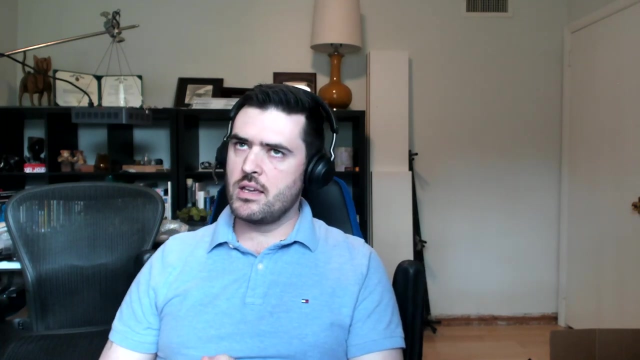 A privacy and information security management system. Is it your thought process that we would with clients that are doing all three, that the AI management system would sort of be integrated into that same and we'd run this through that same single logical construct? I'll say it depends. 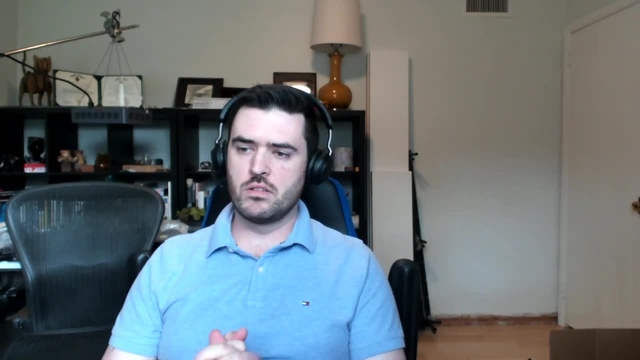 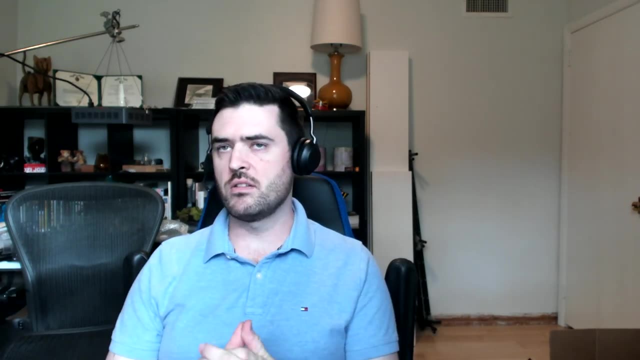 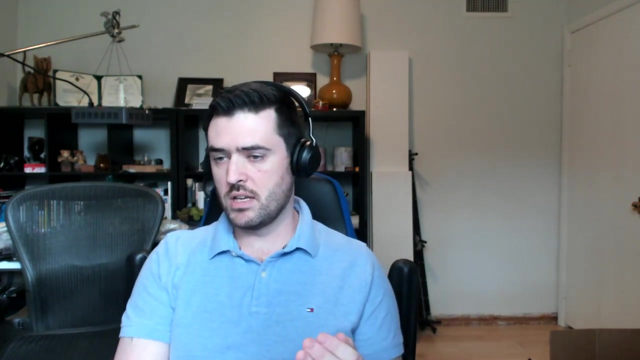 So generally yes, because it's just more efficient. There's a lot less duplicative effort if you integrate those things together. So the areas where it might be separate, so you may have an information security management committee, And if you're to do something that's integrated. 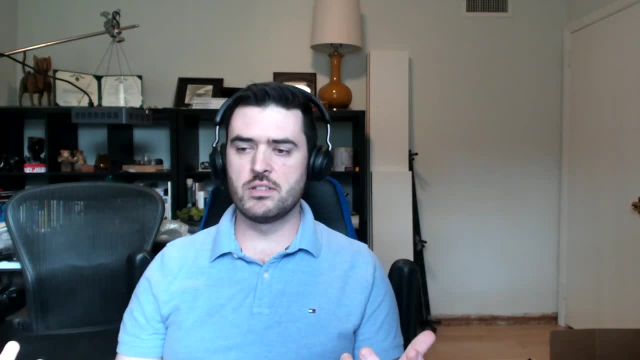 you'd have an information security, privacy and artificial intelligence management committee, But depending on the size of the organization and the implementation of artificial intelligence and how that applies to the organization, you may want to have a subcommittee, but ultimately keeping the leadership commitment. 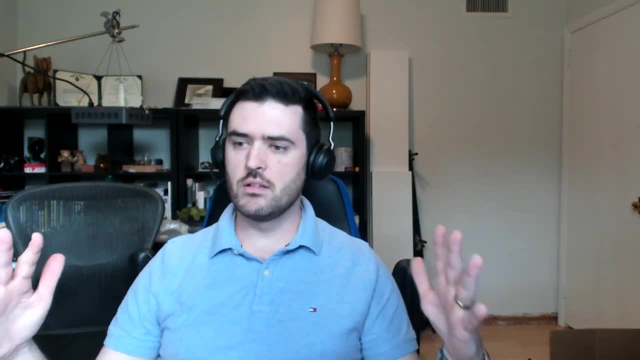 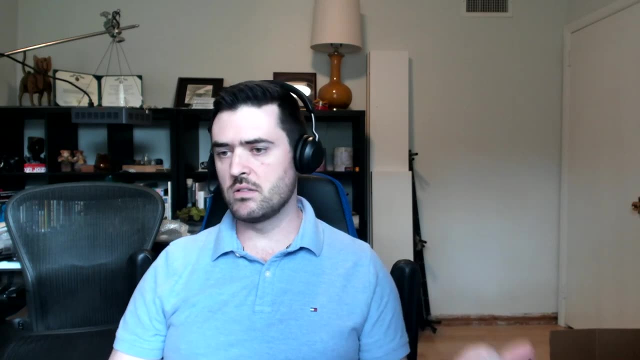 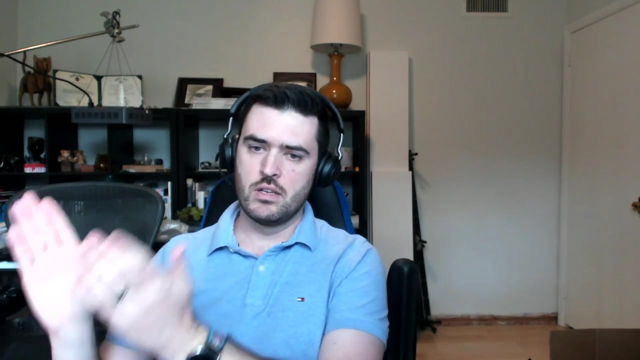 the accountability, the roles and responsibilities integrated is really important. I think that the separation of these things would really happen down at the tactical level, with topic specific policies and unique processes to information security, to privacy and to artificial intelligence. That makes complete sense. 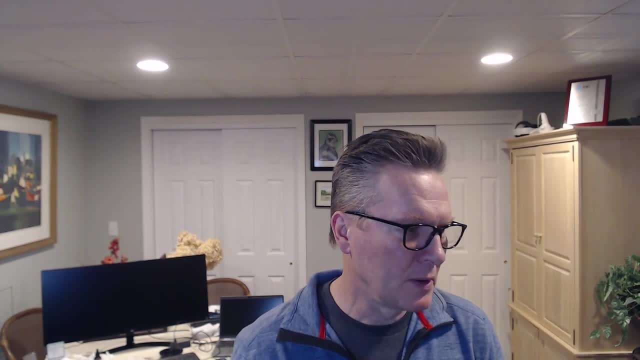 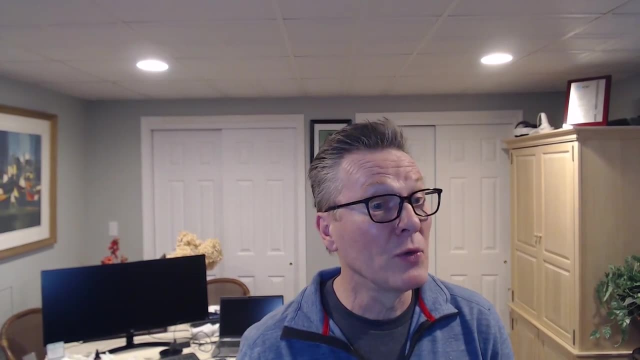 So what I'm finding is that this area, this area is so new that many of the clients that I'm talking to sort of don't know where to begin. or the clients that we're acting as a virtual CISO for: they just they know they need to do something right. 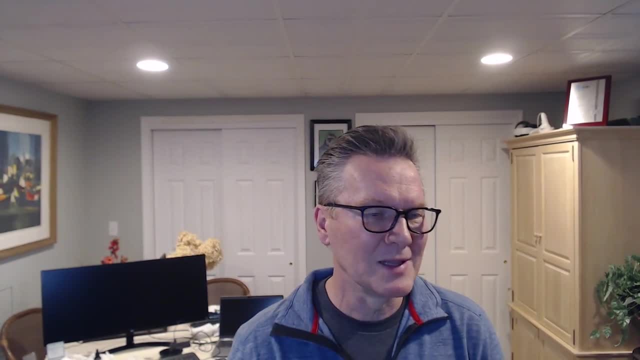 They're becoming aware of that, but they don't really know where to start. So if somebody is listening and they're not ready to jump right in and get to like ISO 42001 level of dealing with AI, what was your guidance for where they should start? 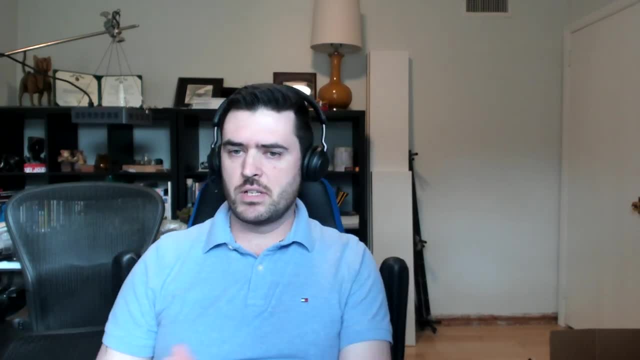 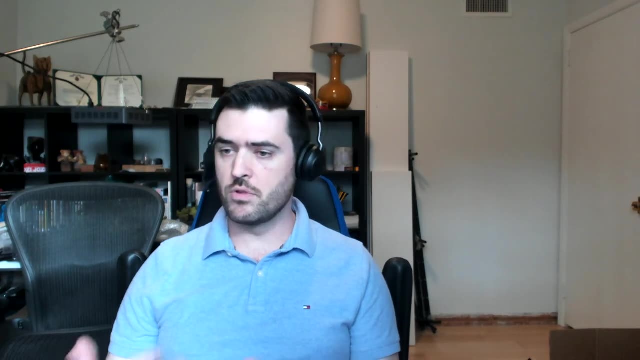 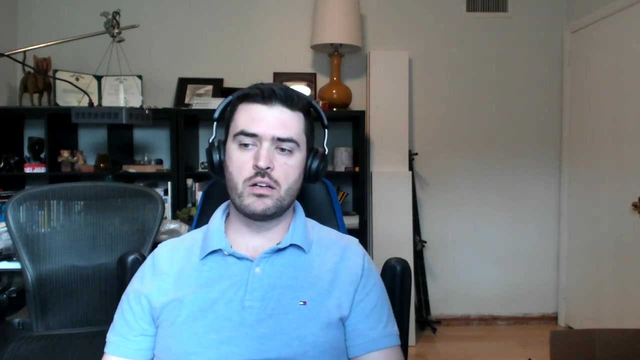 I would provide guidance from a couple of different perspectives, So the first one being organizations that aren't developing, developing or implementing AI formally, but whose employees may be leveraging kind of informal or ad hoc AI applications. So consider developing an artificial intelligence use policy. 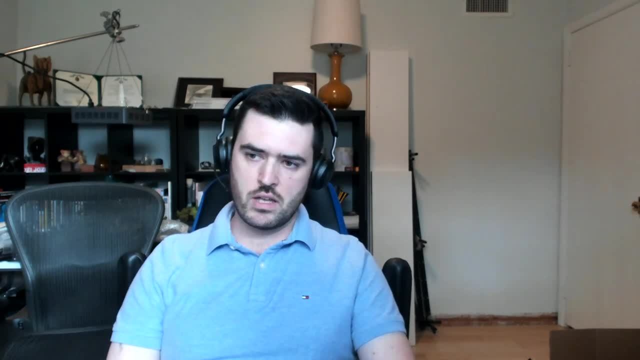 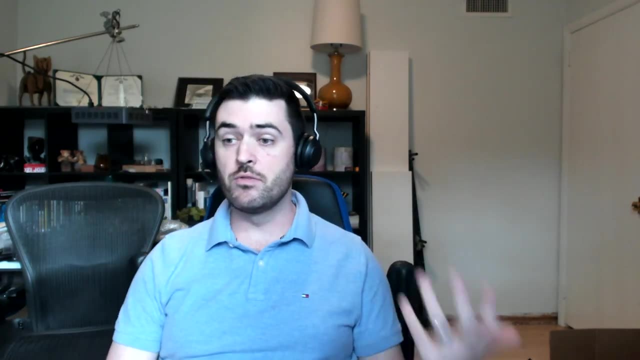 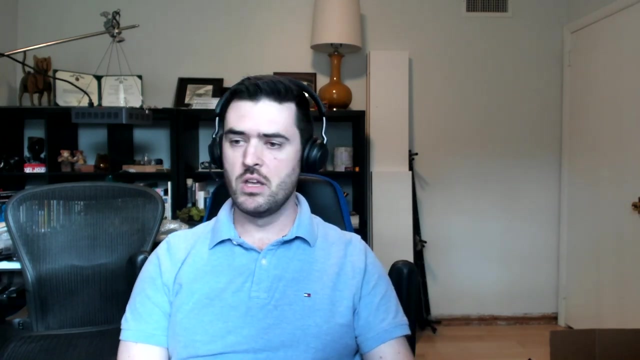 similar to an acceptable use policy. You want to understand how is the organization using artificial intelligence informally and what risks does that introduce, And then establish requirements in your policy that can help reduce some of that risk. And so I would say this will apply. 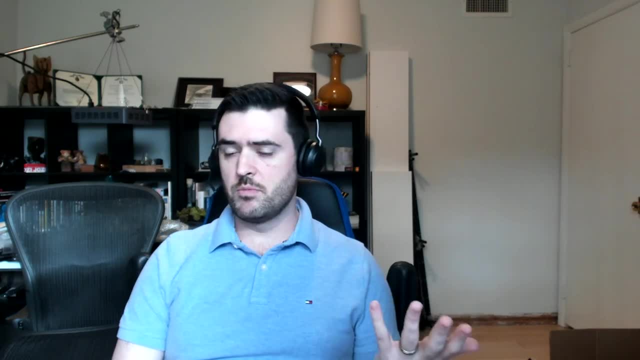 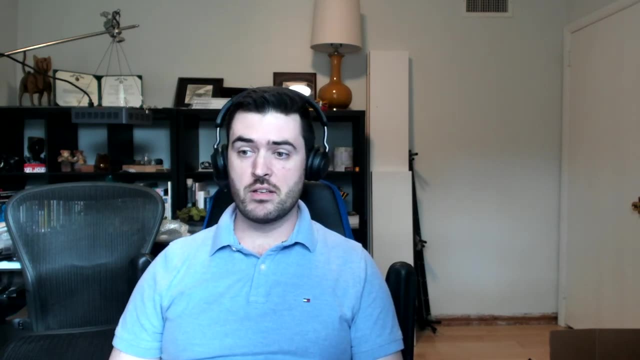 to almost any organization out there. So if you're not approaching AI, it's not something that you're thinking about at this time. your employees probably are, because the tools that are out there today can make almost any process somewhat more efficient in some way. 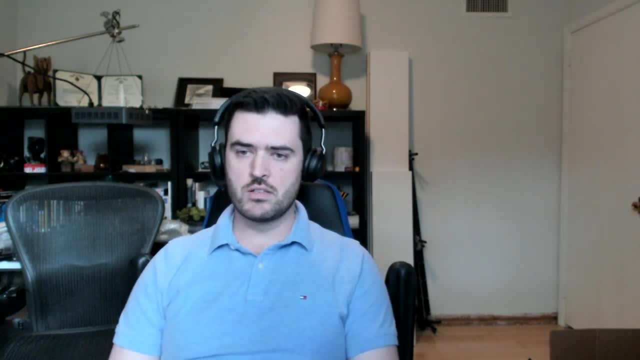 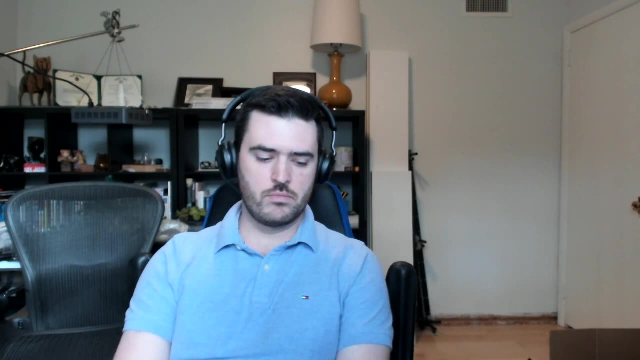 So somebody out there is probably using it in your organization. So at a minimum, consider developing an AI use policy. There's really good guidance out there, especially within the NIST AI risk management framework. There's enough information there to help you understand. 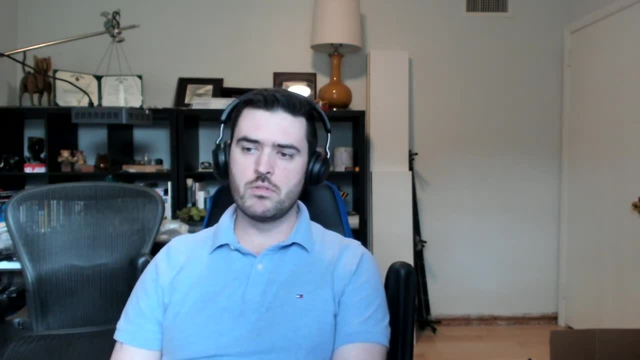 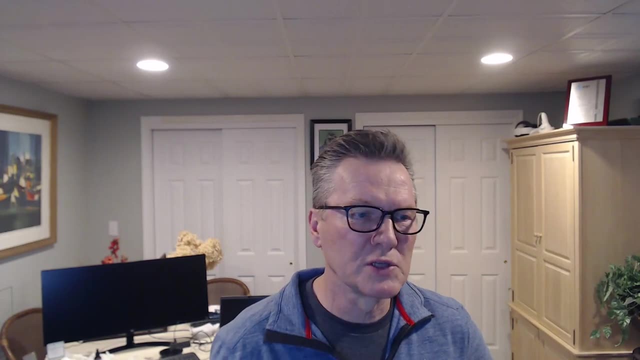 what are some of the risks associated with this and that can help you develop requirements to put in a policy. And then the Yeah, I like what you said, though Oh, I was just going to say I was going to double down on what you said. 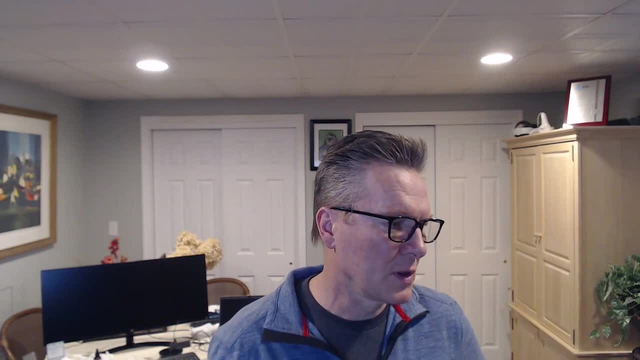 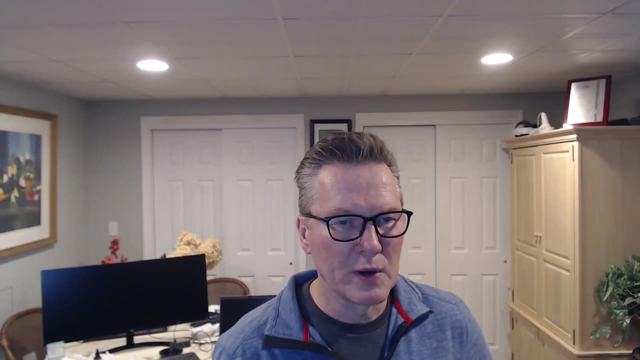 because I don't know that I've emphasized it quite enough when I've chatted with clients- is that don't create the Like. a lot of people are going to go to the internet and download a policy, or they're going to ask someone to give them a policy. 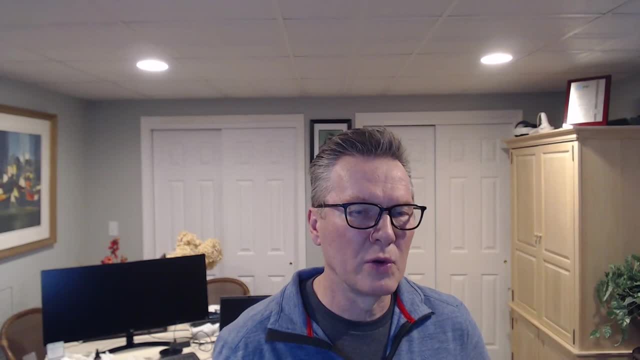 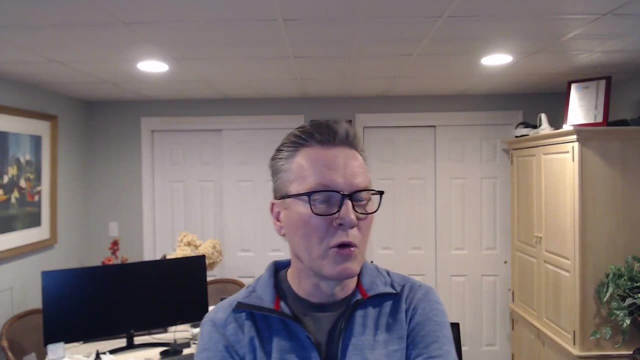 whatever it might be. But you really need to understand risk before you deploy a policy, because the policy is a control and control is a mechanism that reduce risk. We don't really know what an appropriate policy is unless we understand the risk associated with our use. 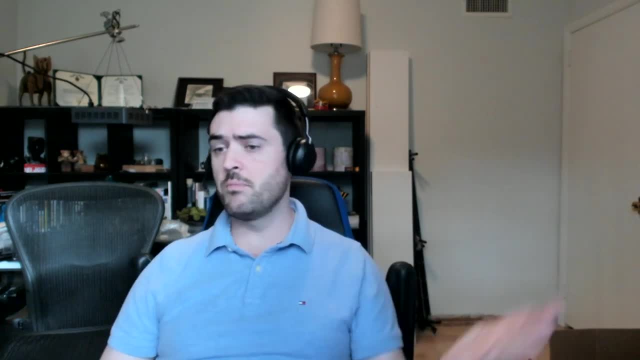 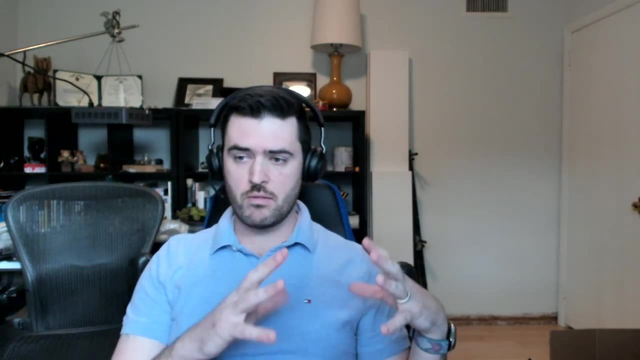 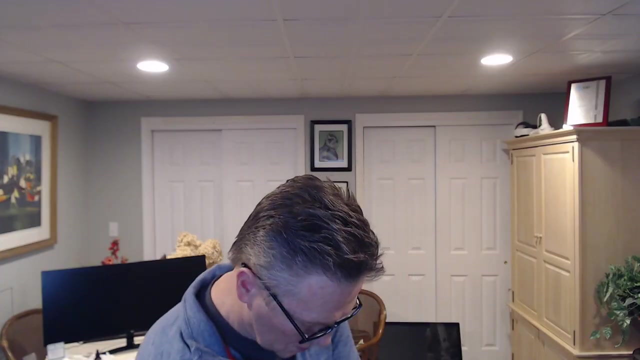 Exactly and absolutely. use templates. Go find templates and see what other organizations are doing, but you have to contextualize it and how you do that is understanding the way it's being used in your organization and the risks that it presents, And I don't think people understand. 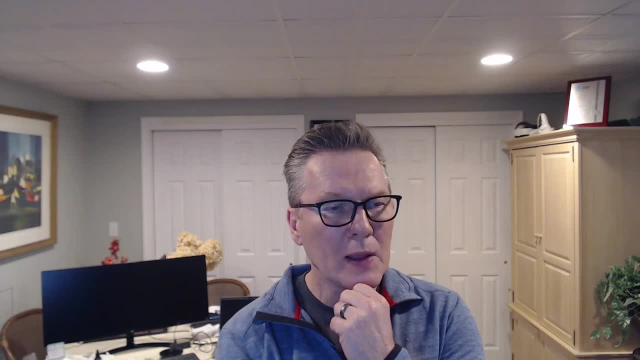 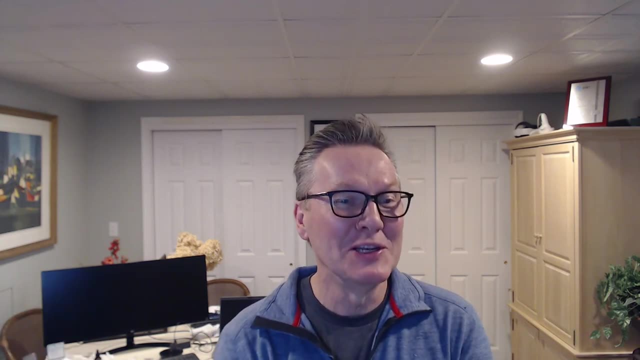 like I was having a chat with a client the other day and they were like: well, we don't allow, we block ChatGPT. I'm like: do you block Bing? And they're like: no, Bing's got ChatGPT built into it. 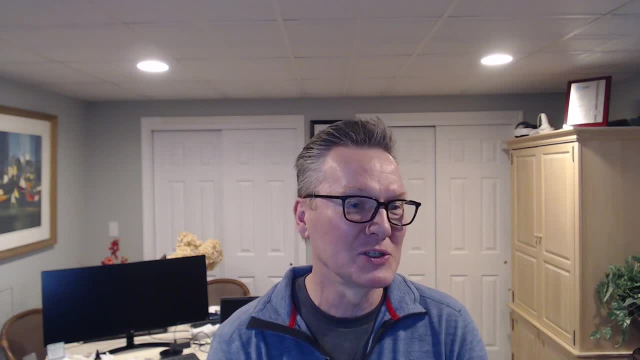 right, so anyone who's using Edge is using ChatGPT And I said, on top of that, virtually a significant number of people, a significant percentage of the SaaS applications you're consuming, right, And we see numbers like a typical enterprise. 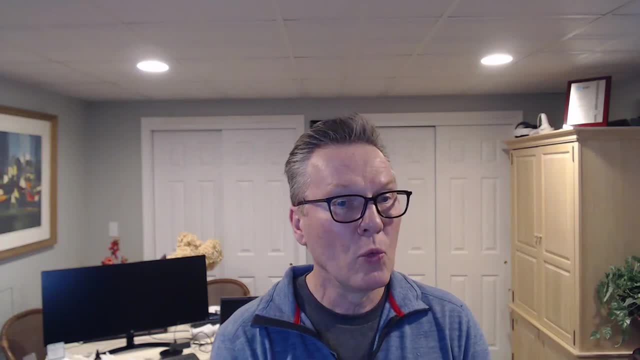 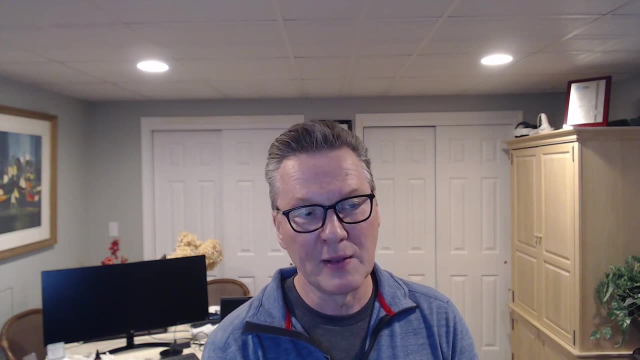 is consuming 1,000 SaaS applications. What percentage of those SaaS applications that are applying some level of artificial intelligence? Right, if you've got all of your human resource tools, and that's where danger comes into play. If you've got an HR application that is scanning. 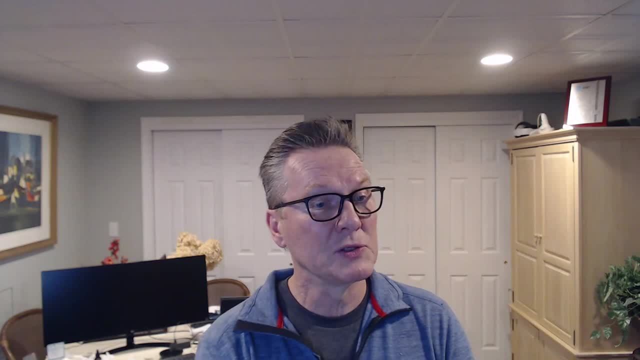 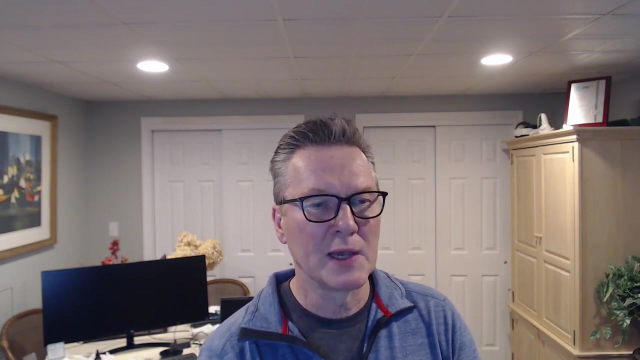 and reviewing and screening resumes. you know they're using AI And if they're using AI and they're using a biased model, right, you could potentially have an issue there. Most of the security tools out there now right that are doing threat intel. 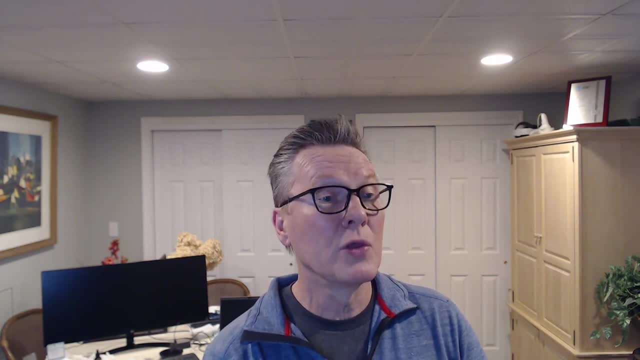 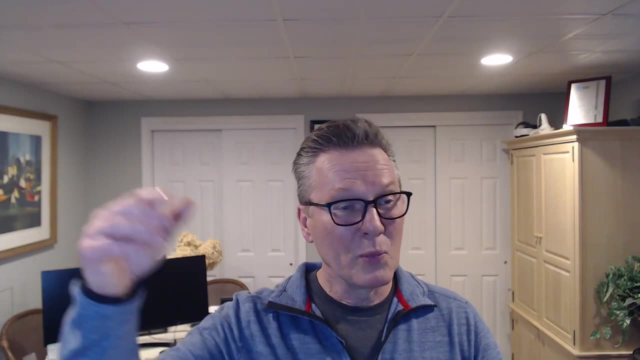 and assessing security logs and things like that. they're using AI. So there's so many tools that are using AI, right, Not only do we have to have that policy, but then we also have to. we got to like. isn't part of this all figuring out? 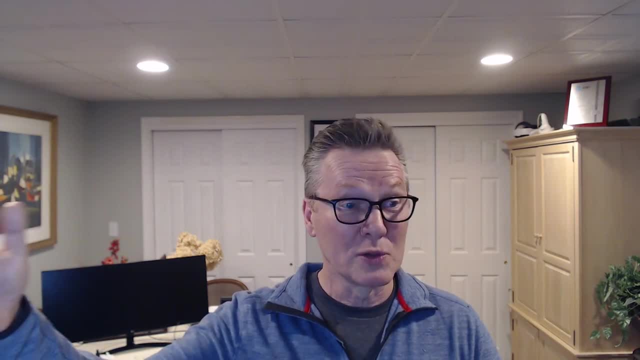 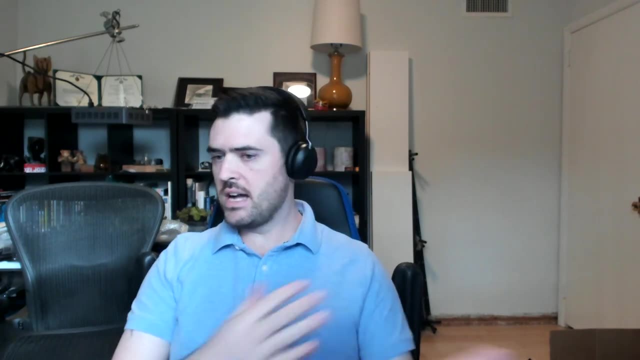 which vendors are actually using AI and then making sure that they have the right. you know they have the right. you know they have the right. you know they have the right control mechanisms in place to protect us So you can have ad hoc use of AI in the organization. 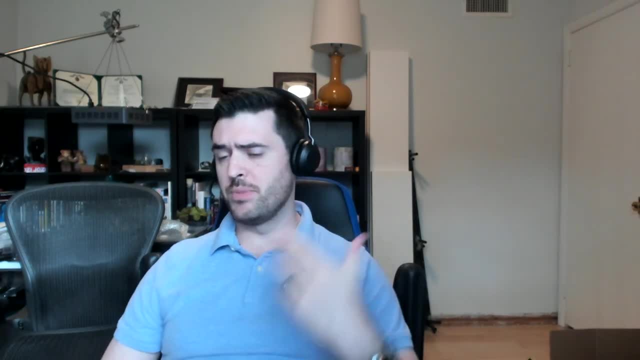 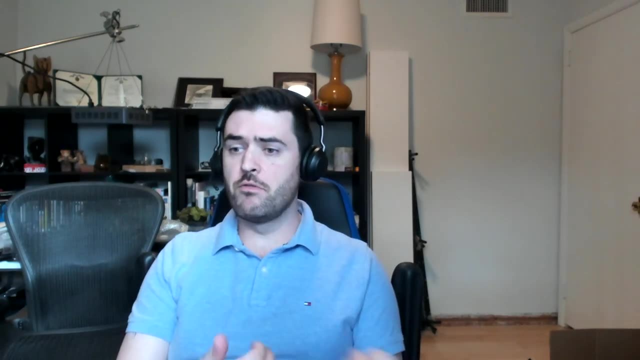 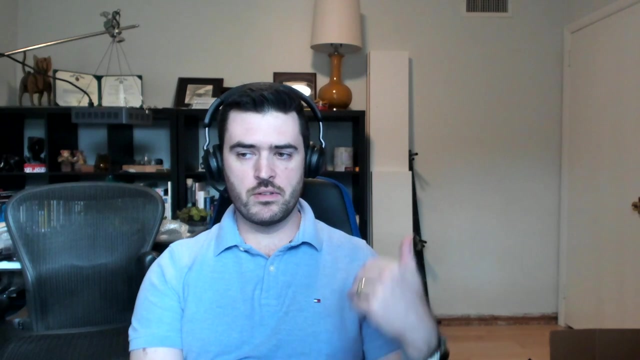 employees using things like ChatGPT and Bing and Copilot and things like this. But then there may be applications that have been formally approved for use in your organization that have new features that leverage AI, And so, if you're going to implement a policy, 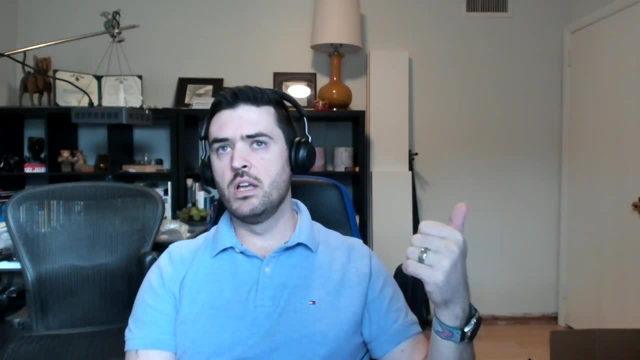 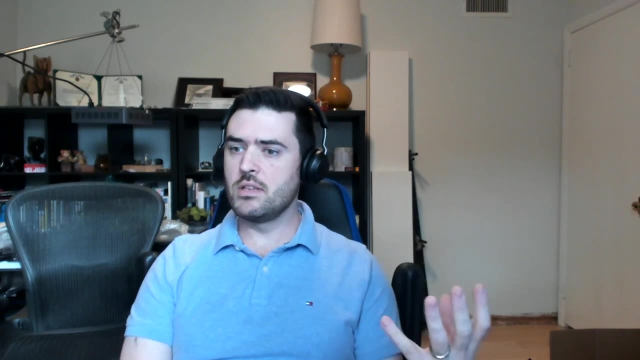 or even if you're going to do more in this next category I'll talk about, do an assessment. How is artificial intelligence being used in the organization? And you need to define what is artificial intelligence mean to this organization. There's a variety of definitions out there for what it means. 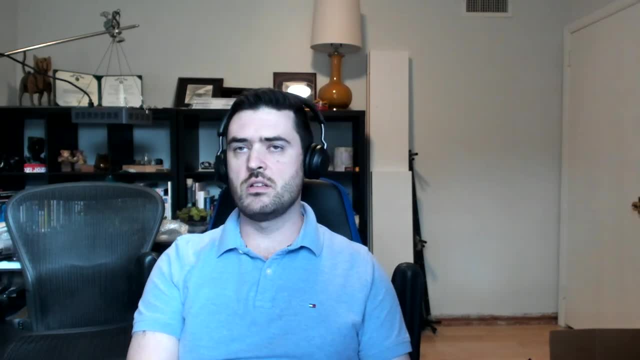 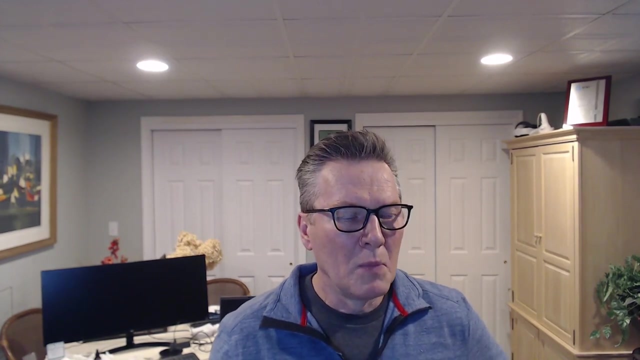 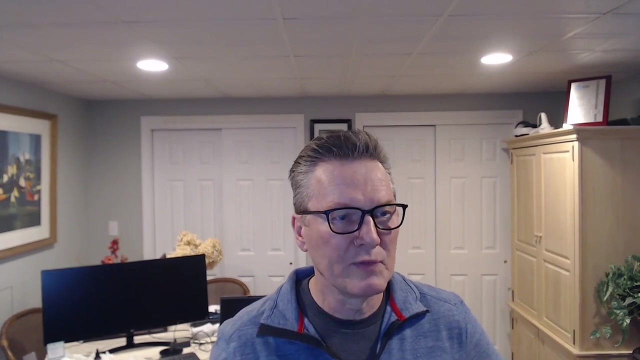 So you need to establish what your organization defines artificial intelligence to be and then go out and find where in your organization that that's being used Gotcha. So that implies to me that updating your third party risk management program, vendor due diligence program, 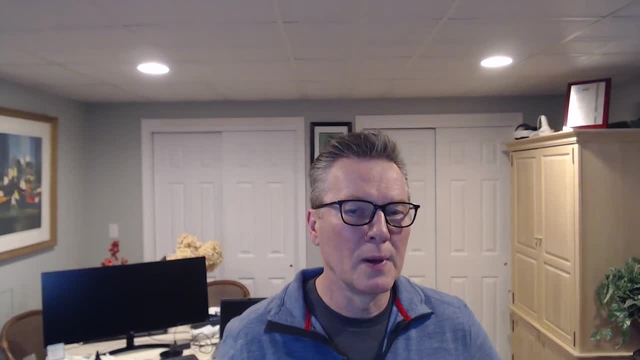 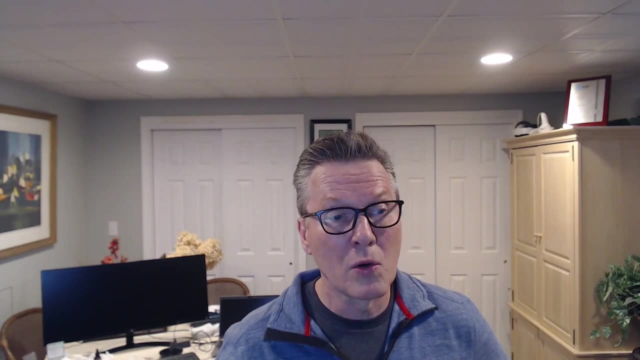 whatever you're calling it- vendor risk management- to ask those. begin to ask those questions about the use of artificial intelligence and how they are or are not complying with the guidance- good guidance- that's out there. That would be another next step recommendation. 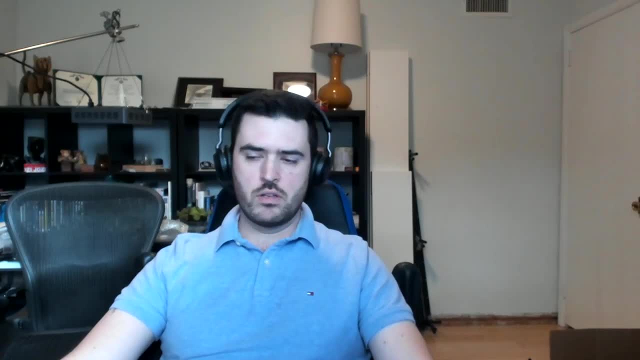 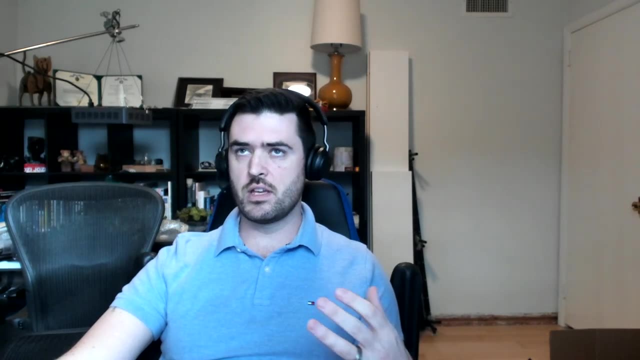 beyond getting that policy. you know understanding the risk with the policy in place. Yeah, so that's going to be a really good opportunity to determine how artificial intelligence is being used in the organization. a couple of angles here. So if you ask your SAS providers, 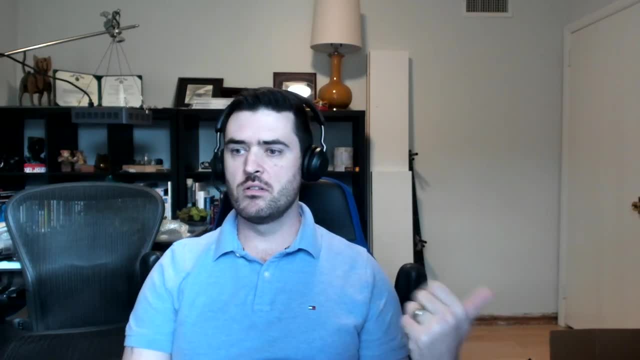 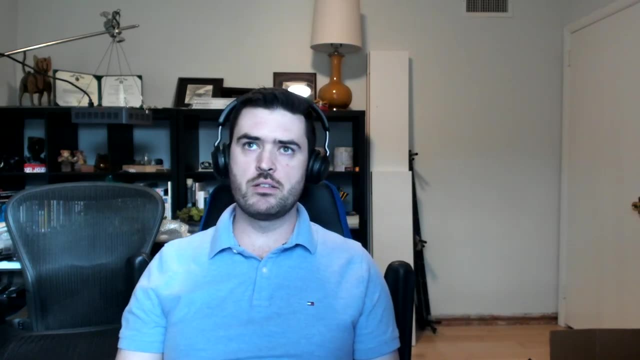 do you leverage artificial intelligence to provide these services? you may find in a lot of cases they say yes And you didn't know this previously, and it may not be because they implemented artificial intelligence recently because of large language models, Although Yeah. 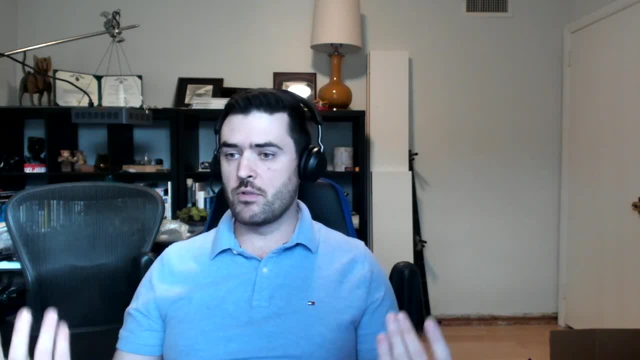 Certainly that's a case a lot of times, but maybe you're just discovering that they've always used artificial intelligence in some capacity. And then, because of the awareness, as has happened with the rapid development of large language models recently, you now have to pay attention. 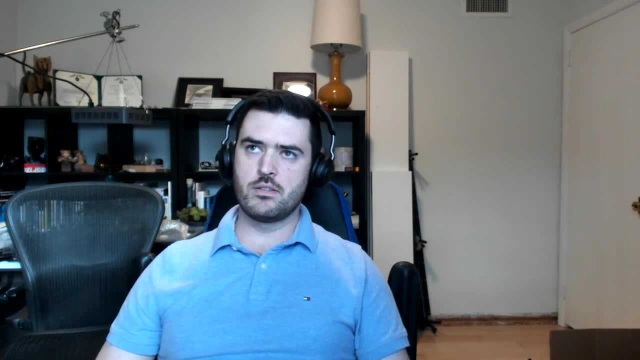 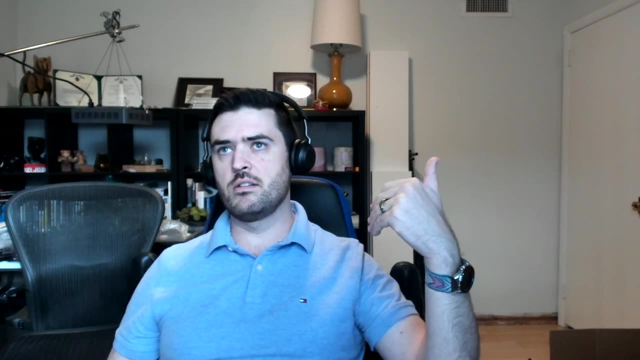 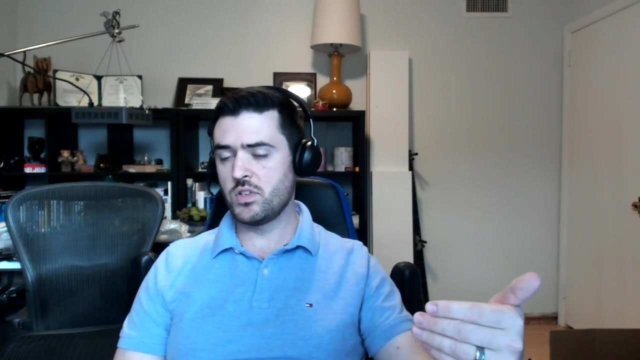 Okay, what does that mean? So there is the aspect of understanding. how do we reach out to our vendors and understand how they're using artificial intelligence in the services they're providing us, but then also, how are they using artificial intelligence within their organization? 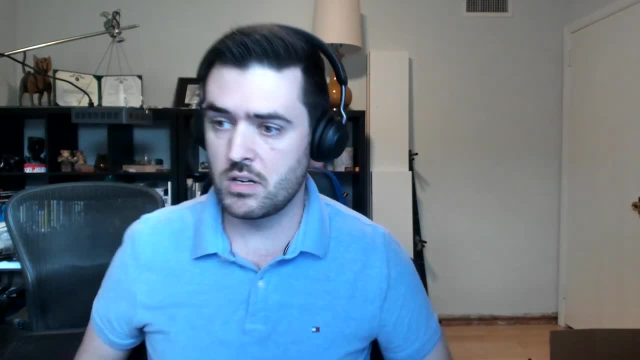 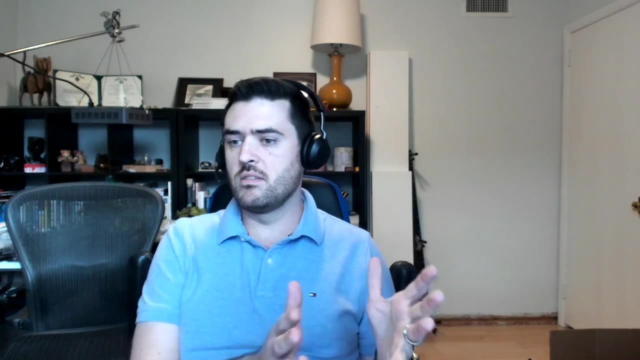 and what risk does that present? just by them using artificial intelligence? So they may use ChatGPT internally. It may not be used in a way that is within the service provided to you, but it might introduce additional risk for that organization being able to provide. 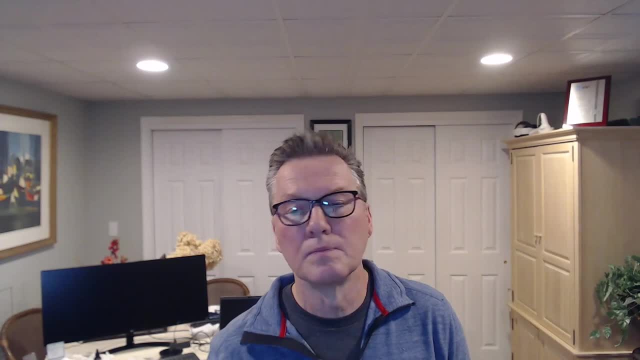 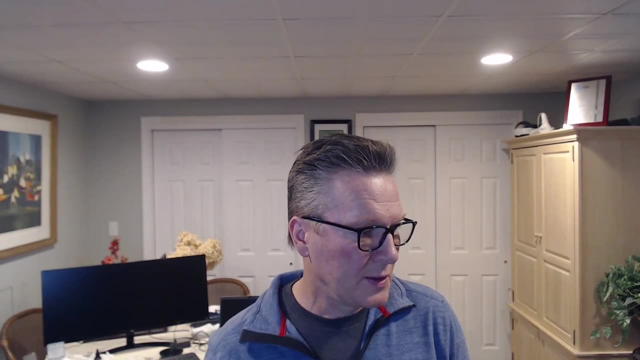 that service to you effectively. Yeah, and I like something you said and I never thought of it- Sort of defining what AI is within the context of organization, because I don't think people realize how pervasive it's become, right, You know anyone that sit down in front of their TV. 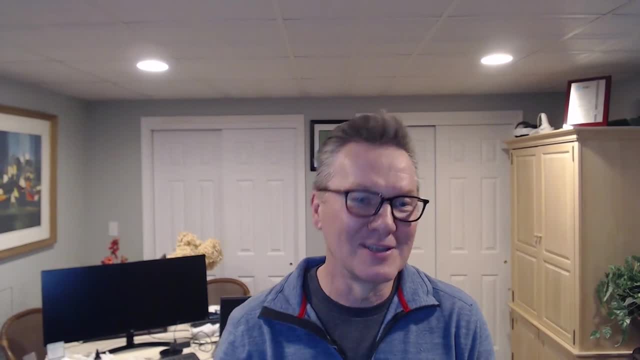 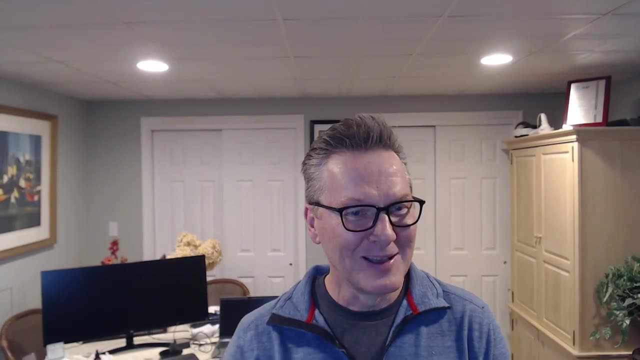 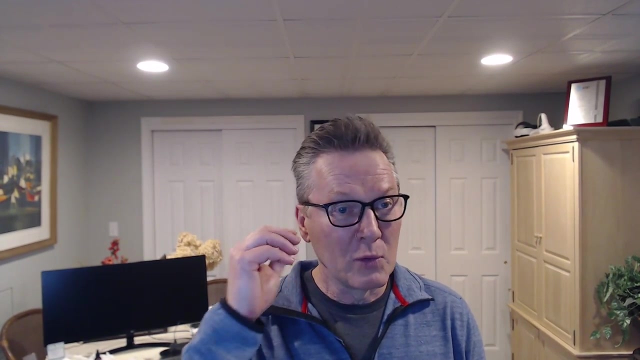 and hits Netflix, that recommendation engine is artificial intelligence. I mean, if you are talking to- and I won't use her name because she's sitting next to my desk, but if you're talking to a virtual assistant of that nature, uh, you know artificial intelligence. if you're talking to your car, uh, if you know all of these. 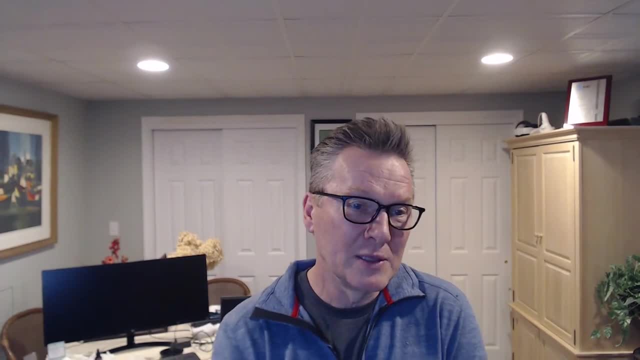 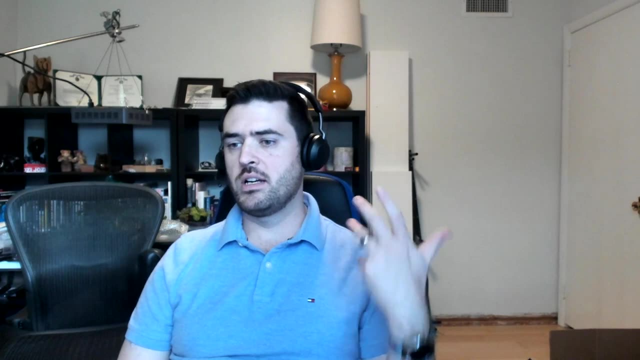 systems right are using ai at this point. so it's a lot more pervasive than we think, and i think that organizations need to be aware of that, something that it can be really easy to get caught up in the hype of of artificial intelligence right now. um, but what has happened recently is the 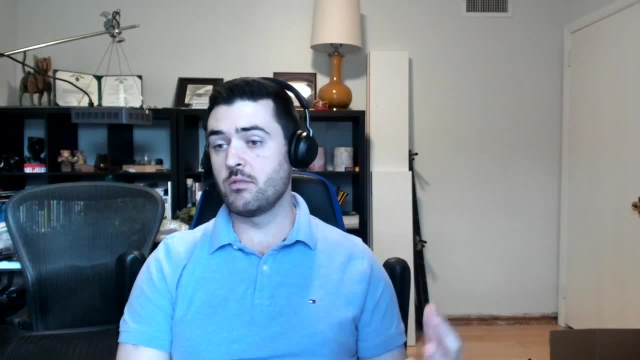 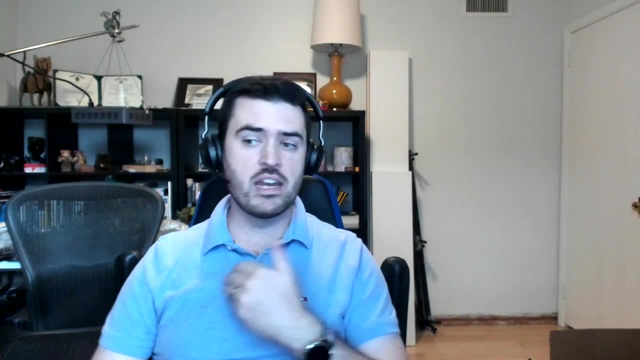 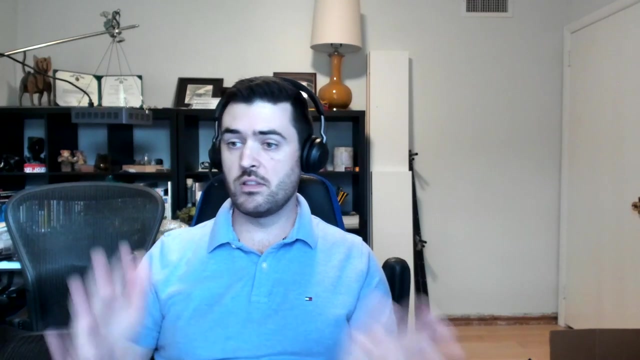 relevant development of large language models where it doesn't take uh uh data scientists to interact with these models. anybody can interact with these models and find benefit in that, and so, um, there is unique risks with large language models and that's causing a lot of the reactions. 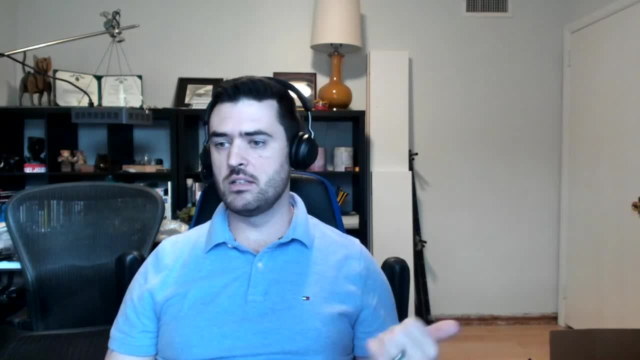 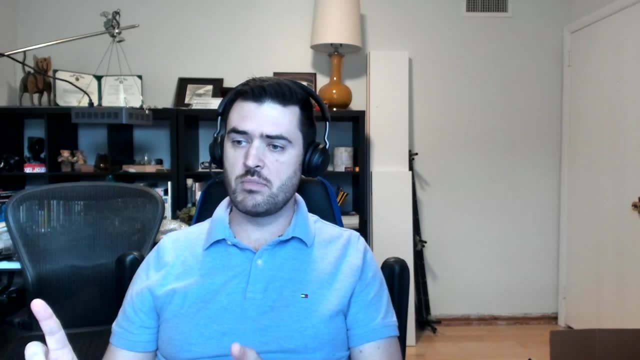 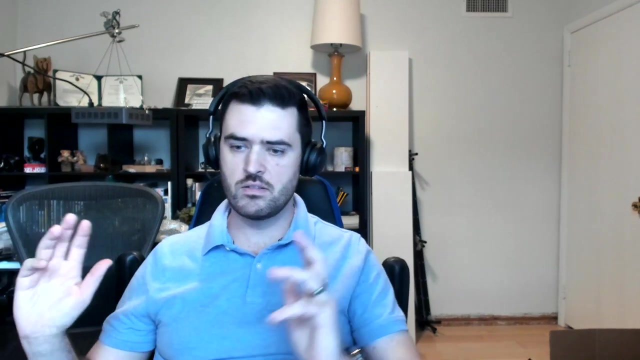 like the executive order, the ai act, um, and different standards and frameworks coming out to help people um, manage risks and opportunities with these things. but then that's also causing people to say, okay, wait a minute, there's artificial intelligence outside of large language models. how do we apply this to artificial intelligence that we've been 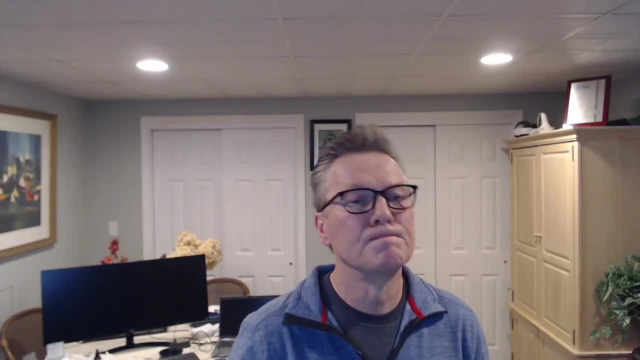 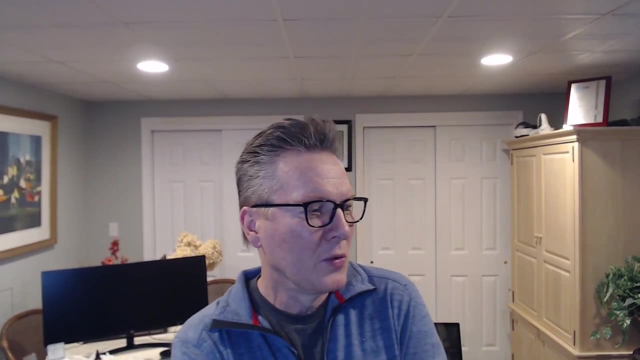 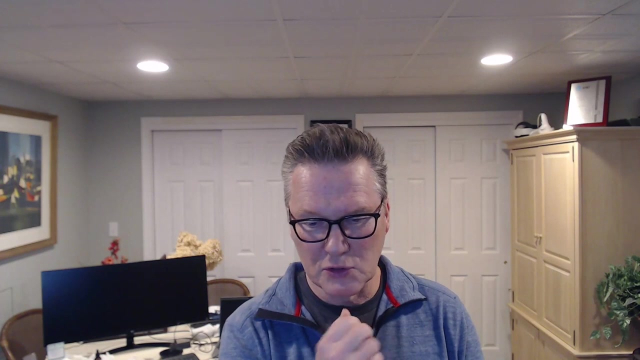 using for years now. yeah, one one pointed risk i'll point out that i just heard about through a client was they were piloting microsoft co-pilot, which i think is going to be a fantastic product. i'm excited to use it. i hope i get a chance to use it soon, uh. however, 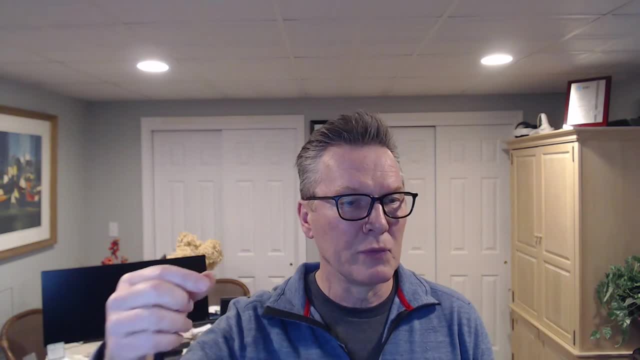 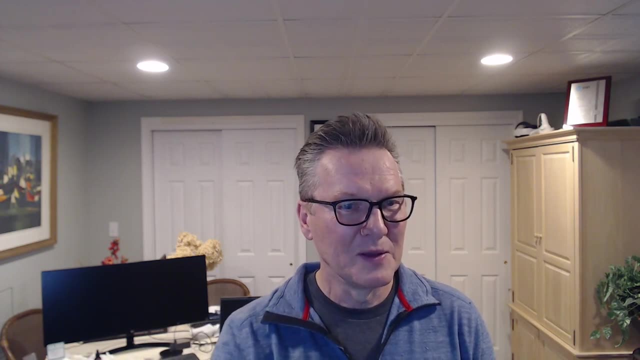 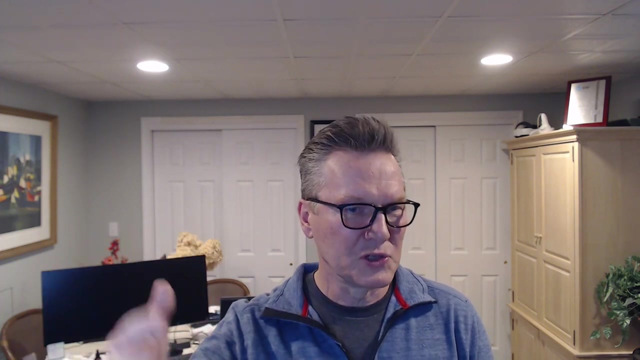 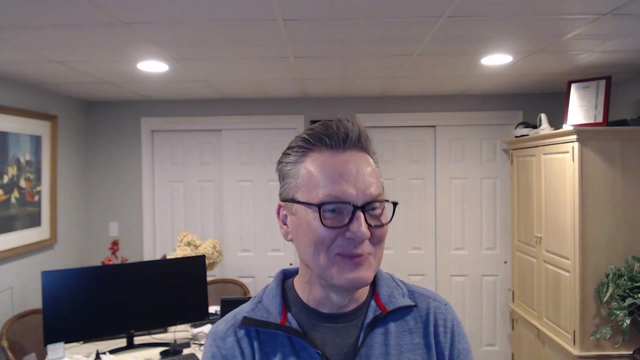 if you do not have the right restrictions on data sources within your organization, co-pilot finds them and uses them. so they had a human resource folder that didn't have the right permissioning on it, that had confidential salary information on it, and somebody asked co-pilot a question and was able to retrieve- uh, all of that data. so so for anyone, 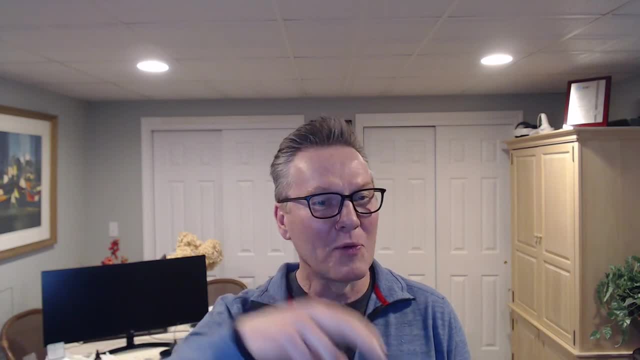 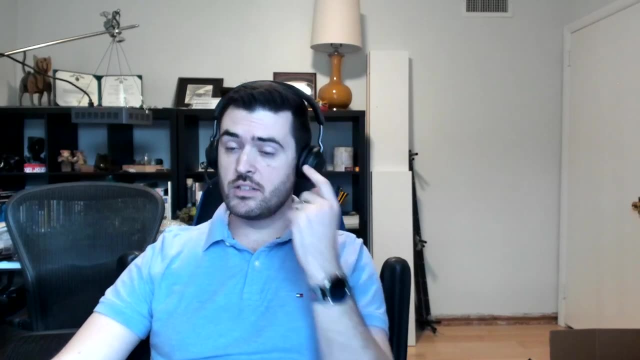 who's thinking about it. i think it's a great way to do it and i think it's a great way to do it. so if you're thinking about deploying co-pilot, do understand that there are probably some things you need to do ahead of that to avoid anything unexpected. this is a really good opportunity to 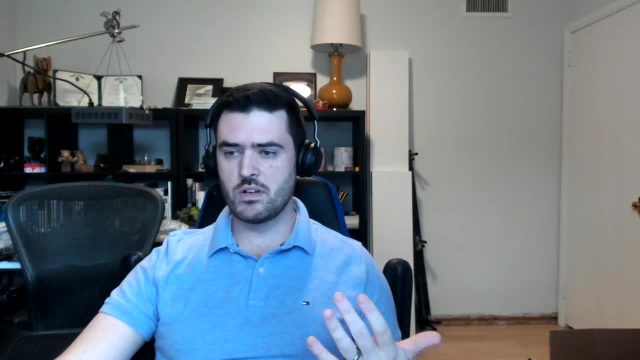 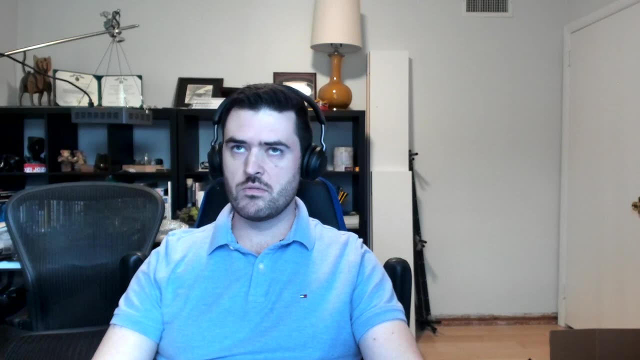 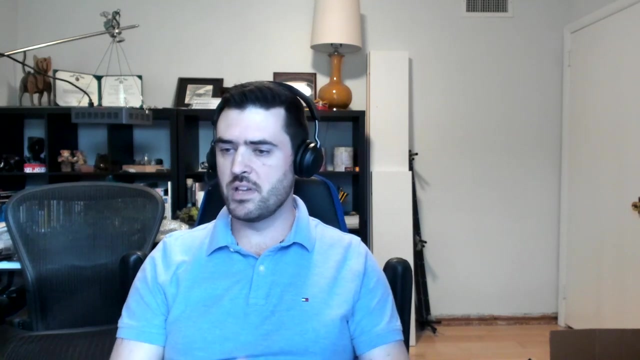 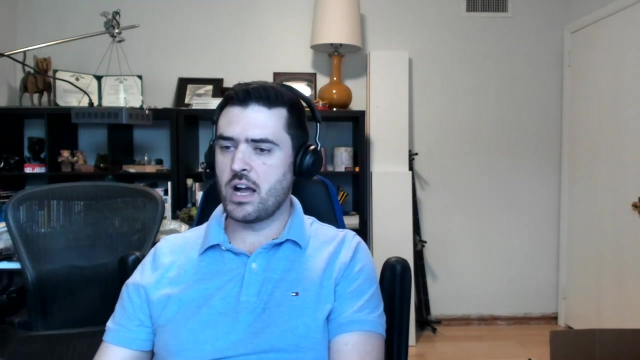 talk about how um iso 27001 is really relevant here and supports iso 42001. so in this instance of access control- right governing access control for users, governing it for systems- that's been a problem for for decades now, and now we have to say: how do we, uh, appropriately manage access? 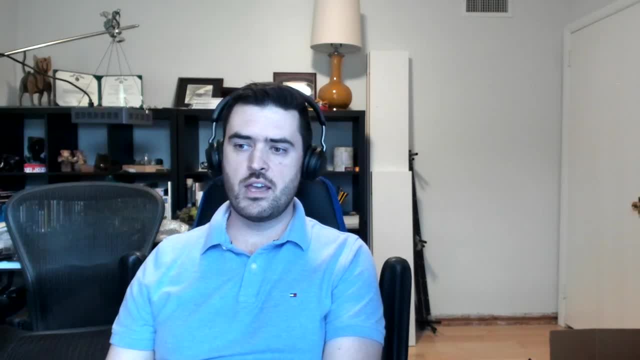 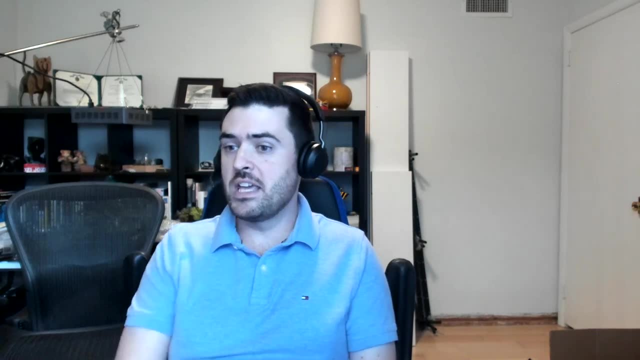 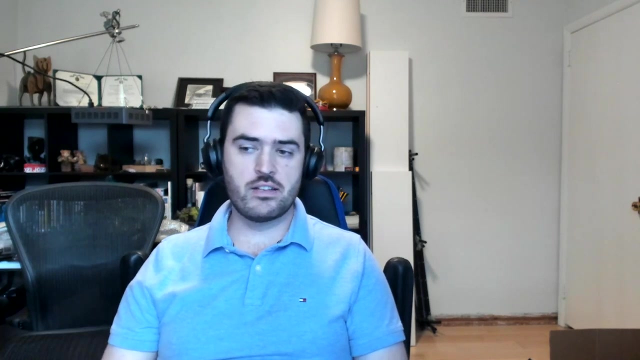 for artificial intelligence systems because they are kind of in the middle between systems and users. it depends on how you implement them. um, they it could behave like a user, um, but in the case of the, the hr file, uh, it just being a permissions issue. that's just a simple information security. 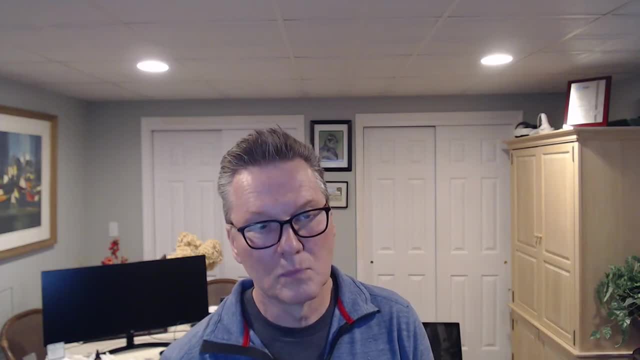 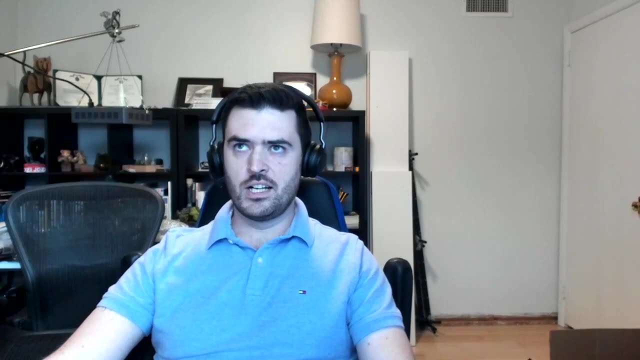 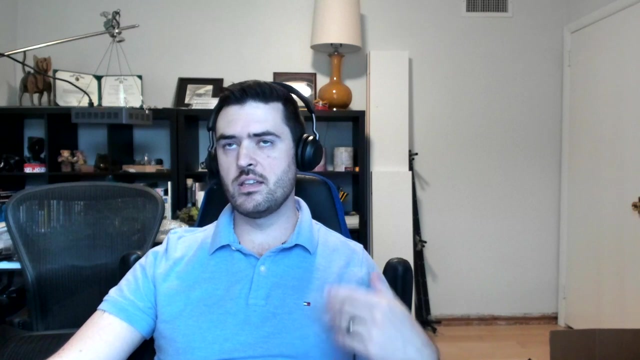 control, but the context wasn't there, right. yeah, pretty cool. uh, we beat this up pretty good. is there anything we missed from your perspective? i did want to point out something uh else about iso 42001. so we have annex a, which are your controls, and then we have annex b, which is the guidance on how to implement those controls. 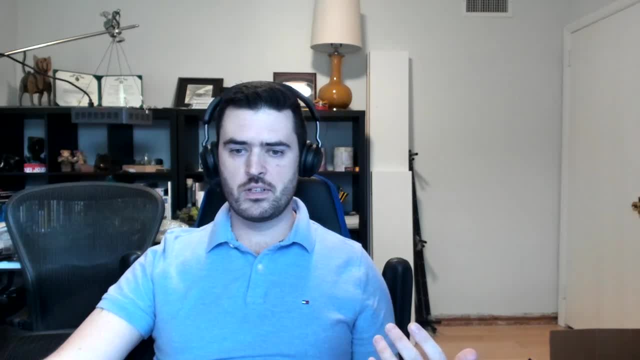 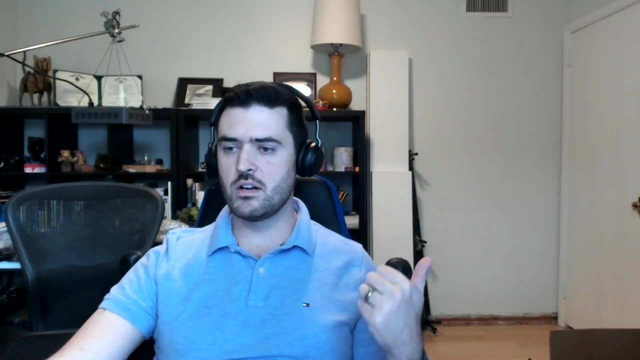 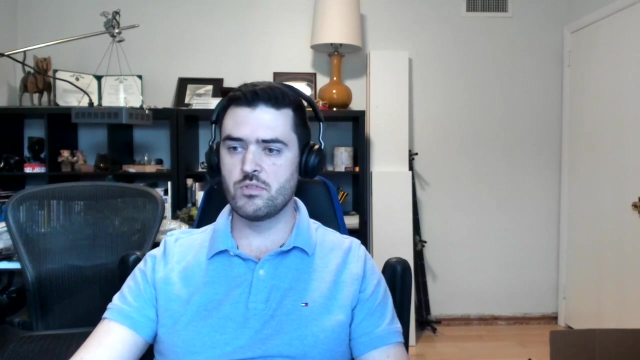 um, but there's also um, an annex c and an annex d, and so the annex c provides uh. both those two annexes are informative, so they're not requirements. but annex c provides really good guidance on uh and examples of ai related organizational objectives, as well as what are some of the potential sources of artificial intelligence risk. so it's just. 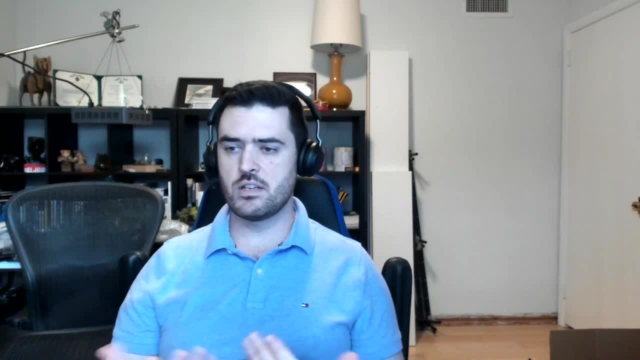 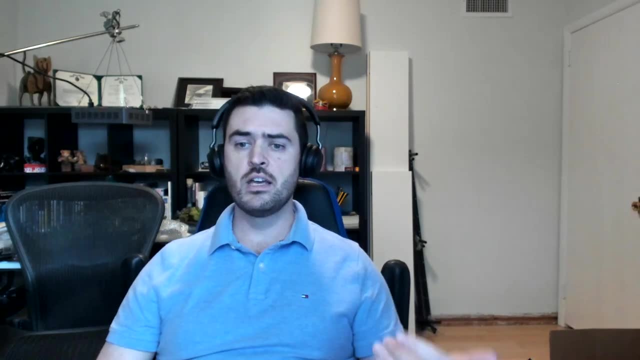 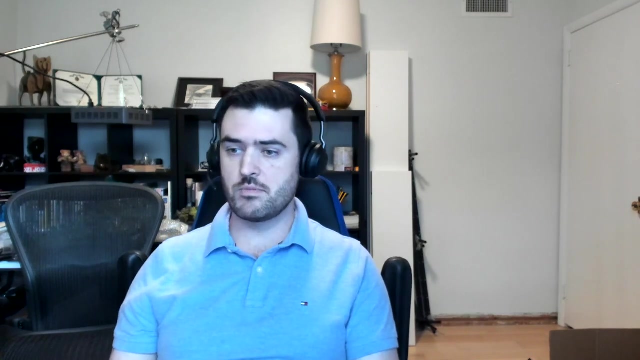 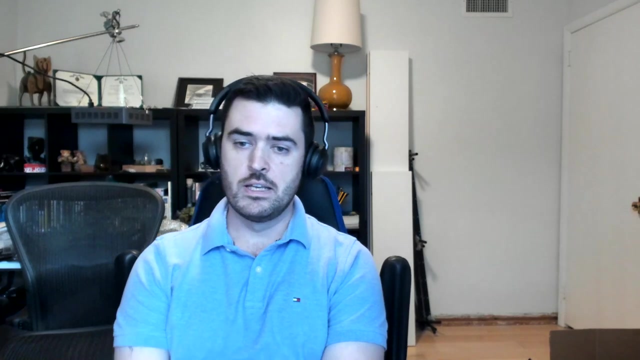 another step above guidance and helps organizations really understand the context of the ai management system. and then, finally, in annex d, it contains some brief guidance on integrating the ai management system with other management systems. like it mentions 27001, 27701 and, uh, even iso 9001. so it's 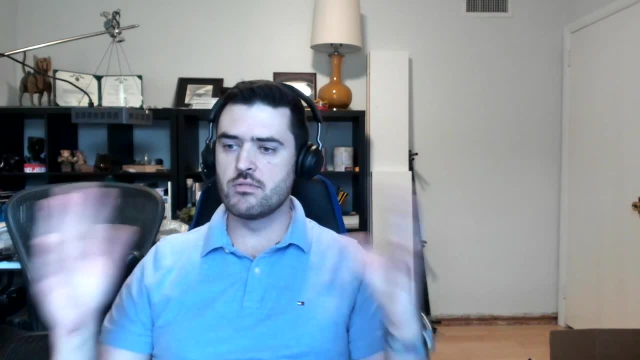 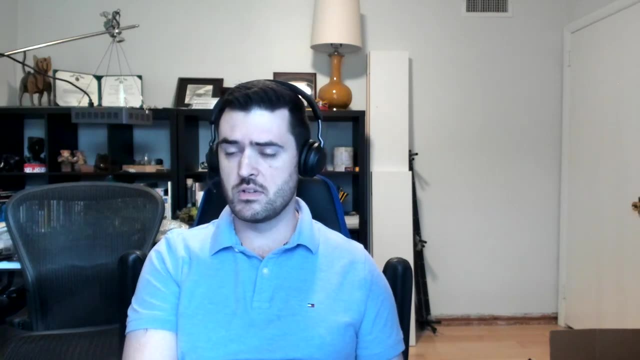 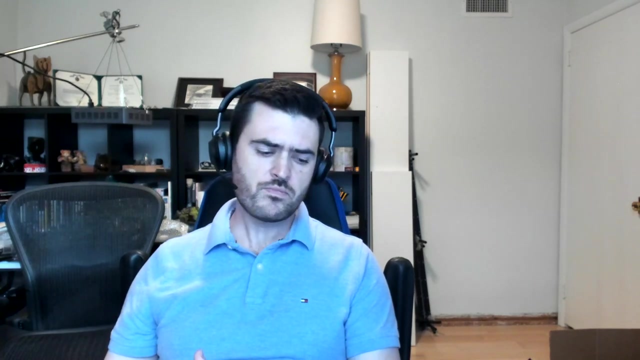 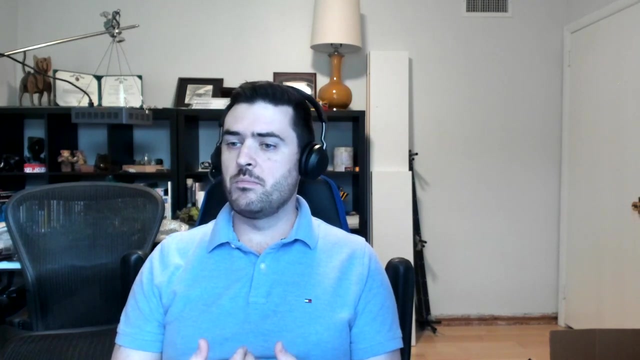 just some extra information that really rounds out the the standard documentation. so i think that organizations that especially who have already implemented iso 27001, should have no issue understanding how to really implement the management system. i think where the gaps can occur, you're only going to be gaat hit different times in the order of skill that you code. 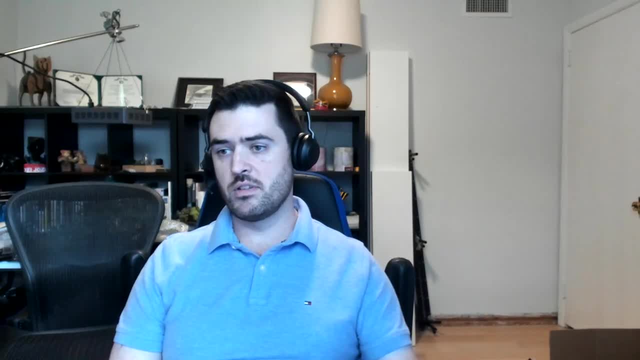 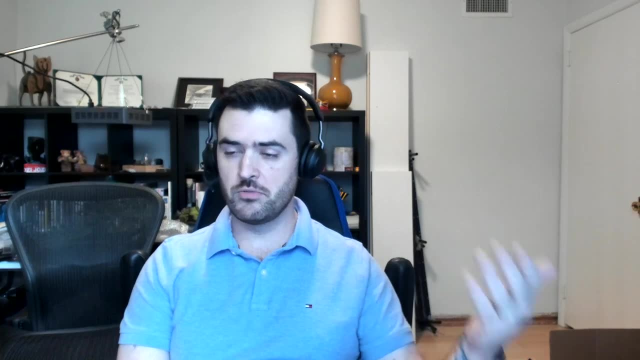 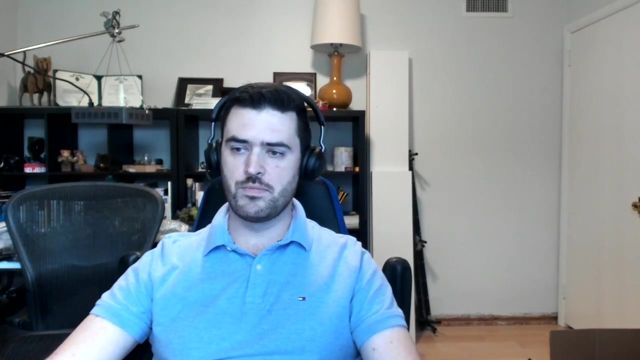 it just doesn't really make the knowledge gaps is: how do you develop secure artificial intelligence? right, you have to have the right resources in your organization to understand that, and that goes back to the clause requirement of having appropriate resources, appropriate competence, uh, with those resources as well. so i just want to give a shout out to annex cnd, because 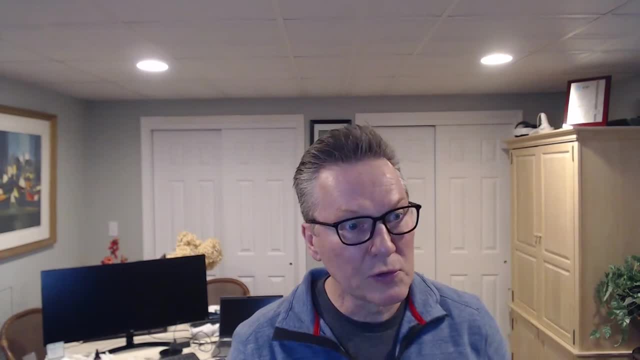 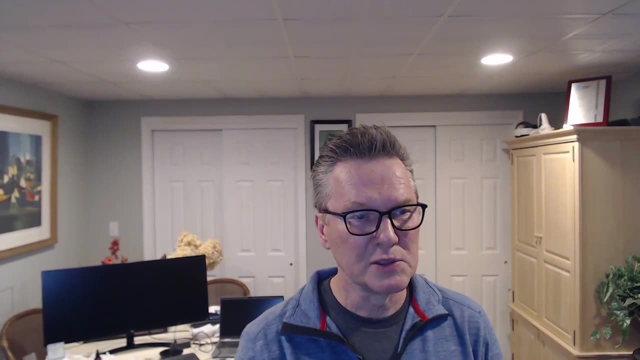 that goes kind of a above and beyond what 27 000 does the 9001 as well, because increasingly we're starting to see people talk about using 9001 to ensure the quality of their SDLC, their development processes And, I think, in light. 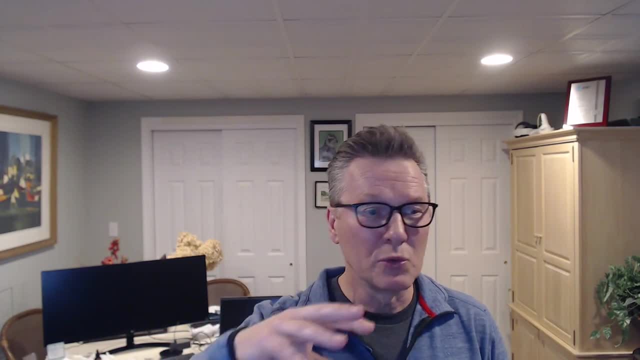 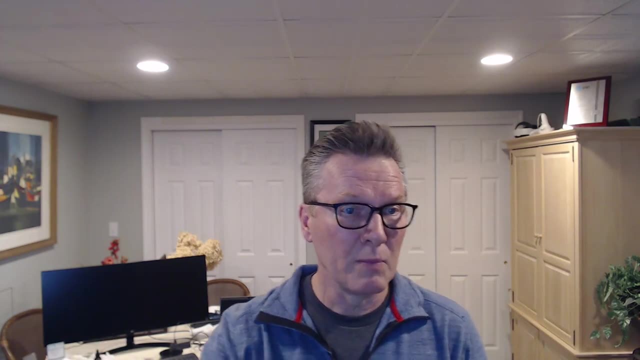 of the potential risk associated with AI, right, Because you were talking about just risks about decision-making. that was around data. And we do have systems that are like autonomous vehicles, right, They're making decisions that could have life and limb or weapon system targeting systems. 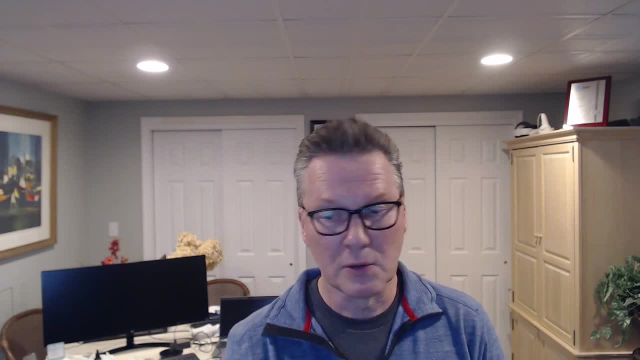 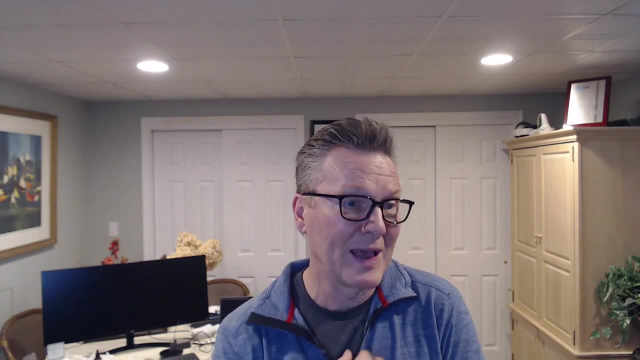 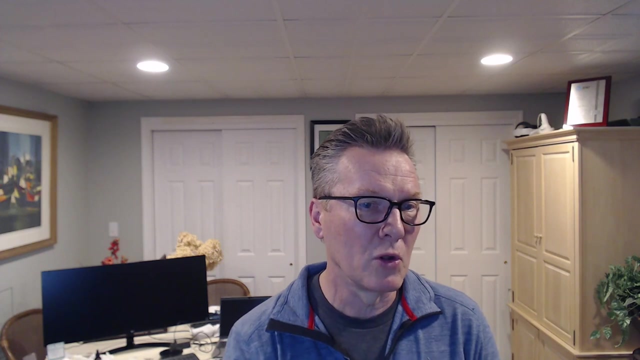 things of that nature, but they all have life and limb implication. So ensuring the quality of those development processes around the AI process, I think, is a fantastic thing And I agree with you that instead of maybe having a holy trinity, a holy quartet might've been a better term earlier. 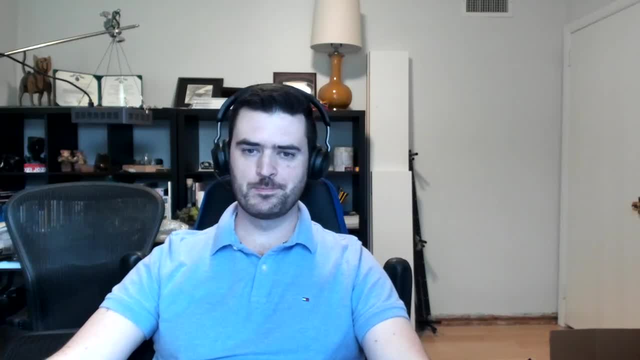 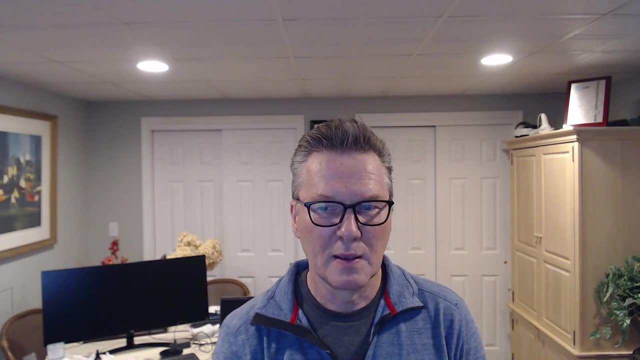 where you're actually using all four of those standards I talked about. So thanks for bringing that up. So give me a real world of fictional character you think would make an amazing or horrible. We can do a CISO, we can do a AI lead, we can do whatever you want. 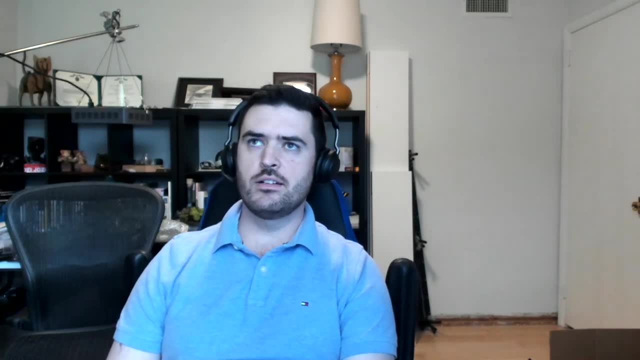 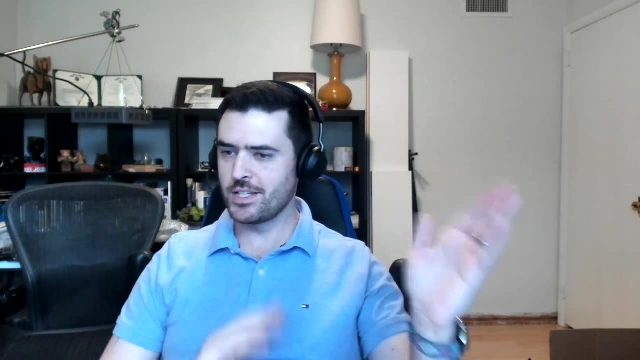 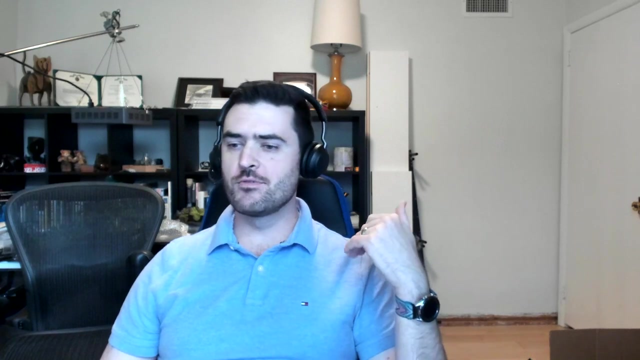 So I will do. I would say I'll go with a fictional character as a CISO, And this may be controversial, but I guess you could go both ways, And I just picked out the qualities that made it go this way. So I think Darth Vader would make a horrible CISO, and here's why. So he is ruthless, but he's. 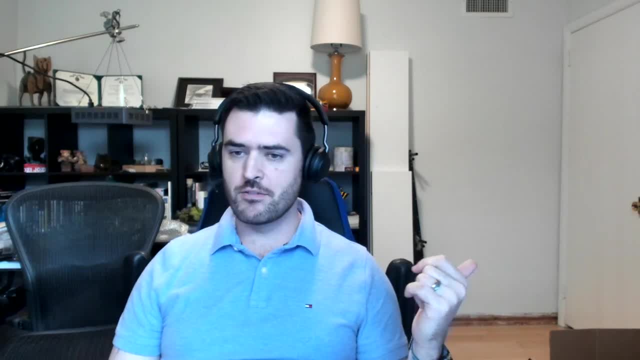